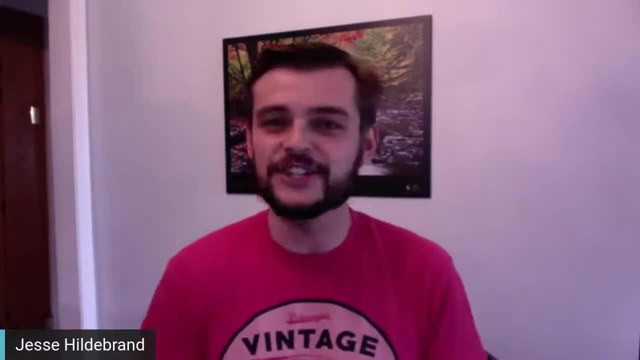 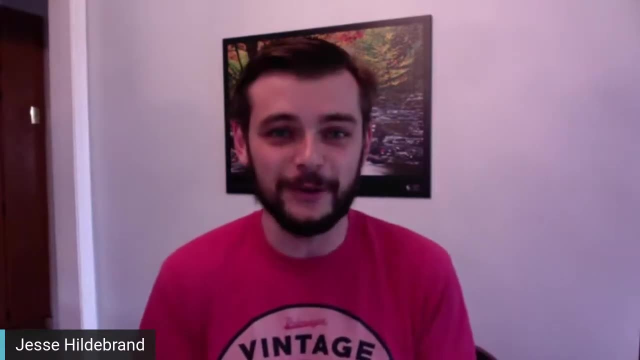 October is focused on space. We've got NASA engineers, we've got astronauts, we've got CSA personnel. It is a fantastic month highlighting our efforts to explore the cosmos around us. So huge welcome to our four classes. live right now. We should be getting a few more over the next. 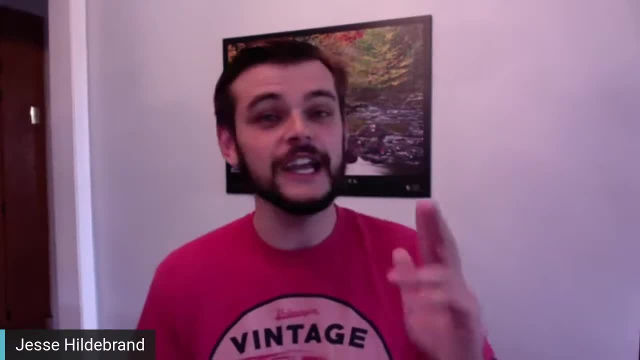 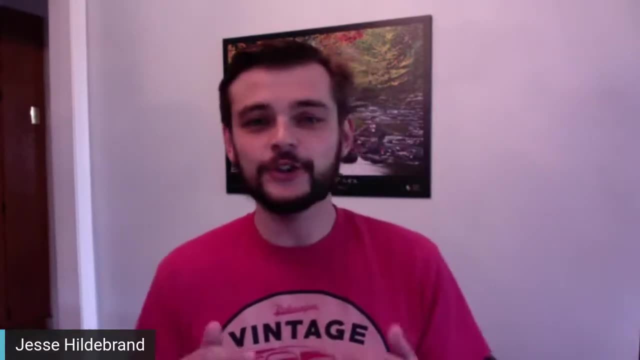 few minutes and all our students joining on YouTube and Facebook. If you're on YouTube or Facebook, let me know where you're joining from. I'd love to find out where you guys are coming in from and share your questions with Kevin. So today we are joined by one of my favorite people to have 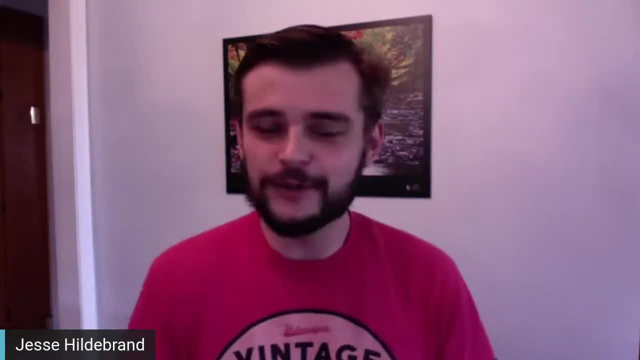 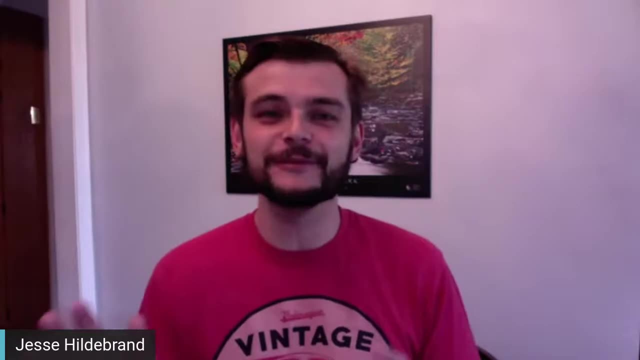 on the broadcast: Kevin DeBruin. So for all of you who wake up and you're like lazy, you don't feel like doing anything. today, Kevin is the antidote to all that, because he just cannot stop himself, because he's a NASA rocket scientist, He's a spacecraft systems engineer, He's gotten to work. 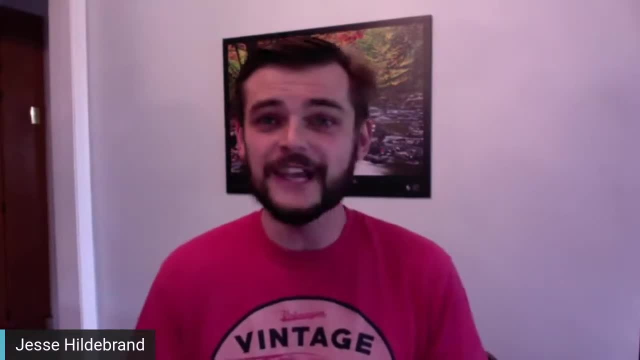 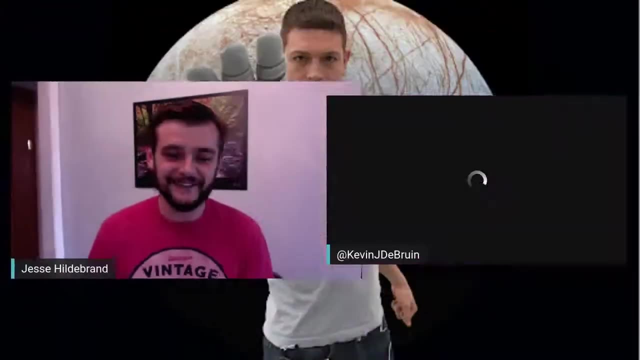 on some of the most elite and amazing robot space missions of all time. He's an Eagle Scout, American Ninja Warrior, personal fitness trainer. He does it all Without further ado. I'm going to bring in Kevin. Kevin, thank you so much for joining us again, man, And can't wait to hear. 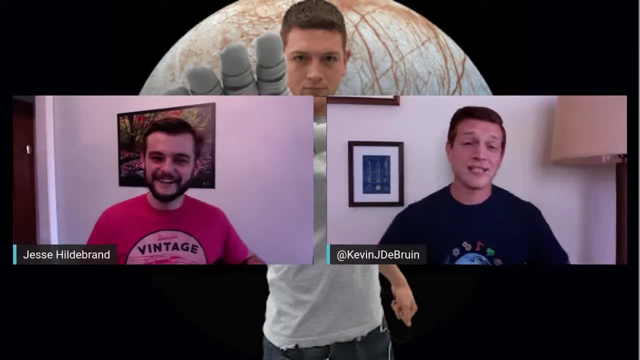 from you again today. This is great. Thanks, Jesse. That was an amazing intro there. I am extremely grateful for you doing that. That was amazing. My pleasure, man. Well, hey, you live it here, your story and share with all sorts of kids. today Got some great questions from kids around. 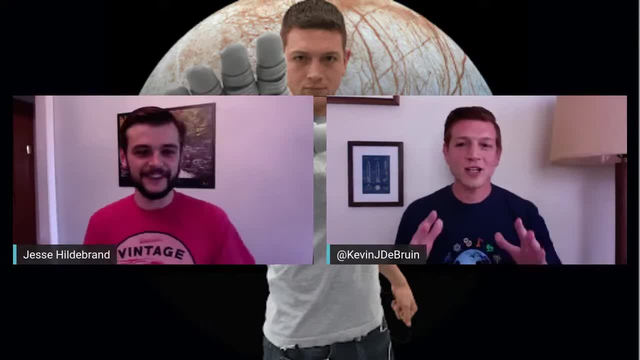 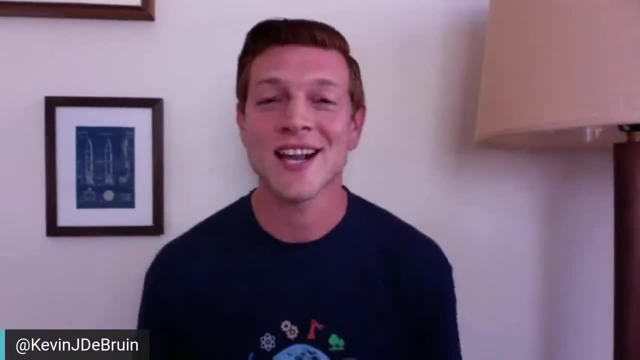 the globe. So let's dive in man. All right, Fantastic. So I got about like 20 minutes where I'm going to like teach you guys, talk to you about like what I did at NASA, one mission specifically- that's really exciting for me- And then we're going to open up to questions because 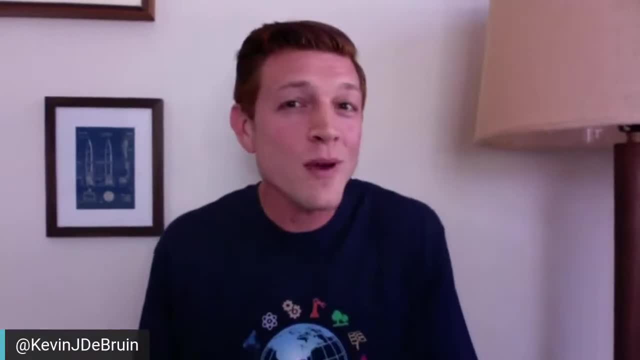 I want to answer all of your curious minds about what you might be thinking about space, or if you got questions about American Ninja Warrior or anything else that you hear as we're going through here. So I'm going to share my screen so that you can see. 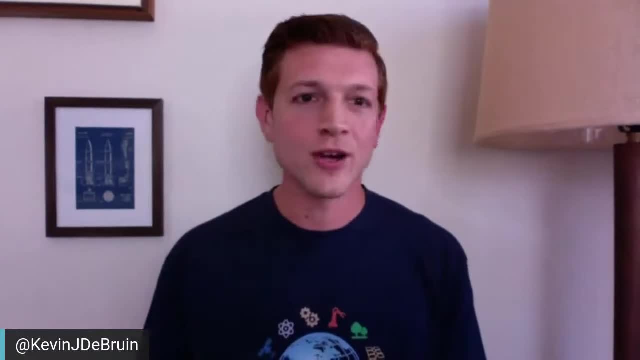 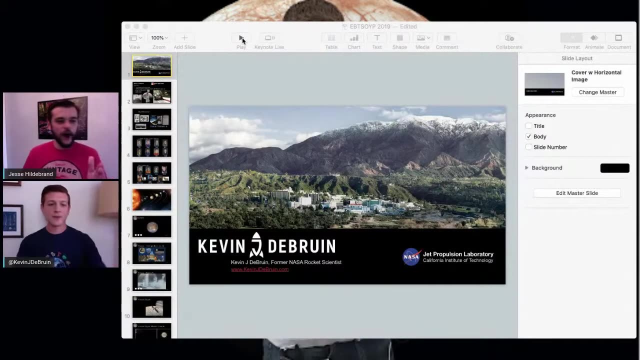 Some cool pictures and videos that I put together over here. So we'll go that. make it nice and big so we can all see it. Give me a thumbs up, Jesse, when I'm good to go Almost. So it didn't want to. 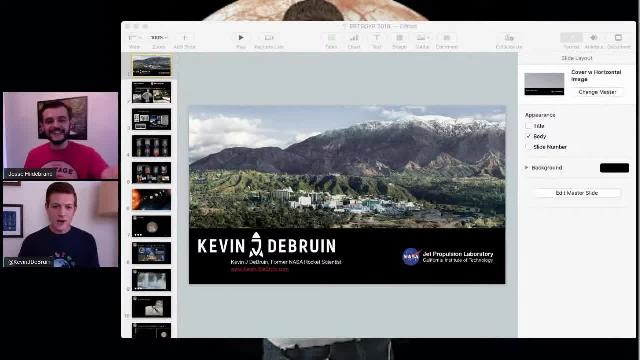 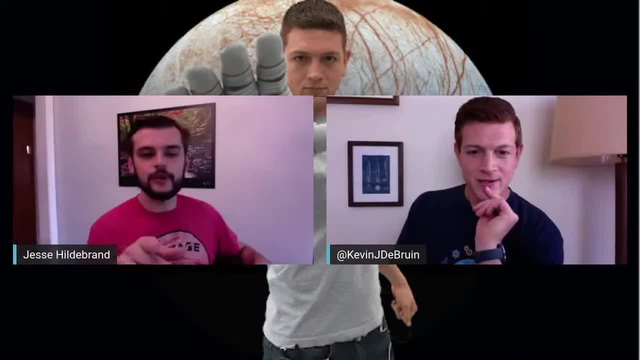 it didn't work. for some strange reason It worked earlier. We got your slide back on the left still, which is cool. It's kind of like a sneak peek, but there's a way to make that thing full screen. Let's check that out. Try full screen. If you did application window before, 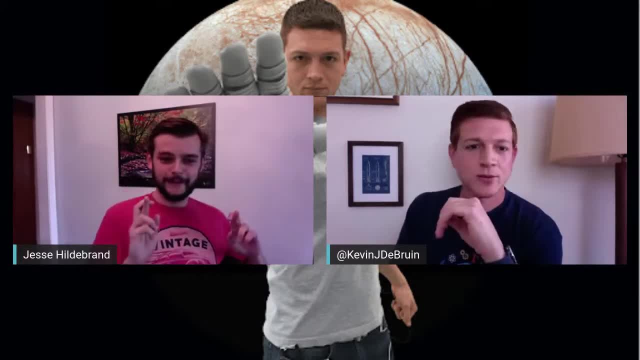 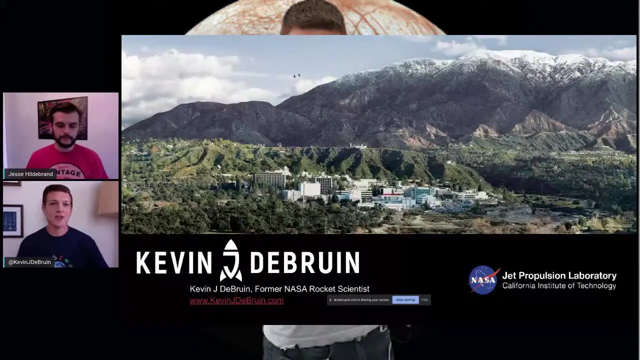 try full screen. Sometimes that works. Do the entire screen. We'll share that, which means you're seeing A couple different things. Very meta, There we go. Perfect, So you're good to go, man. Awesome, If you can see my cursor as well. it's in the sky. 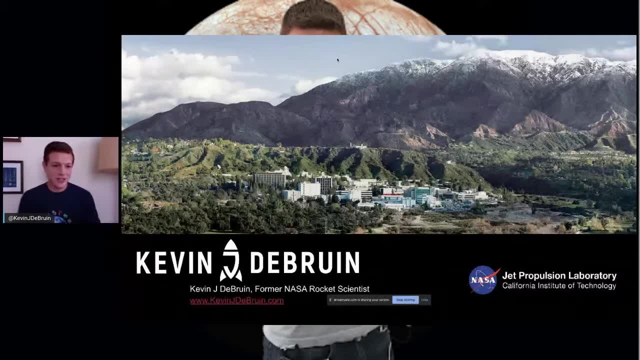 Yeah, we're perfect, Go for it. Okay. Well, what's up everybody? So, like Jesse said, Kevin Jader-Brun. So what we're looking at here is NASA's Jet Propulsion Laboratory. This is in Pasadena, California, just outside of Los. 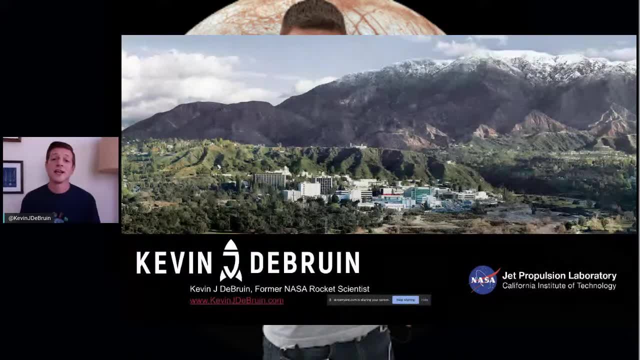 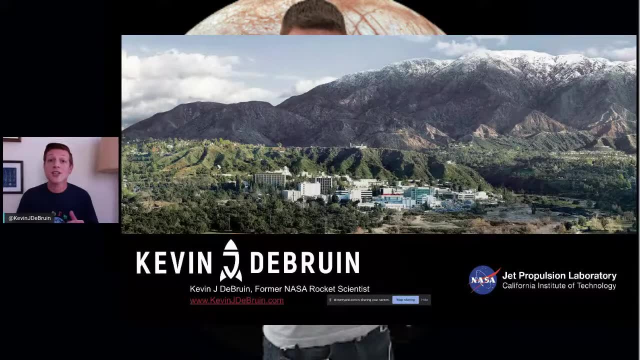 Angeles, where I used to work and where I'm still currently living, And I'd like to point this out because these are the buildings that the Mars rovers and almost all of the spacecrafts that are out beyond the moon are designed and built in before we send them off to the launch pad to go. 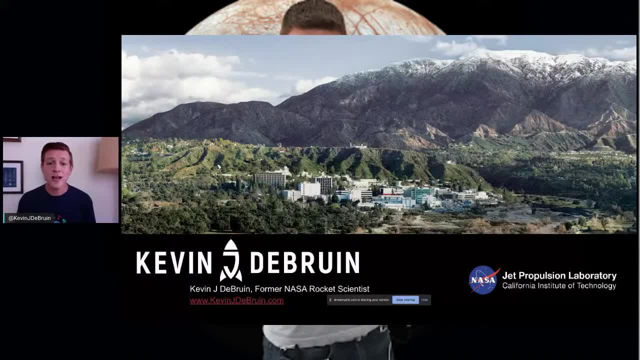 into outer space on the top of a rocket. And if you see this building right here that I'm moving around with my cursor, it's kind of like a teal green. That's where I used to work. That is that window right there. That's not my office. I was in the center. I wasn't one of the big fancy people. 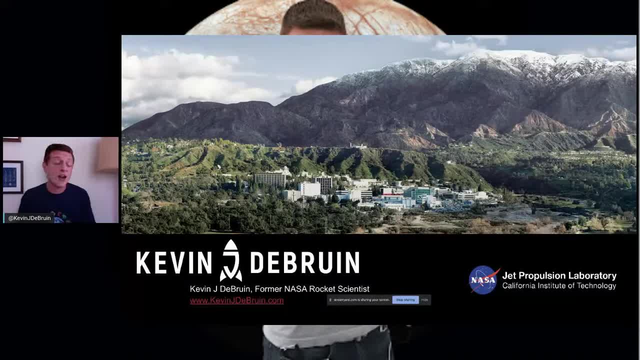 on the side, But that is where all of the rocket scientists and other types of scientists would come together and we would design these rovers, These spacecrafts, these satellites that you're seeing out on other planets and orbiting around other planets, flying to the outsides of our solar system. Now, first off, let's talk a little bit. 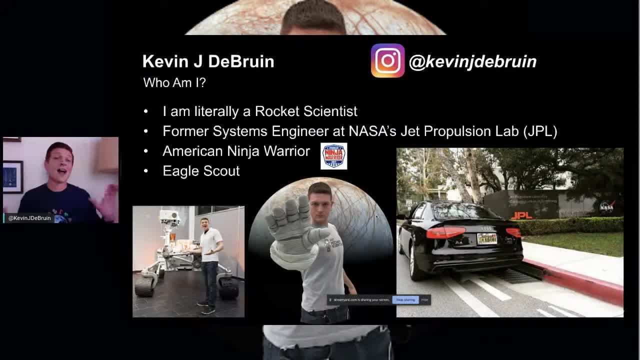 about who I am, All right. So I'm Kevin. I'm literally a rocket scientist And that is my favorite thing that I get to say: I know how to design spaceships. Now my official title, which you put on your job application and resume stuff, is systems engineer, And that was at NASA's Jet. 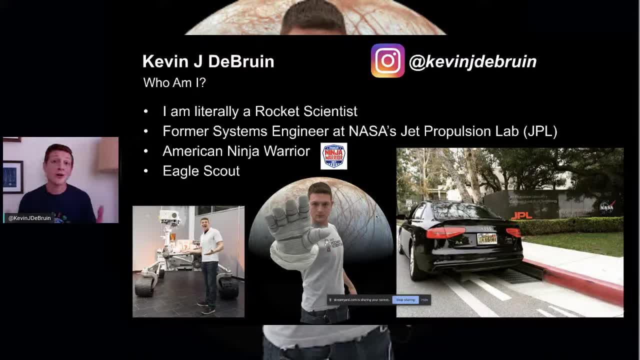 Propulsion Laboratory, And we just call that JPL. I'm also, as Jesse said, an American Ninja Warrior. I competed on season 9 and season 10.. And we're on season 12 right now. So for the last two seasons I'm not. 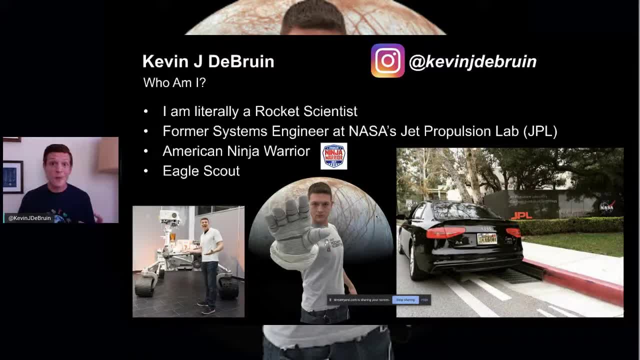 competing. I'm actually working with American Ninja Warrior the company to test the new obstacles that they have. So you know, when you're watching the show and then there's a new obstacle, Well, I've played on that to make sure it's not too easy for the ninjas, not too hard, Maybe things. 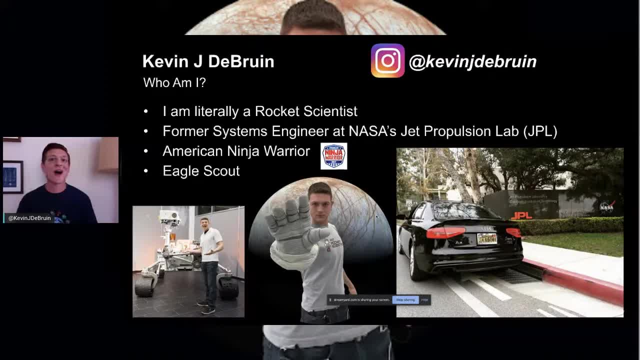 are a little higher or lower. Maybe we want to make it spin more, So I help them make that look all fun and fancy. And lastly, I'm an Eagle Scout. I like to talk about that because it talks about community service. you know, helping back, helping give back to the community, And it teaches you a 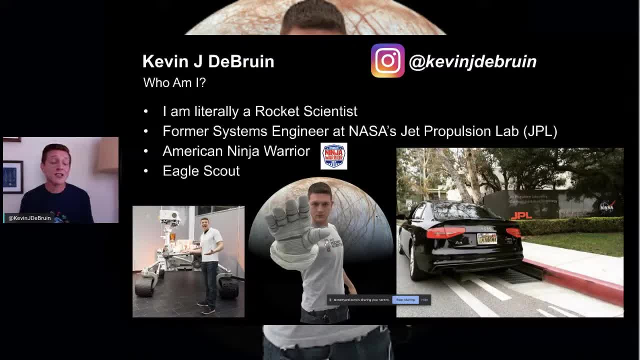 lot of really cool things. So if you're in the Scouts or not in a service organization, I suggest you join one. It really helps you out when you're going for college scholarships, college applications and then actually getting a job. I've got some of my jobs because I was an Eagle Scout. 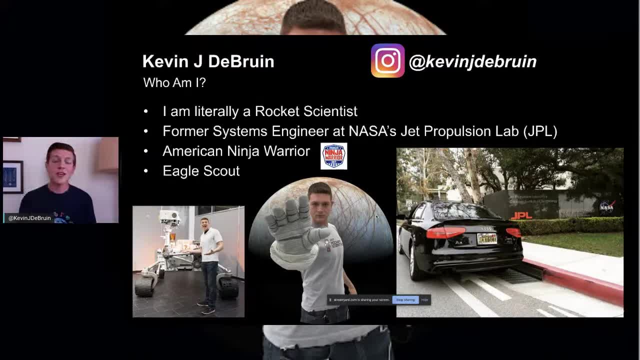 They looked down at the resume and were like: you're an Eagle Scout. We know we can trust you because you know how to communicate, you're a leader and you know how to operate with the team. So I just got some cool pictures of me down here. The one on the bottom: 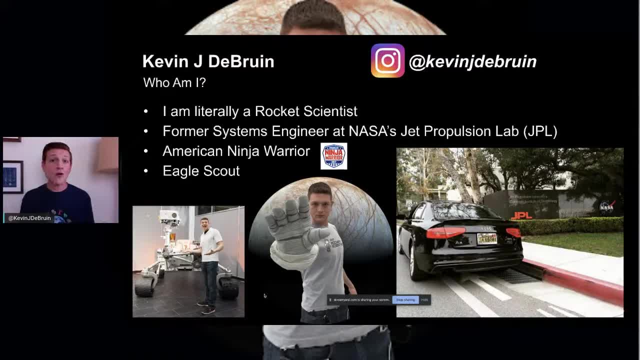 left side we see is with the Mars rover, the Curiosity rover. This isn't the actual one, but it's the same size. That's how big it is on the surface of Mars. Then you got me there with an astronaut glove pointing at you, kind of like Iron Man, with a special moon in the background. that 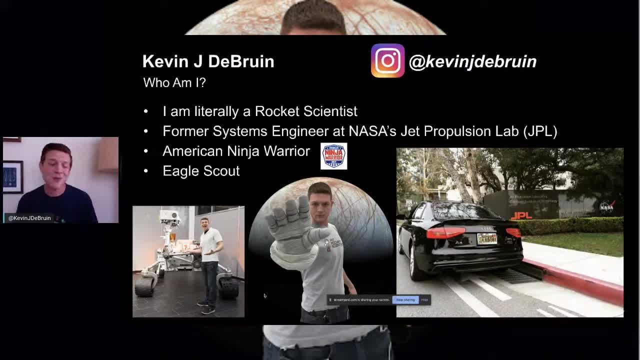 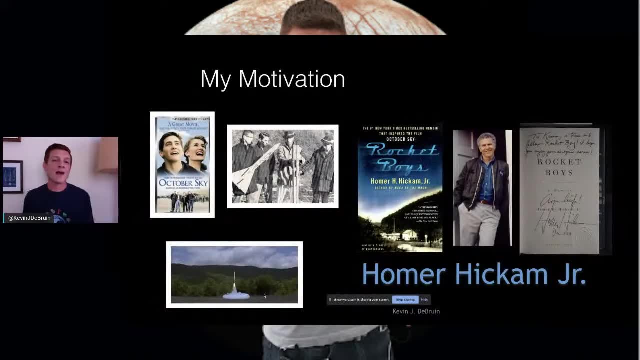 we're going to talk about today. And then, lastly, that's just my car, on the right-hand side, with the rocket. I just love everything about rocket science. Now, why I became a rocket scientist is because of this. I like to share my motivation. It's a movie. It's called October Sky. You see it. 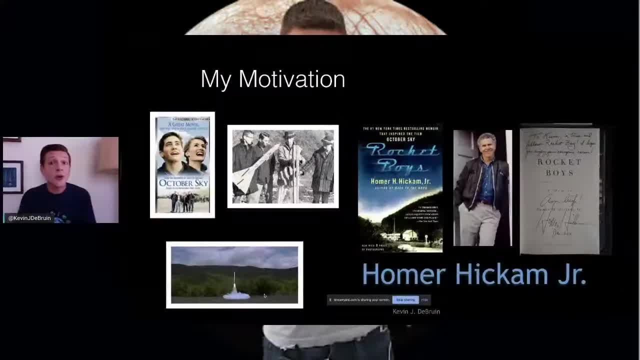 on the left-hand side And it's based upon this book. So it's a true story called Rocket Boys, And that guy you see on the right is Homer Hickam. He started off if you haven't seen the movie seeing the first satellite ever go across the night sky and got inspired starting building. 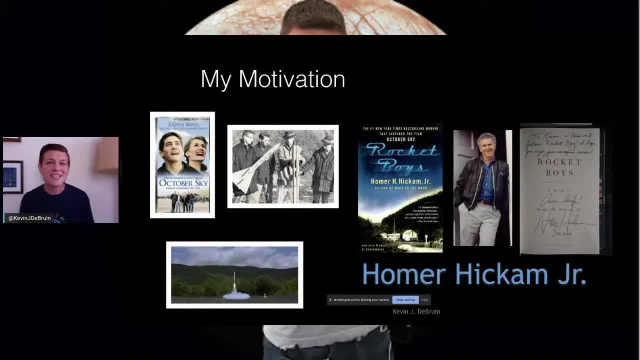 satellites, And then he goes on to become a NASA engineer training astronauts. Now I saw this when I was 10 years old. It was like, wow, I want to design spaceships for NASA. And I like to talk about this because it's hard work: going through school, having tests, doing homework, all of these. 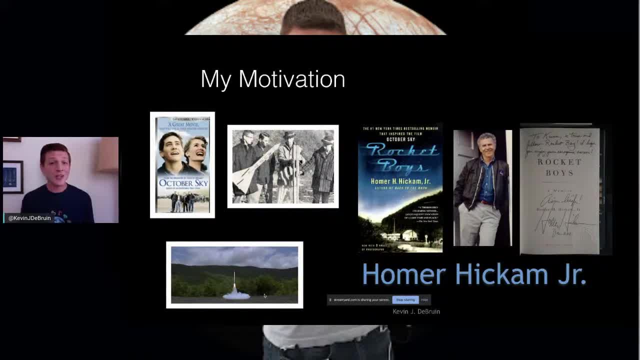 projects. I went up to the 19th grade And there was a lot of times where I got sad or it was difficult. I kind of wanted to give up. I would re-watch this movie or re-read this book to help re-ignite that fire. And I would re-watch this movie or re-read this book to help re-ignite that fire. 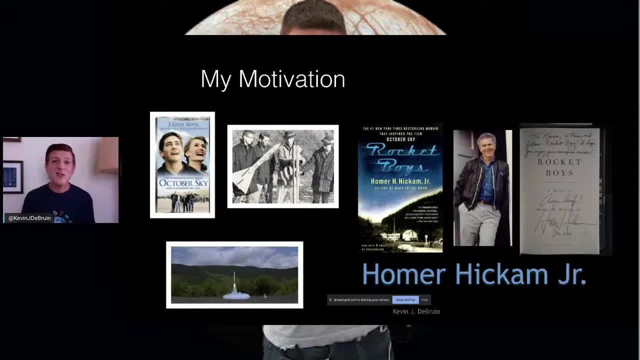 So it's something that can help you when you're kind of feeling down in the dumps or you're getting stressed out or maybe tired, Like why do I have to do this math homework? It was like: oh yeah, the math homework helps me design the spaceships. eventually, It's just part of the. 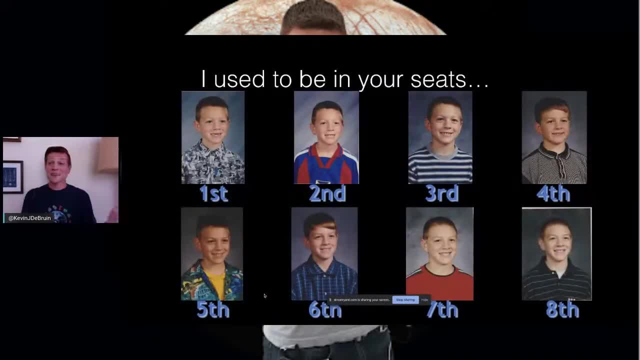 journey, So I like to share that with you. And there we go. This is what I used to look like as I was sitting in your seats. It wasn't that long ago where I saw October Sky and was figuring out exactly what I wanted to do with my life, And that was working for NASA designing spaceships. 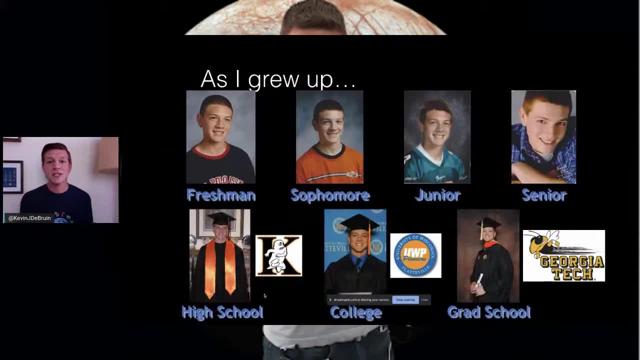 You know, and then as I grew up, going into high school, here's my education. Like, I got a high school degree, Then I got a bachelor's in mechanical engineering from University of Wisconsin-Platteville, And then I went on to Georgia Tech and I have a master's in aerospace engineering And that's. 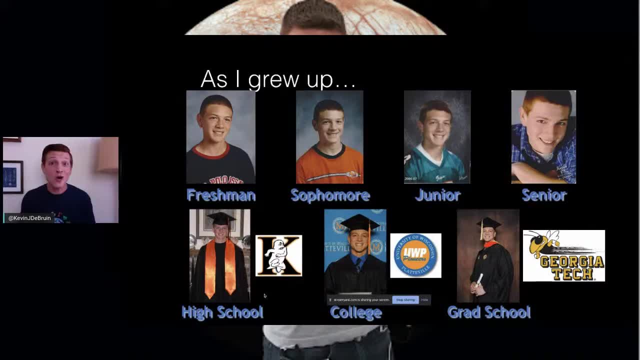 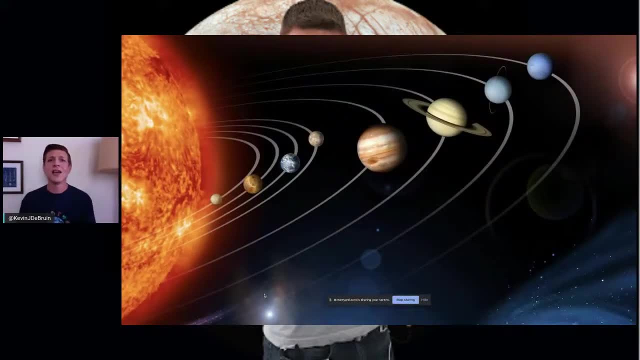 where I went to the 19th grade. So it's a long journey, but it's worth it, because then you can design spaceships. So, speaking of spaceships, that's the important part, right? That's what we want to get to here. We want to talk about space. So we got here. we got eight planets. 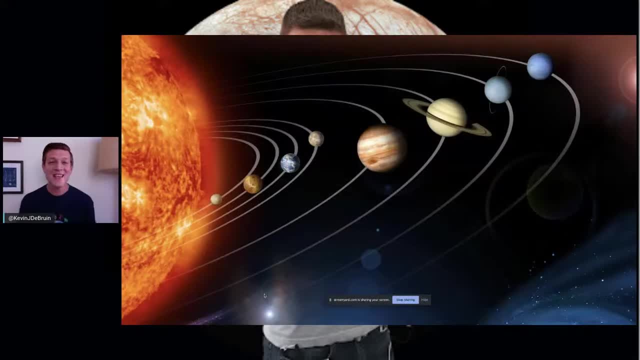 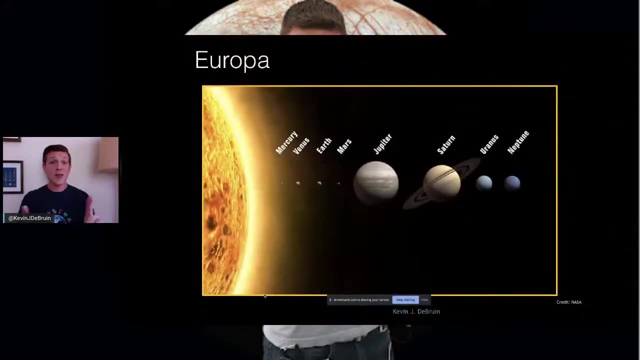 not nine. Pluto was demoted. We can talk about that later if you want, But let's bring this up because this is what I want to talk about, that cool moon we saw earlier. Here's our planets. So that moon was called Europa, And if you haven't heard of Europa before, I'm very excited to tell. 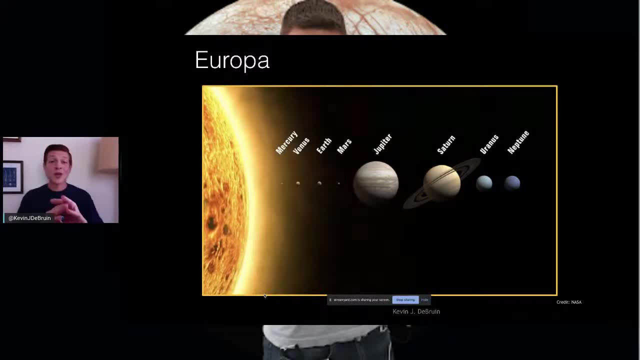 you all about it, And if you have heard about it, you're going to learn even more. So we got our eight planets here Now. some of them have moons, some don't. Mercury and Venus do not have moons, but everyone else in the solar system does. Saturn has the most. 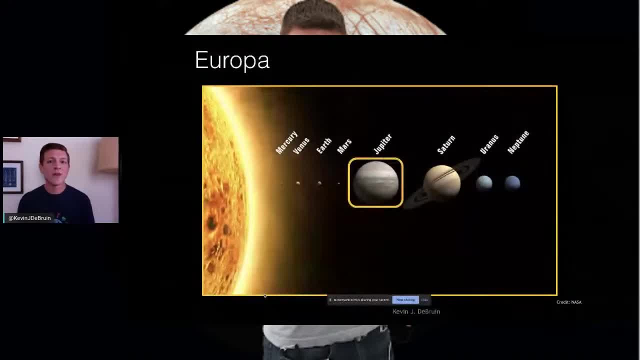 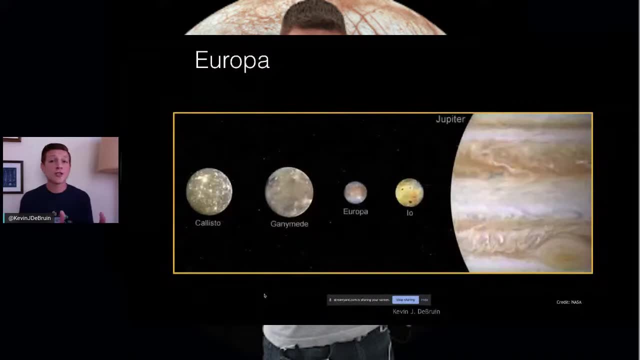 but Jupiter has a whole lot too. So let's bring up Jupiter. The four biggest moons are called the Galilean moons and they're right here. So going from closest to furthest away, we got Io. It is the most volcanically active body in the solar system. What that means is there's volcanoes. 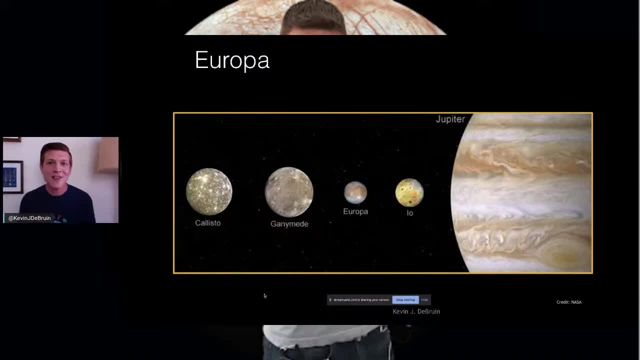 erupting all the time. So you see some of those little dots on the moon. Those are volcanoes. Next up is Europa. We're going to dive into that one in a second, So we're going to jump on a Ganymede. This is the largest moon in the solar system. It is bigger than the planet Mercury. 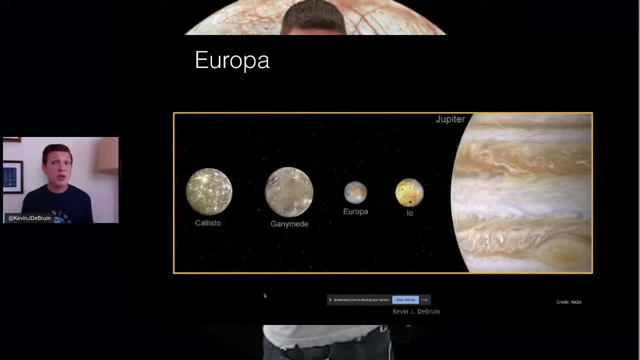 Yeah, bigger than Mercury. So if it wasn't around Jupiter, it probably could have been its own planet. And then Callisto, that last one there, that is one of the oldest, if not the oldest, body in our solar system, Kevin, how do you know that? Well, take a look. You see all those bright dots. 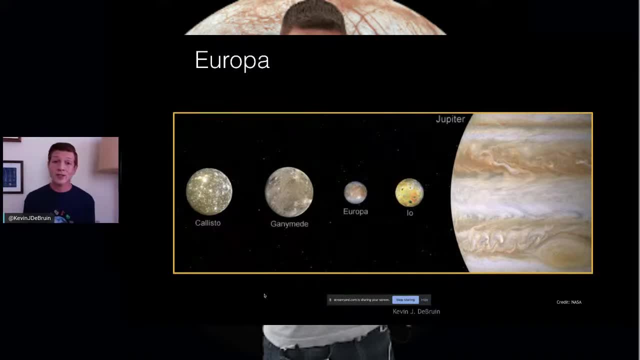 Those are actually craters. So the longer something has been in our solar system, the more chance it has of things hitting it. So an impact crater creates those little holes all around. So if you look at a body- a body being like a moon, a comet, an asteroid, a planet, a star- and it has a ton of craters on it. 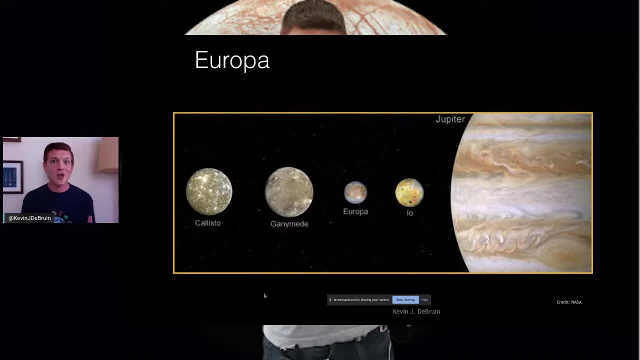 we call it crater dating, and it's got so many craters on it we know that it's been so old. Now they are actually a lot further apart than they are here in this image. This is just to show them really close. So we found these over 400 years ago. A guy named Galileo. 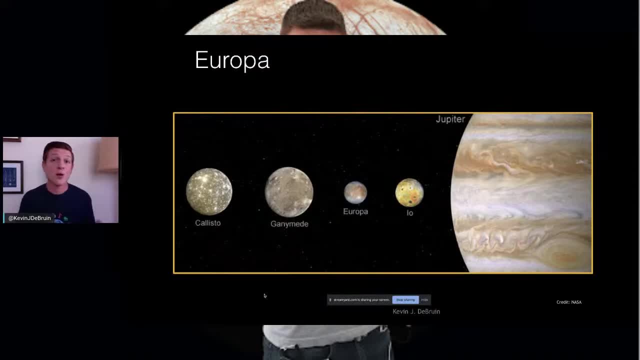 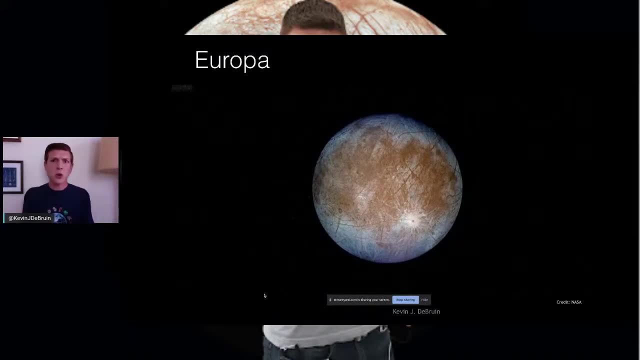 you might have heard of him, Looked through his telescope and found these four moons. Now Europa. that's the cool one, That's the one that I worked on and it looks cool, literally like it's blue. Blue's cool color. 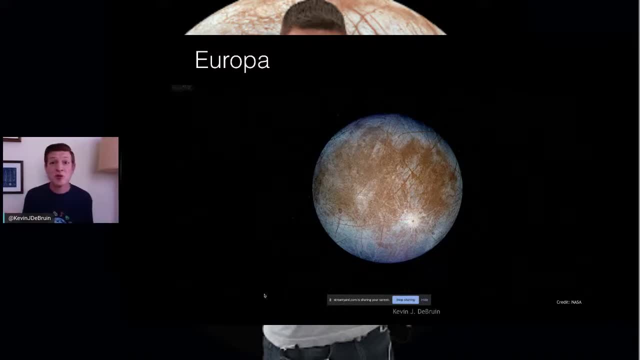 We got these red splotches and some red lines. Maybe those are cracks, Maybe an alien was just taking a shovel and, you know, made those cracks. We don't know What we kind of do. So Europa is the best place in our solar system to find aliens. Yes, 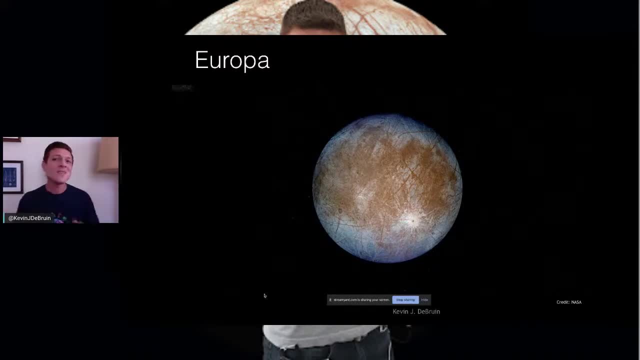 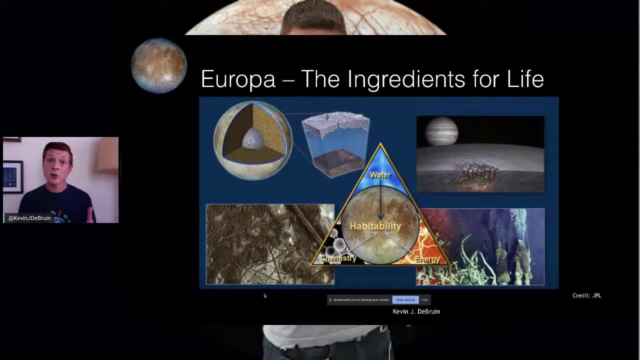 If there's aliens in our solar system, we believe that Europa is the best place to search for them. Now why, Well, Europa has the ingredients for life that we know about, because there's life like we know, like us, we're carbon-based life forms and stuff. and then there's life that we don't know. 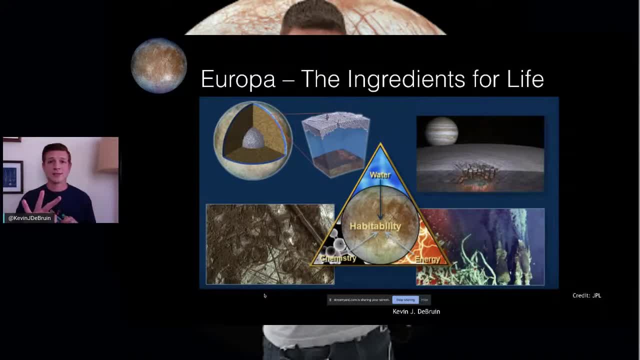 about. But this is what we do. know That you need three things to find life, Like when we find life here on Earth. it has these three things. The first one: there is water. Where you find water here on Earth, you find life, You go out. well, I'm close to the ocean so I can take a spoon. 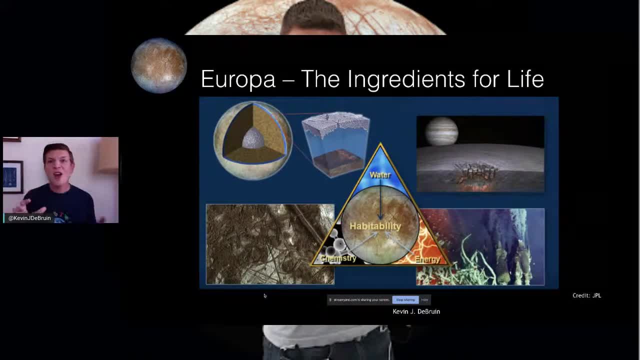 go a couple miles down the road, take a spoonful of ocean water and there are millions of microorganisms just inside that one spoonful of water. So Europa is essentially a big ball of water that's frozen on the outside. It's got this huge liquid ocean underneath it and then it's got 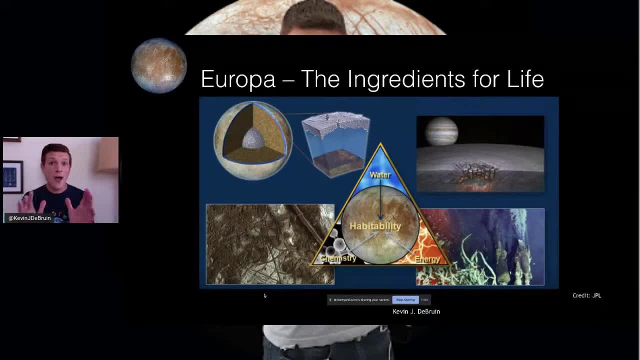 an icy crust on the top So we can check that box. Europa has water. Now what else do you need? You need chemistry, So that's in that bottom left-hand corner. there You need the building blocks of life. You know the things that we find in rocks. Specifically, you may have heard these: 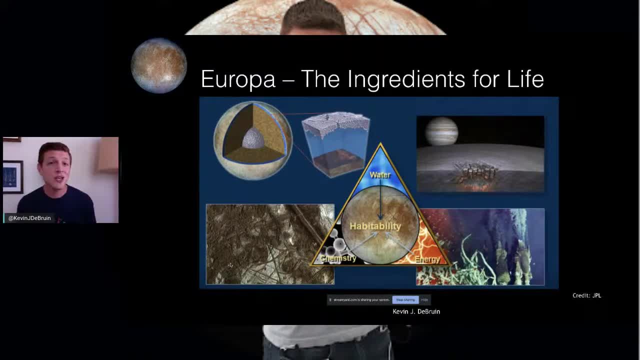 words before, and if not, they're cool science words. You need carbon, hydrogen, nitrogen, oxygen, phosphorus and sulfur. C-H-N-O-P-S is the abbreviation. I say schnapps and that's how I remember it, So you need those elements. Those are scientific elements on the periodic table in the. 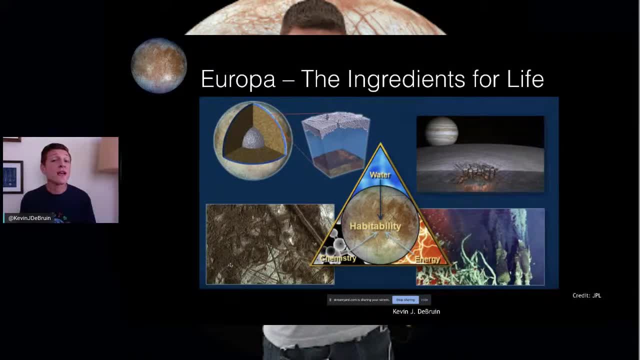 right combinations to build up life And we think that Europa has all of them out there. We've actually detected some of them already from previous missions and from using the Hubble Space Telescope. That's a giant telescope that's out orbiting Earth looking out at distant planets. 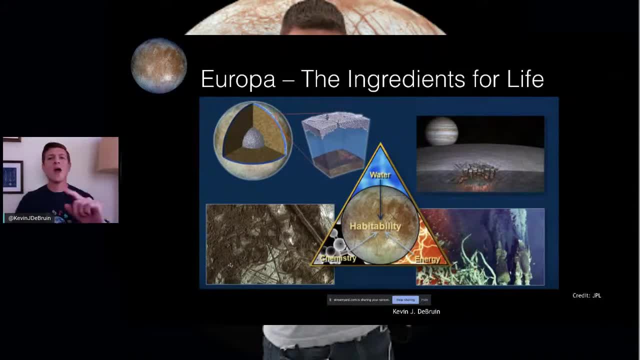 and stars and other galaxies. Okay, so now energy. We need a way to power life, right? So here on Earth, what do we have? What's that huge thing in the sky During the daytime that gives us all our heat and light? The sun? Well, Jupiter, which is where. 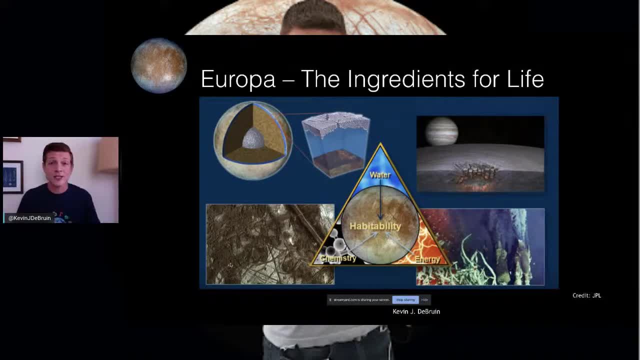 Europa is is five times further away than Earth is from the sun. So the sun is just not strong enough to power life like how we do here on Earth, how it does here on Earth. So we need something else to happen. Well, we saw those four moons before right That go around Jupiter, called the 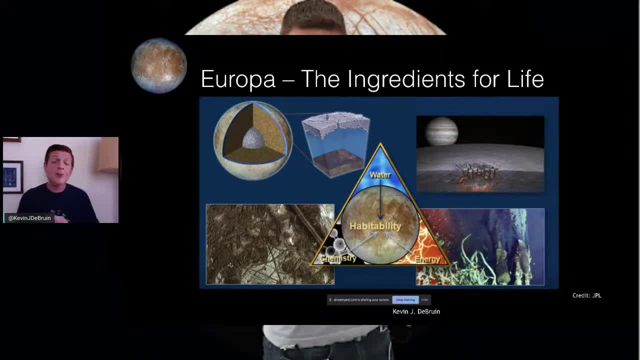 Galilean moons. Well, they actually. they play with each other the whole time. They push on each other and pull on each other. So make a fist and hold it really tight. So this is Europa when it's not being played with, And then open it. 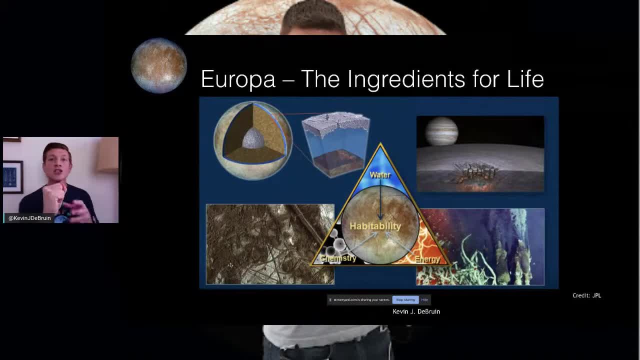 up a little bit and then squeeze it. Open it up a little bit and squeeze it. So that's what's going on at Europa: It expands a little bit and stretches and then compresses. That's because the other moons are pushing and pulling on it with their gravity. Now, how does that give us energy? Well, 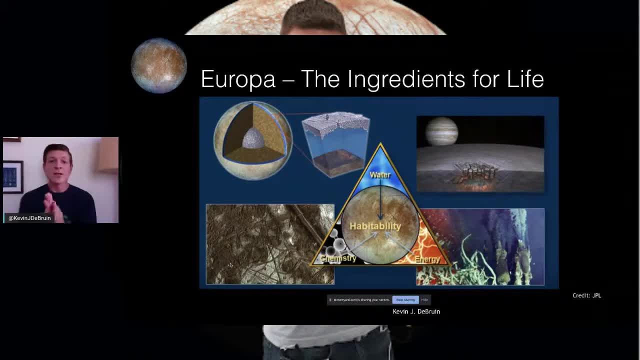 put your hands together, All right, And I'll rub them real fast. What do you feel? You feel heat, right? Well, there's friction. So that movement, moving your hands together, creates friction, creating heat. And that is what the energy. 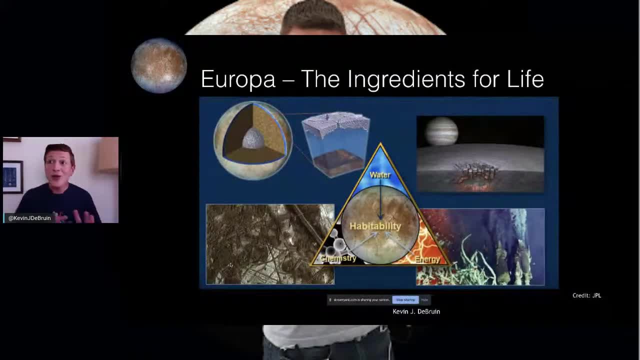 source is out at Europa to maintain that liquid right. If we have liquid water way out in space, how does it stay liquid without some sort of energy, some sort of warmth? That's it. It's Europa getting bigger and smaller, And what's really interesting is that image in the bottom. 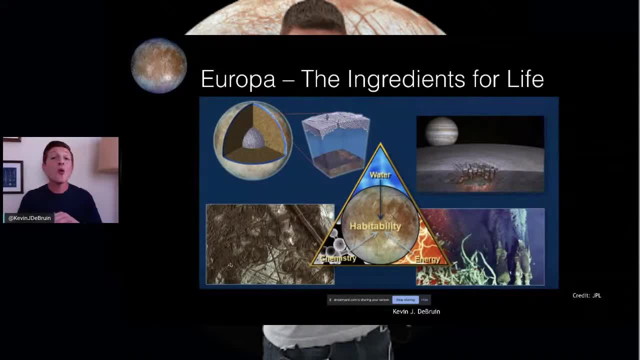 right. So that's from the surface, the ocean floor at Earth, And those are hydrothermal vents or things like under the surface, And that's what's going on at Europa And that's what's happening. We have underwater volcanoes that are releasing salts and minerals and energy. 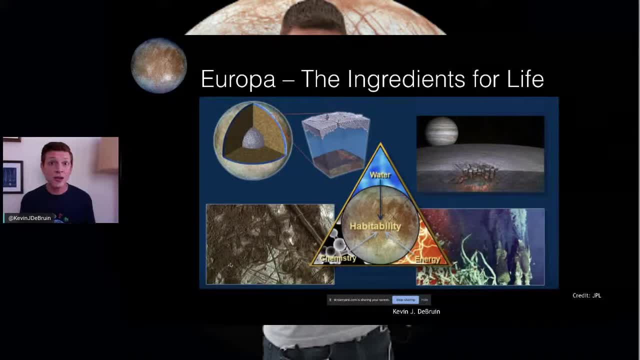 into the ocean And we have those here on Earth, Yeah, And we find life around those what we call also like black smokers. You see, like the black smoke that's coming out of it, We got hairy snails. We have fish. you can see through down there. It's crazy. It's completely black. No sunlight can get. 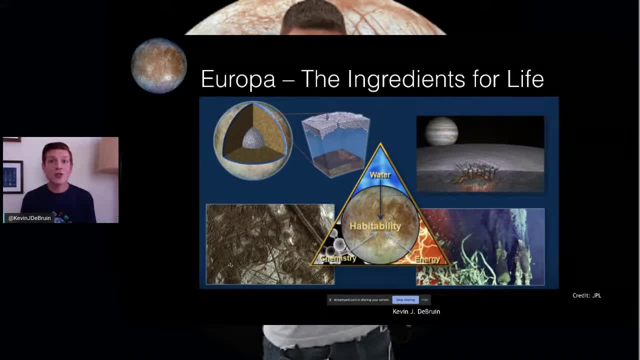 there. But all of the energy coming out of these vents powers the life down there, And so energy from the sun is called photosynthesis. That's how our plants get their metabolism, their energy, their life source down there. It's chemical energy called chemosynthesis. So we believe the 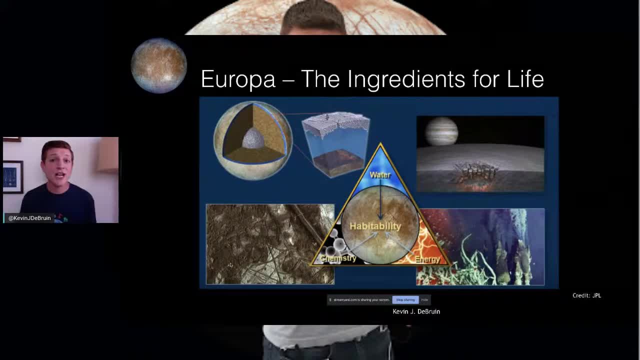 combination of water, the carbon, hydrogen, nitrogen, oxygen, phosphorus and sulfur, And this chemosynthesis is going on at Europa And that is the best place in our solar system to find aliens. Now I know what you're thinking: Are there going to be, like alien sharks and alien? 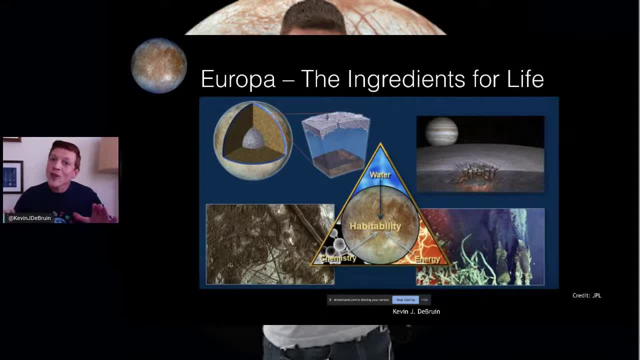 whales and maybe alien octopus out there. I would love to find that, But I don't think we will. What we're looking for are tiny little microorganisms, so small you can't see them with your eye. You'll need a microscope to look at them. So we're going to see if we can find them. 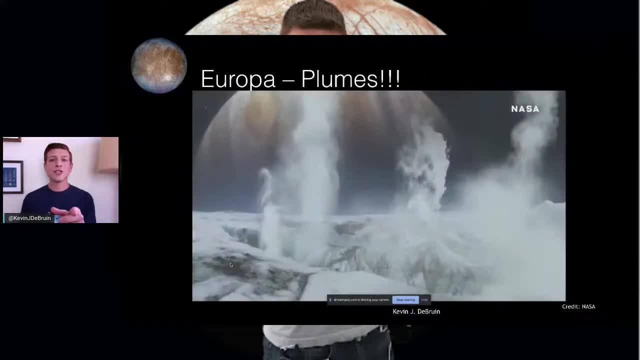 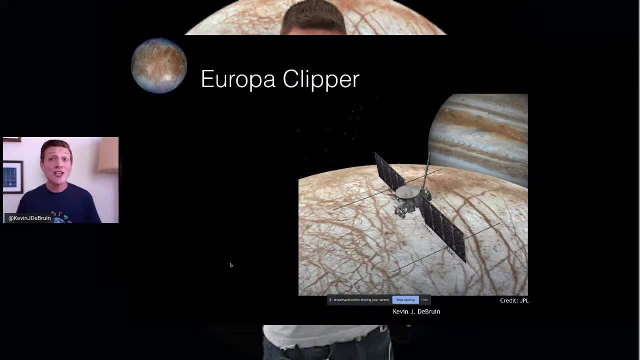 And how are we going to do that? Well, we jump past that really quick. I want to show you this first. So this is Europa Clipper. This is the spacecraft that we're currently building to send to investigate and see if we can find these potential signs of life. What we're really. 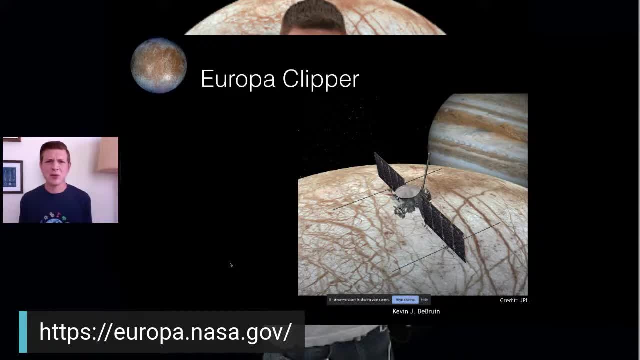 testing for is how habitable. habitable, it's a big word. Well, habitat is like something you can live in. Habitable is: is that place livable? So we're going to test and see if everything we think about Europa being livable is accurate. We're going to do that with Europa Clipper. 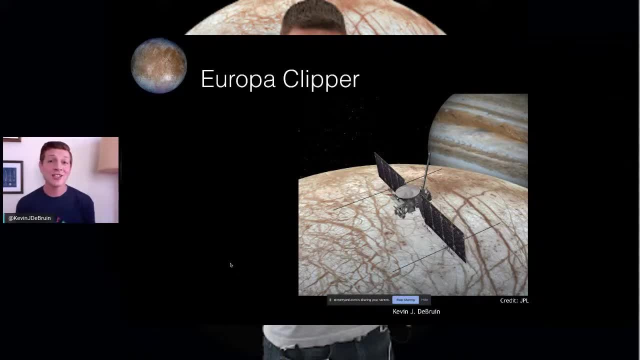 Now, I started working on this spacecraft when I was in college And then, once I got hired at NASA, I kept working on this spacecraft and another one that I'll tell you about after this. So what does it look like there? It's kind of funky looking. 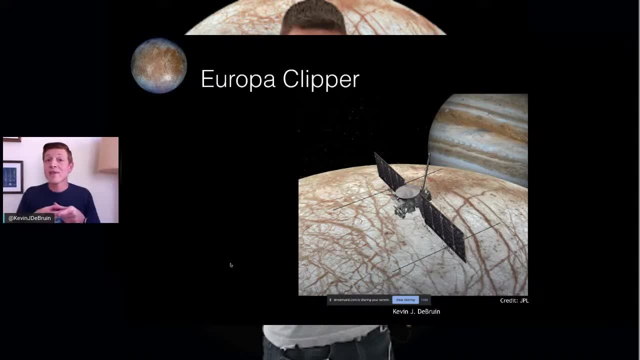 Well, the big circle in the middle, that's our antenna. Essentially it's like a cell phone that we call home with. So we point that at Earth and we send all of our information back like: hey, we found carbon. Hey, we found CO2.. Hey, we found H2O, We found all these things. 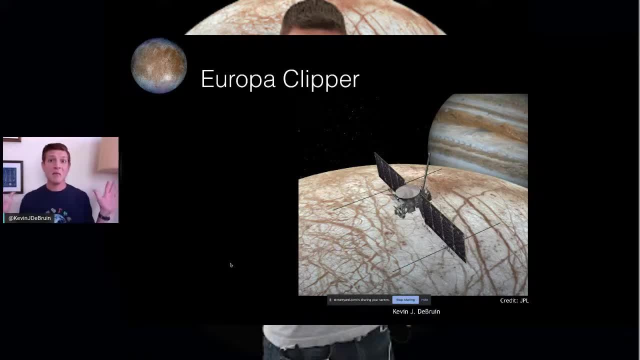 Or if things go wrong with the spacecraft. that's how it can tell us: hey, something's going wrong And we can be like: hold on, Okay, do this to fix yourself. And the big little panel things you see on the side like the wings, those are solar panels, So the sun can't power life. 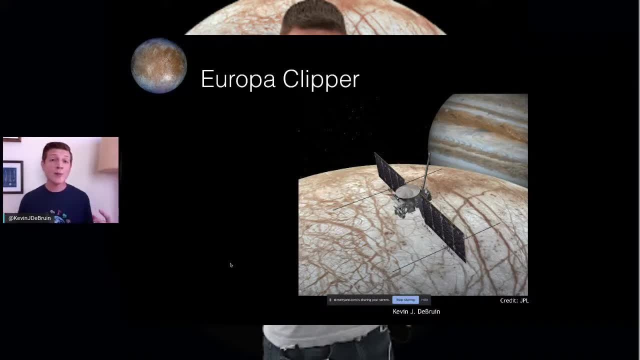 but gigantic solar panels can absorb some of the sun's energy to power our spacecraft out there. And then the rest of the things you see on. there are other types of science, instruments like microscopes and radars and other things for us to test as we're going around Europa. 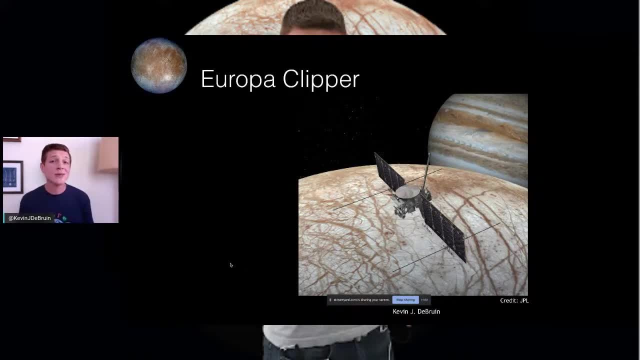 So we're going to launch in approximately 2023. So about three years from now. we started to build this thing already. It's being built in a couple of different places around the country. Then they're all going to come together to create our spacecraft. We'll launch it in three years. 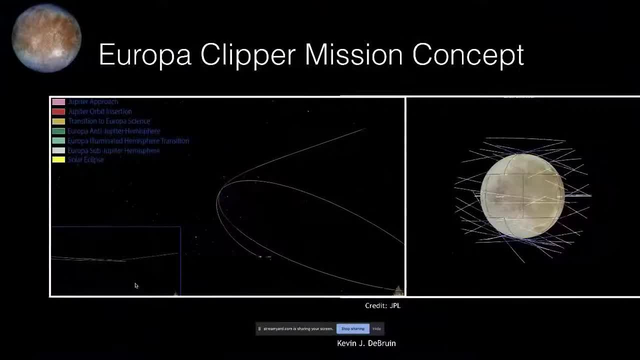 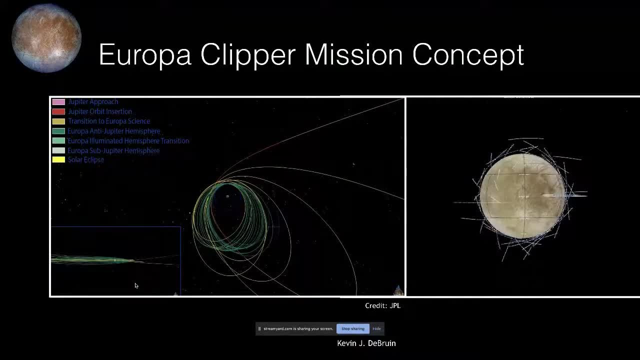 Then it looks like this: So on the left-hand side is tracing the path of the spacecraft once it gets to Jupiter. Now, it's going to take a long time to get to Jupiter- about two and a half years- And then, once we're here, we're going to be at Jupiter. So we're going to be at Jupiter. 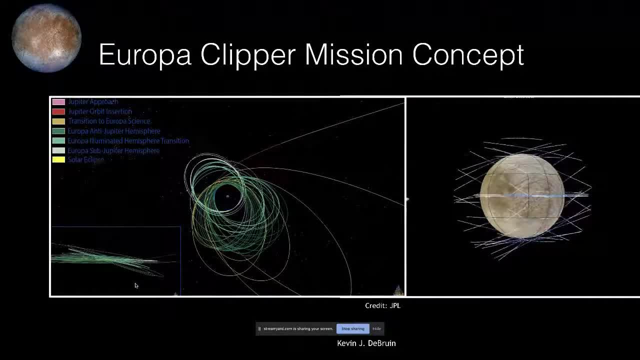 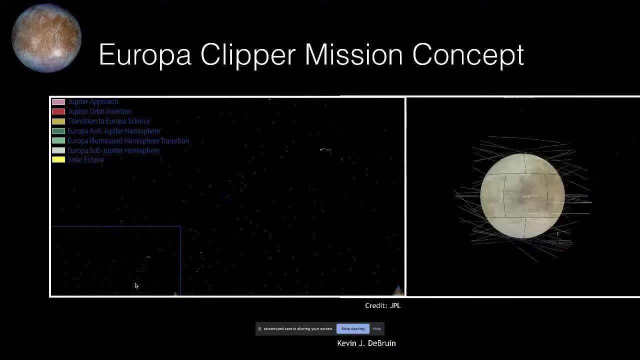 For two and a half years And we're actually orbiting Jupiter and just flying by Europa because the radiation environment at Jupiter is crazy. Let me play that again for you while we're talking. So we're seeing our spacecraft go on the left-hand side It's. 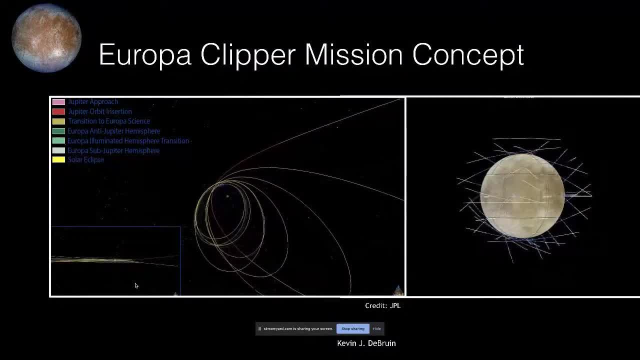 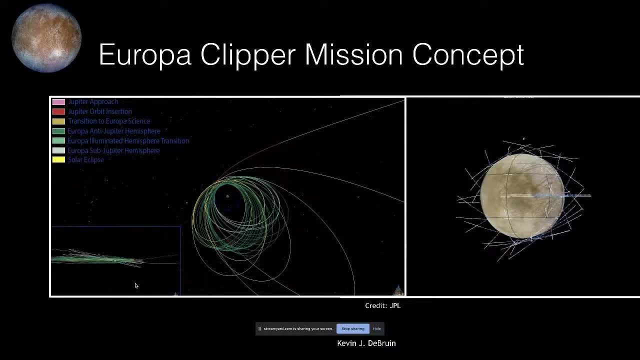 doing long looping orbits around Jupiter and then closely flying by Europa to hustle in and collect our science. On the right-hand side you see all the different places, those white lines where we're flying over Europa to essentially be like we're orbiting it. 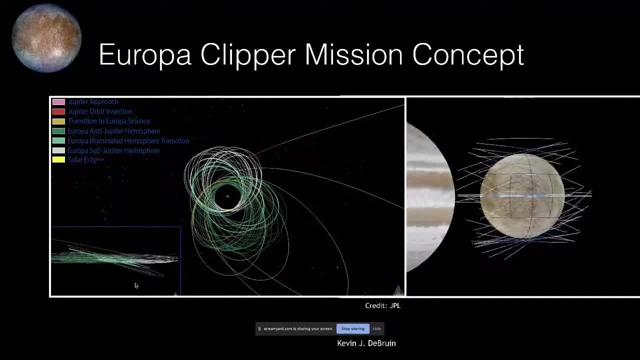 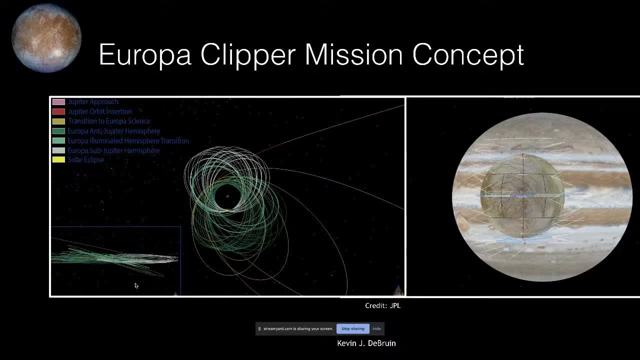 But, like I said, we're not orbiting it, We're flying by it because of the radiation environment at Jupiter. Jupiter is so big, it pulls in a lot of the radiation with gravity- and electronics don't like gravity- Like if you've accidentally ever put metal in the microwave and it goes crazy. 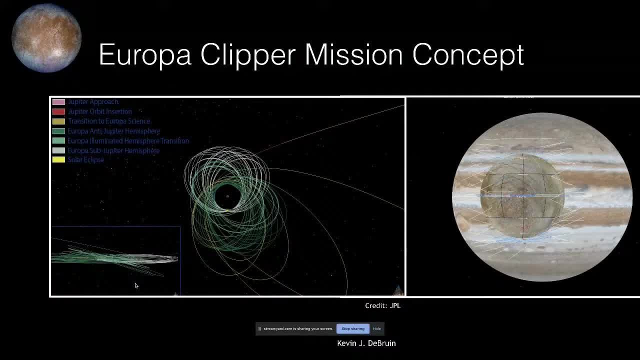 don't do that. Jupiter is like a huge microwave out there, and we don't want our spacecraft, which is metal with electronics, to be in there very long. Now, what does each one of those look like? Well, as we're going into Europa, we're going to be in the middle of Europa, So we're 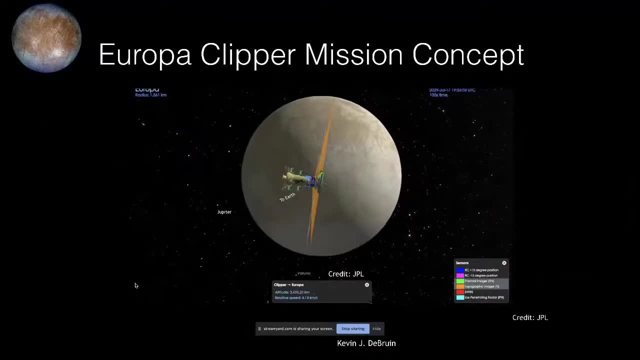 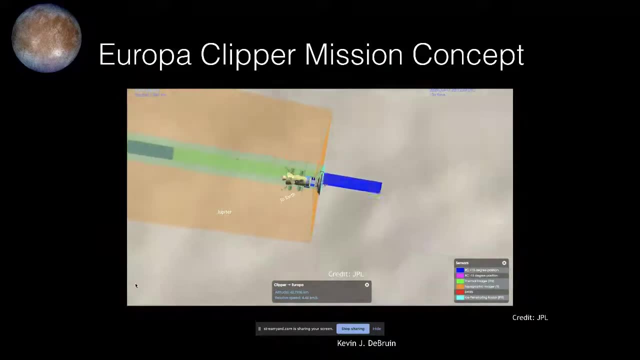 going to be in Europa. Each of those things is called a flyby And it looks like this: We're coming in. these different colored bars turning on are just different science instruments. So as you get closer, this blue and pink is us taking photos back and forth, back and forth, to give us. 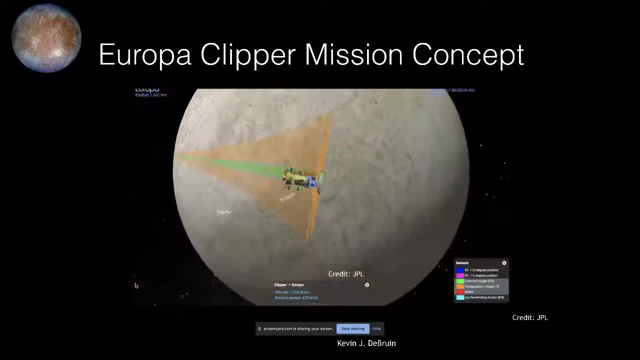 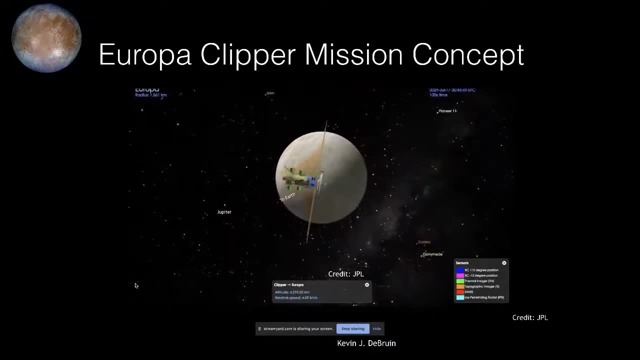 a stereo image, So like a two-direction image of what we're looking at the surface, And then we keep on flying by, And then, when we get so far away that our instruments, our science devices, don't really work anymore, we turn them off, And then we take all of that. 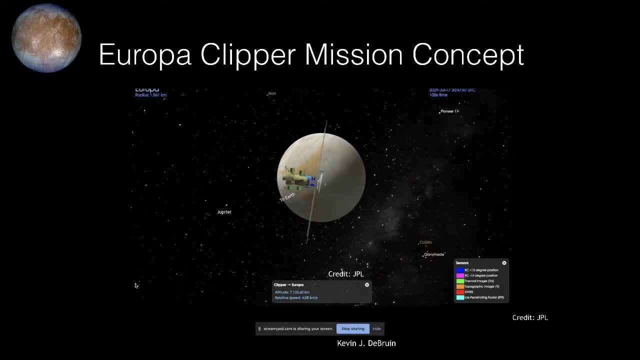 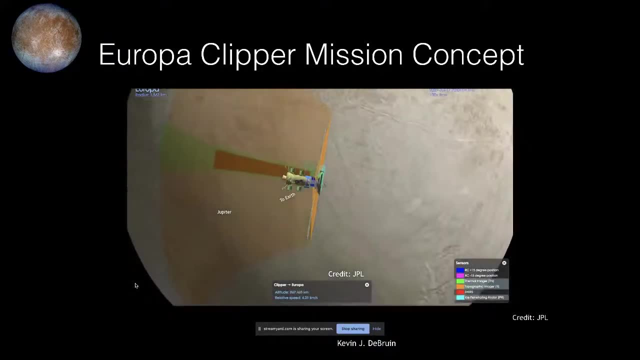 all of that data, all of that information that we've collected and send it back to Earth with that giant antenna. Let's look at that again. So we're like 66,000 kilometers away. We've got our radars on, We're coming in trying to see how thick is that ice, How deep is the ocean. Let's take 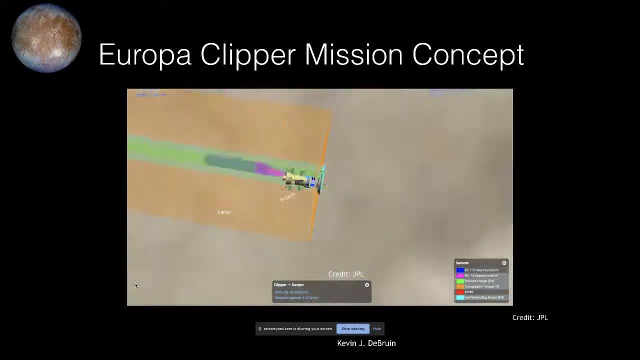 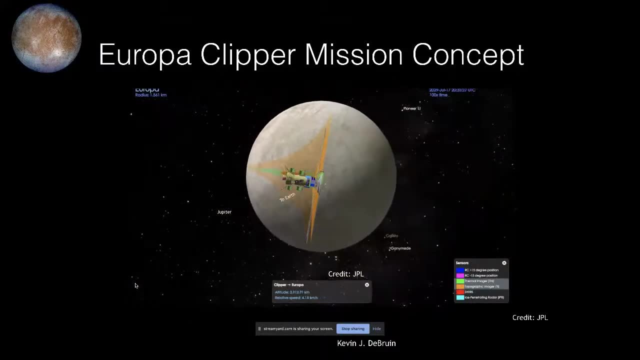 some high-resolution pictures to see what the surface is like if we want to land there in the future. And let's keep on studying it until we get again about 66,000 kilometers away, trying to detect the gravity field around Europa. what it's like? what's the radiation? 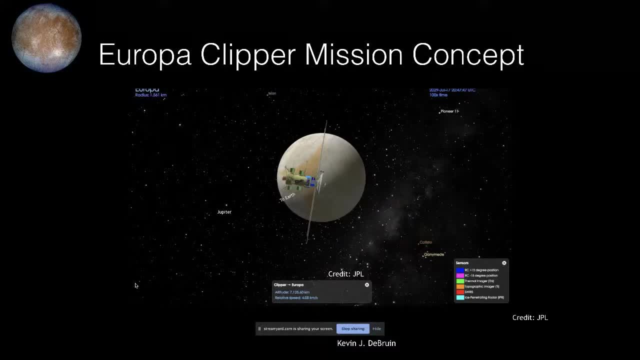 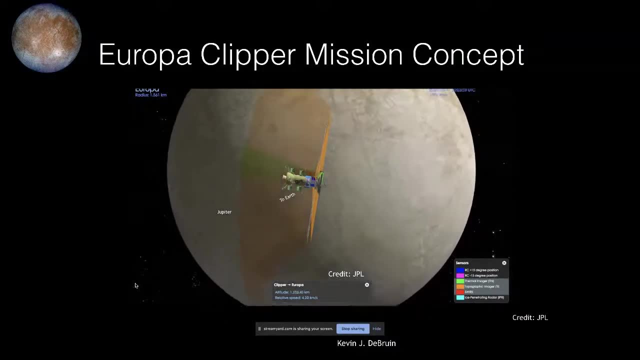 like and then send all of that information back to Earth. Now it's going to take 14 days before we come back and fly by again. We're going to be sending information to Earth and then recharging our solar panels. So it takes, we're coming in, we come within 10 kilometers here flying super. 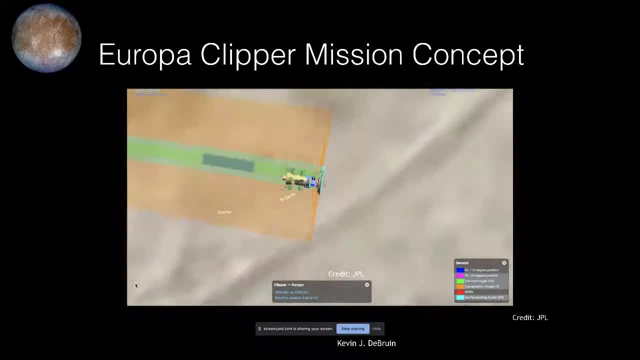 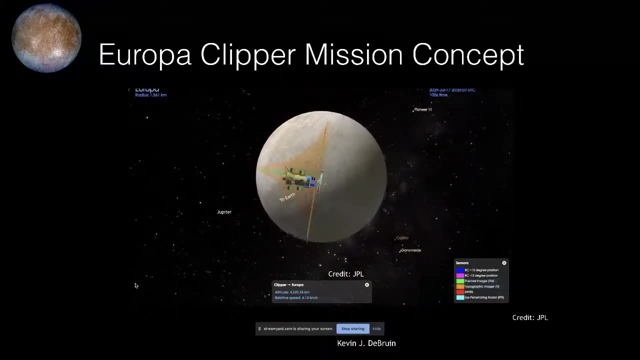 super fast, a couple kilometers a second, as we're flying through, And then we have to get out of there because we're in the hard radiation zone And then kind of like cool off, recharge ourselves, And then in two weeks we're going to come back. 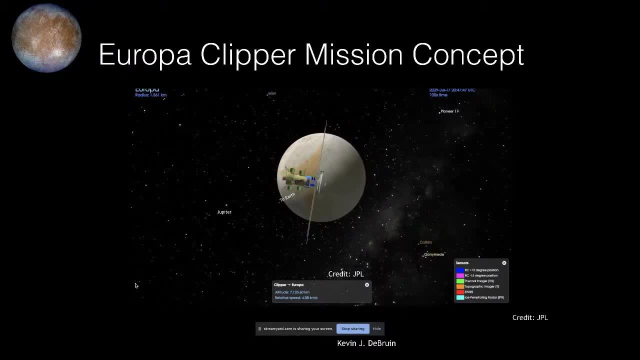 And then we're going to fly and do that again for two and a half years. So we're collecting all this information to see: is Europa actually livable? The word we use is habitable- And if so, we should probably send something to the surface, maybe something like a rover, a lander of sorts, to 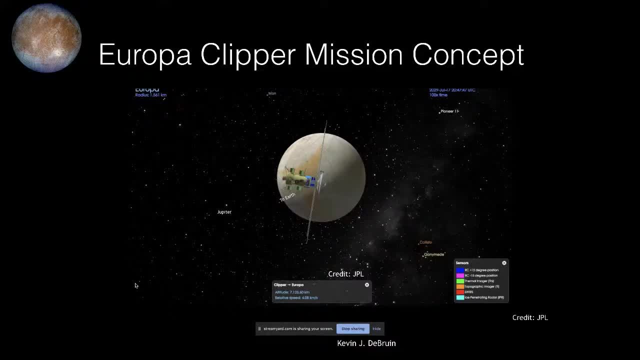 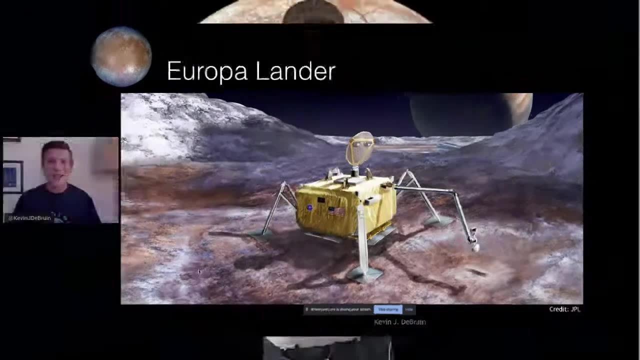 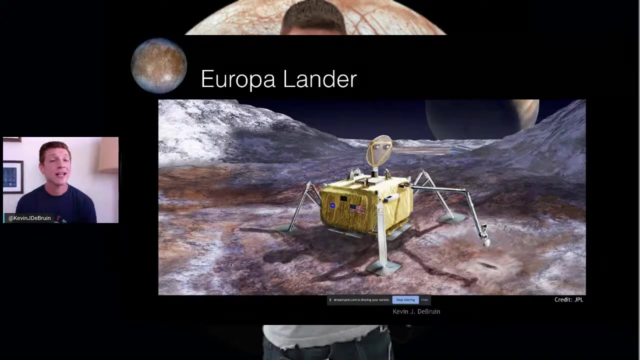 actually test for the signs of life. So Europa Clipper won't be able to find aliens. It's not designed to do that, But we did work on this. This is Europa Lander, the other spacecraft that I helped build. Well, not build design, So this one isn't official, It's not going to be launched yet, But NASA was. 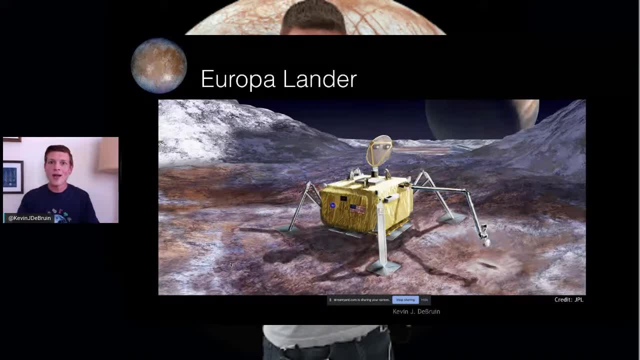 like: okay, if we want to put something on the surface of Europa and see if we can test, like the ice, maybe get down to the ocean a little bit, how are we going to do that? So we designed this. It's a box, It's a big metal box to protect us from the radiation with all of our important. 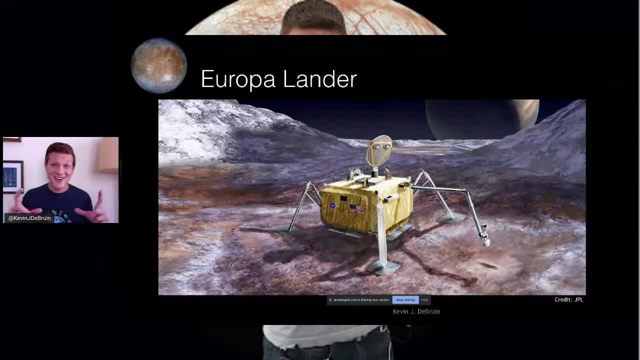 electronics inside. That thing that looks like a face is our antenna. That's our way to communicate home with those two little eyes. Then we got the robotic arm out there with a saw and a shovel on the end of it to saw into the ice. 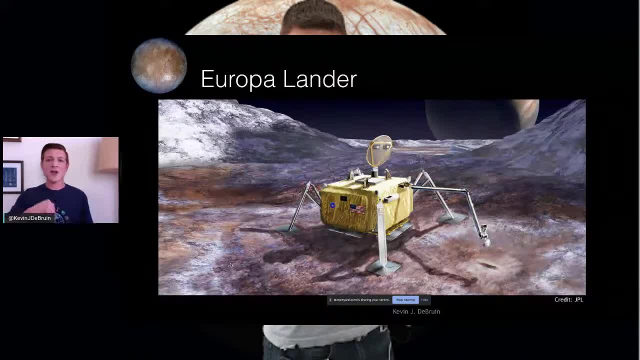 and scoop up some and then put it in a little container that's right on the front, there in the belly, where all the microscopes and stuff are. Now it's not officially going to happen. We really want to, But first Europa Clipper is going to go out and investigate And then, if it finds some, 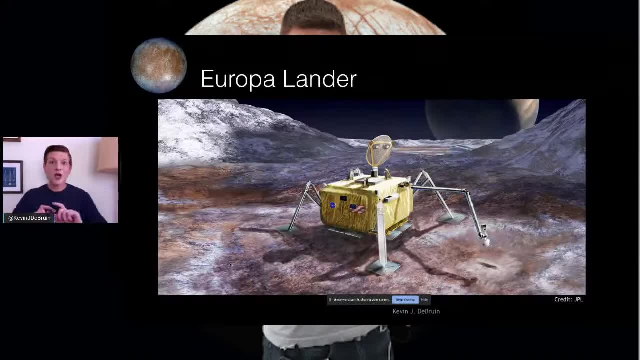 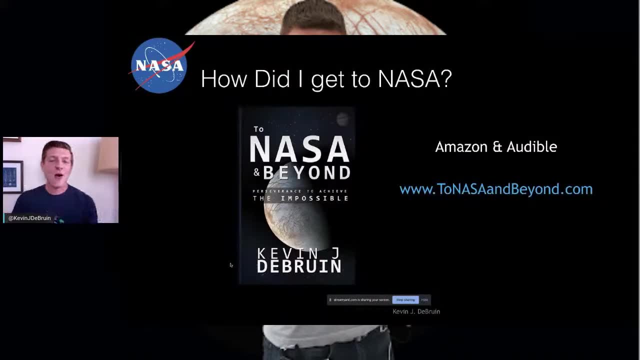 really cool stuff, then NASA is probably going to be like: here's money, Go build Europa Lander and send it off to Europa to find it. Now I really want to quickly touch on how I got into NASA, because if you're out there and you're 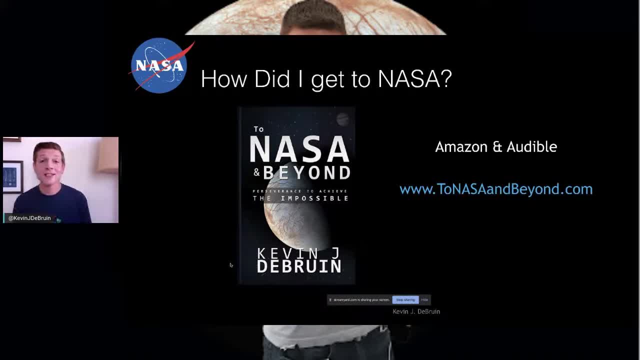 like I want to work for NASA. how do I do it? Well, I wrote a book on it. It's called To NASA and Beyond. It's on Amazon and Audible. This tells you my whole story, but I'm going to tell you a 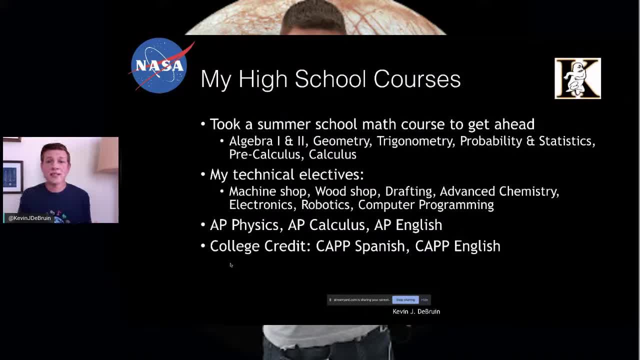 short version right now. So I took a lot of advanced classes as early as I could because I'm like I need to get smart, smarter, I need to work hard. So I took summer school math classes And then I took anything that was like building or design. 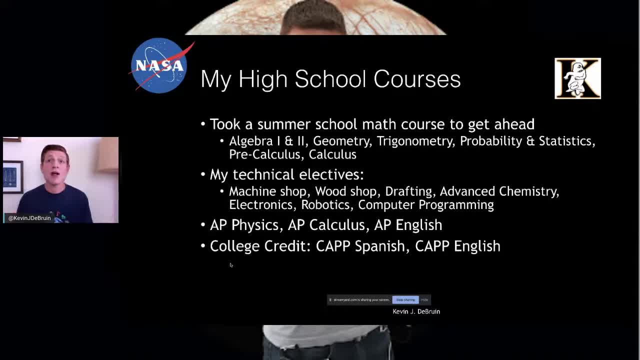 or engineering, like machine shop, wood shop, drafting, computer programming, trying to get all those technical skills as possible And then seeing if I could take any college courses in high school. I tried, took a few of them, Then getting into college. 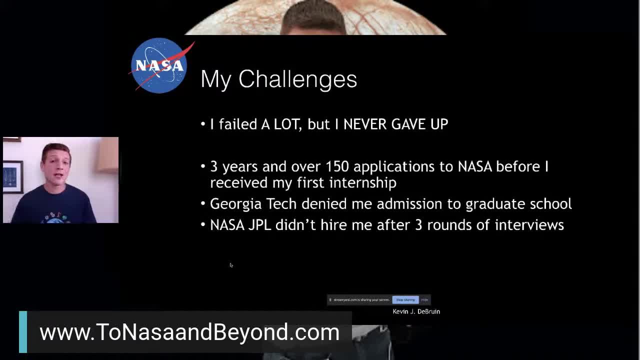 was a little bit difficult for me. I got into undergrad but then I needed to get into grad school. So I like to share this story because my journey into NASA was really tough. I failed a lot when I never gave up. It took me. 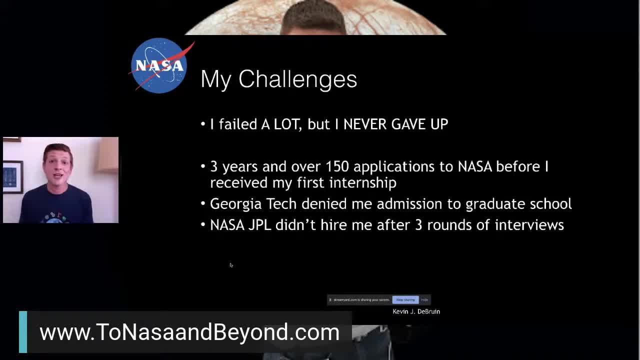 three years and over 150 internship applications before I actually got my first internship. Then I applied to Georgia Tech for grad school. They said no, but then they said yes a couple of weeks later after I was talking to them. And then NASA, JPL- I applied to them. 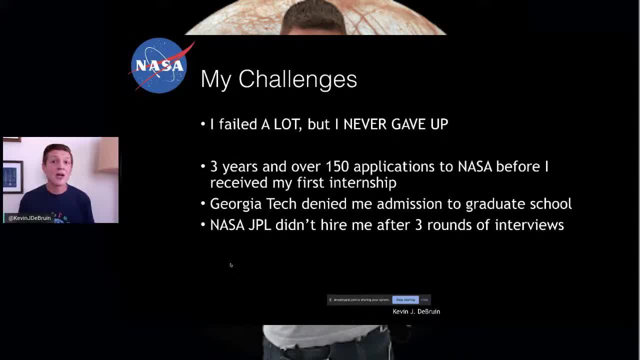 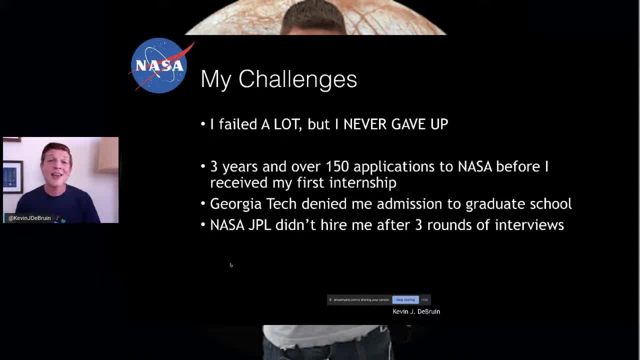 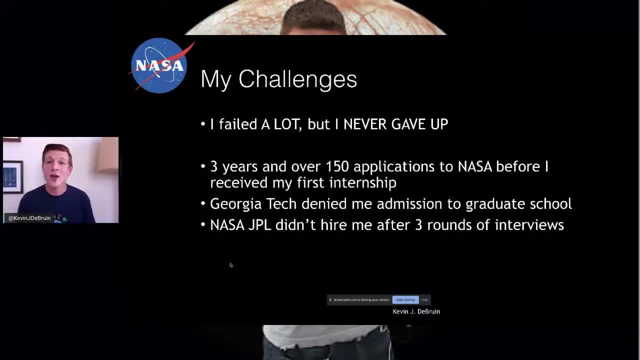 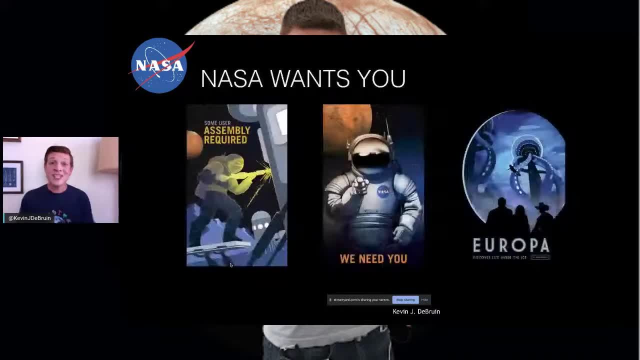 show. it's not impossible, right? Everyone kept telling me no, but if you truly believe in yourself and you're willing to sacrifice and work for it, you can make it happen, because NASA wants you. There are so many different positions that we can fill. I'm an engineer and scientist. 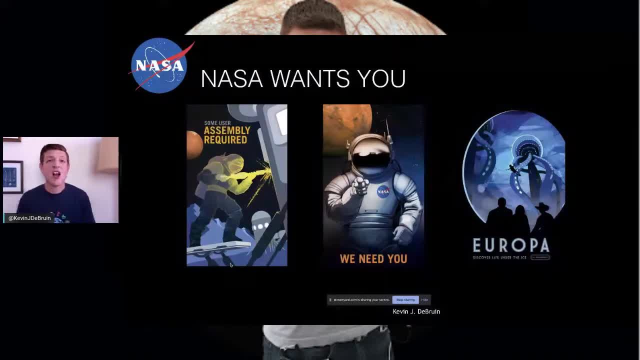 there are. about 80% of us at NASA are engineers and scientists, but we also have managers, we have accountants, we have lawyers, we have artists. So if you're not really feeling the technical side, like math isn't your passion or science, math was not my passion- I had to take a 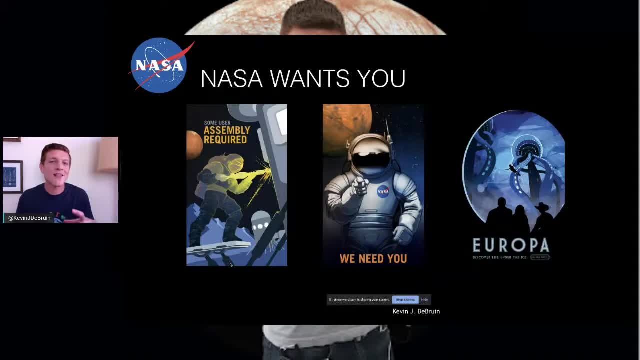 couple of classes, a few times same with science, but I actually wanted to design the spacecraft So I kept going. But if you want to do something else, if you're really passionate about art or design management, you can do that, And I'm an engineer and scientist. So if you're not really 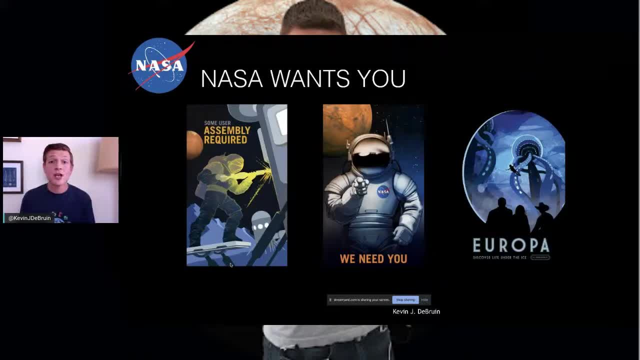 passionate about art or design management, being a lawyer, maybe an attorney, maybe you're really good with numbers. you can find a position within NASA to do that. So we take it all. We want you to help, join us to lead the next generation of explorers to go out and actually put those boots. 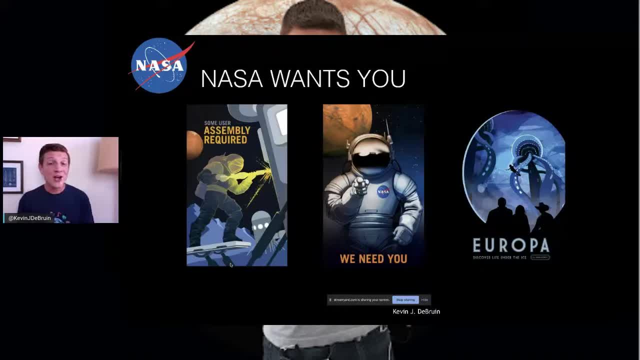 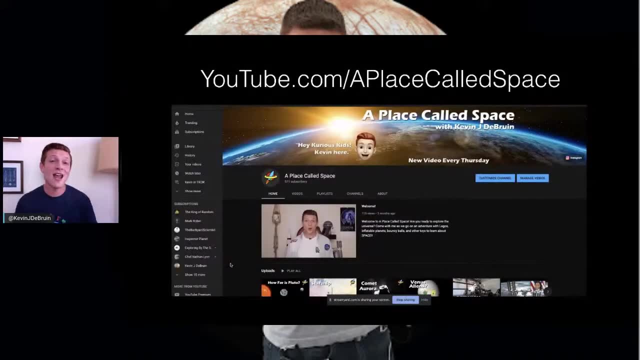 on Mars, because it actually might be one of you that are going to be the first astronauts that are walking around on Mars. It's possible Now. lastly, I'm going to tell you that I teach about space. So it says: former NASA rocket scientist, right? 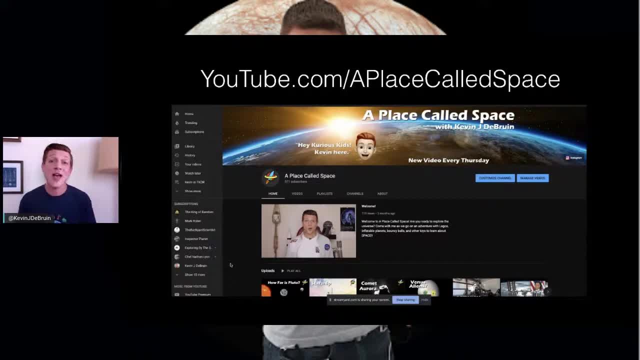 I left NASA to teach people about space, And one place that I do that is on YouTube, where we're at right now, And youtubecom slash, a place called space is where I create a lot of my videos for kids like you who want to learn about space. And, lastly, I do a lot of stuff. 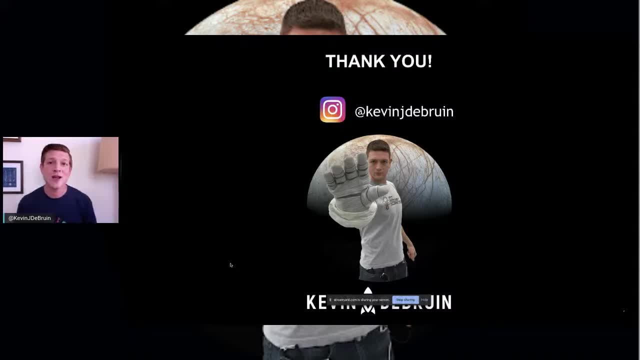 on Instagram as well, at Kevin J DeBruin. right, there is where you can find me on Instagram, And if I'm not able to answer your questions today, if we run out of time, send me a message on Instagram and I answer all of them, because I don't want anyone to knock at their door. 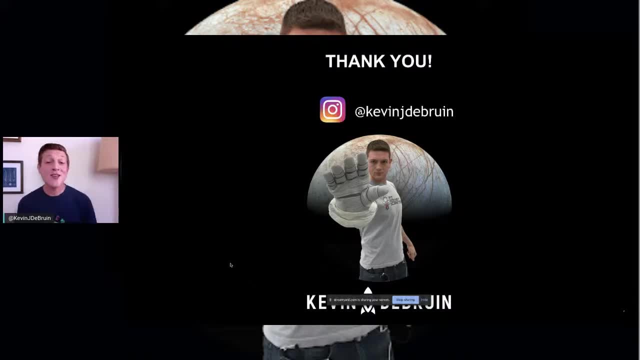 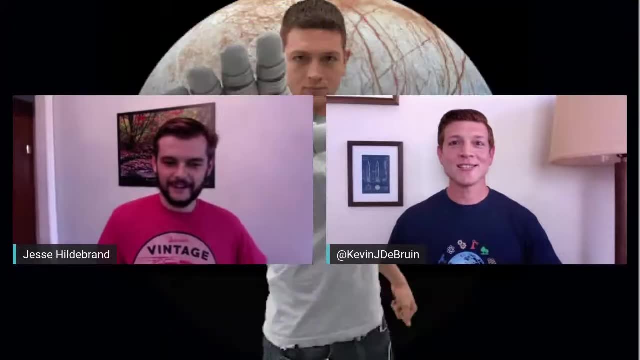 I don't want anyone to have their question answered when they're interested about space. So thank you everybody. Now I want to open it up for questions to see if you have some questions about space science, American Ninja Warrior, anything of this sort. 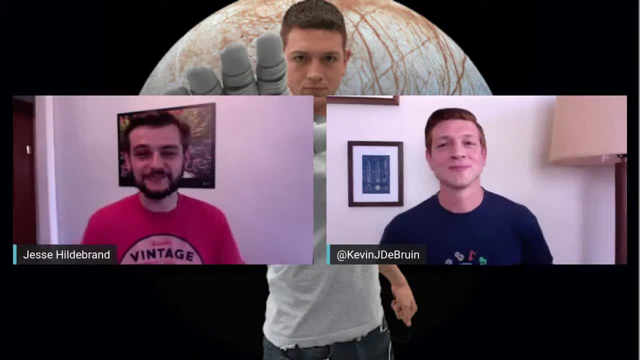 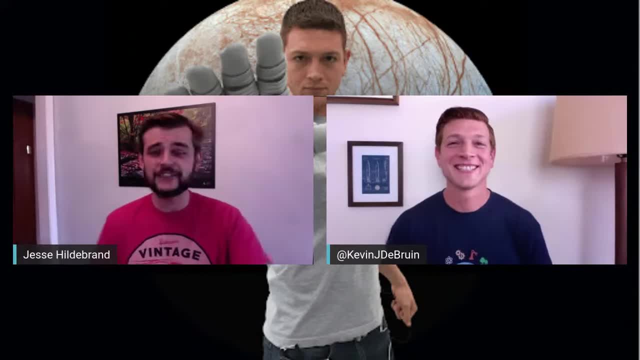 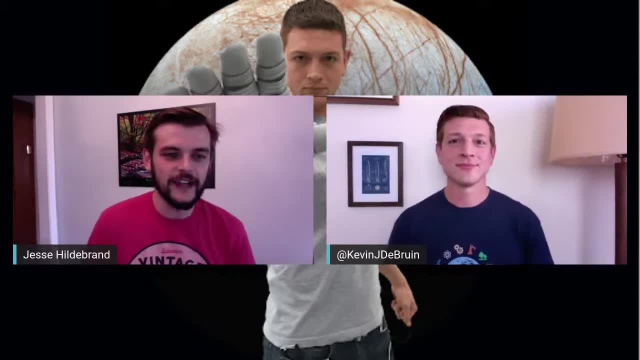 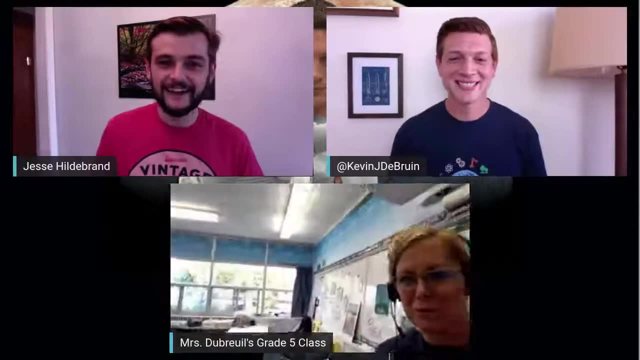 class. They are joining us in Ontario, So welcome in Ms DuBrise's group. You want to share a question with us? Let's do this thing. Hello, We have a few questions, so we don't want to take up everyone's time, but we have a few questions about the spacecraft, So how fast? 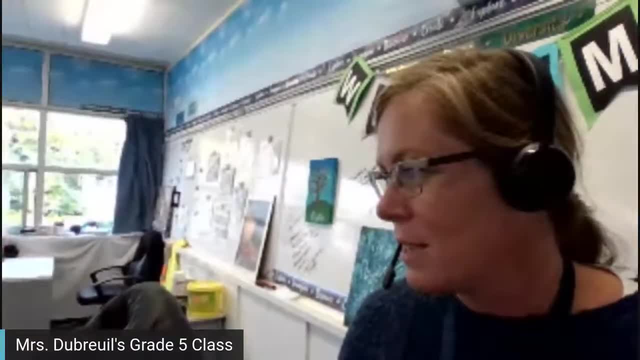 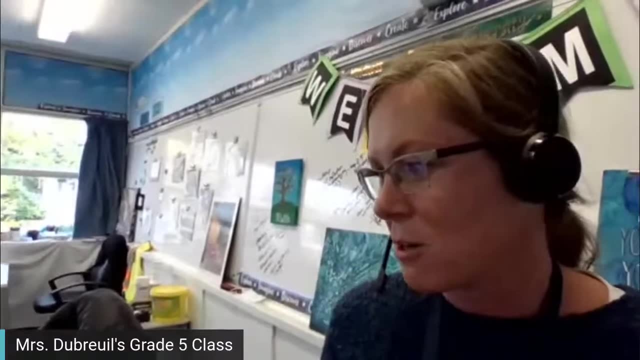 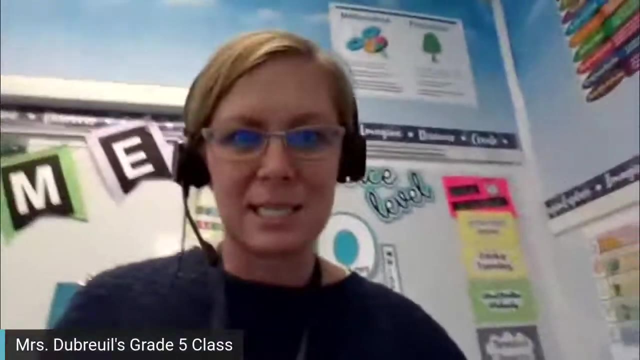 does it travel when it goes from Earth to Europa? Will the Clipper come back after it's done its mission? Will it come back to Earth? And if you need the Europa lander, will you prepare it in case it needs to be sent? or is that just testing right now? All right, Great question. So the first. 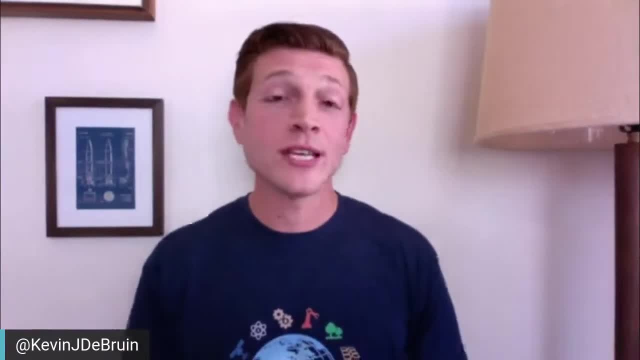 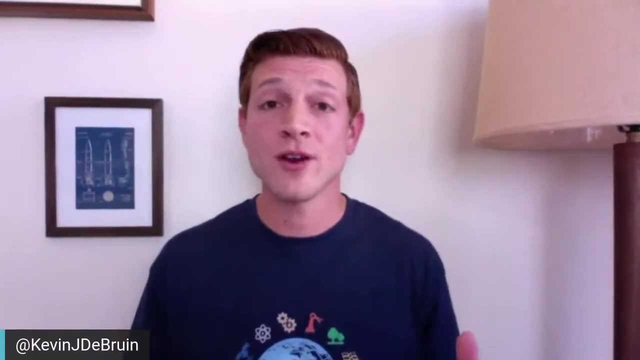 one is: how fast will the spacecraft go? Well, to get off of the surface of Earth, we have to be going at least 17,500 miles an hour, But that only gets you off the surface of Earth, If you want to. leave Earth's orbit, go to the moon, go to Mars, go to beyond. you have to go at least 25,000 miles per hour, So we'll be going at least that fast. Now Europa Clipper is supposed to go aboard the 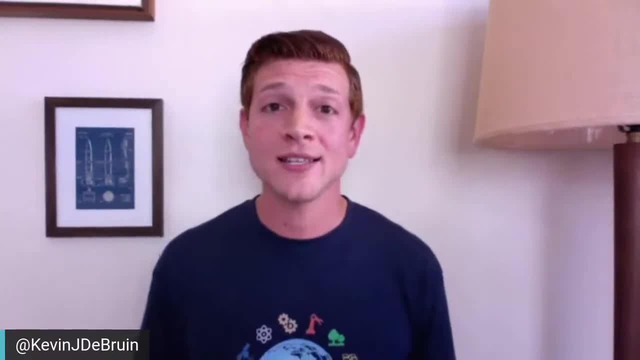 SLS, That's the Space Launch System, the new rocket that NASA is designing, And we're going to put that thing in like Ferrari mode and shoot straight to Jupiter, instead of doing flybys, which you may have heard of before, where we have to build up speed. 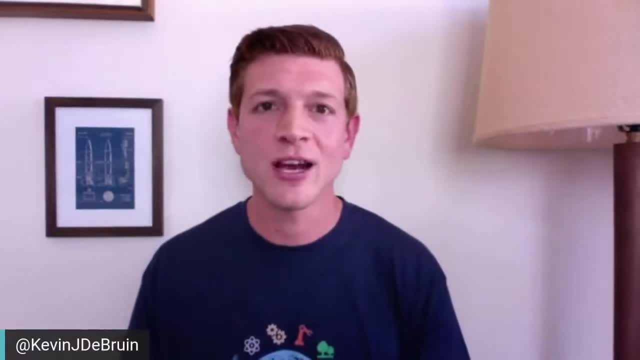 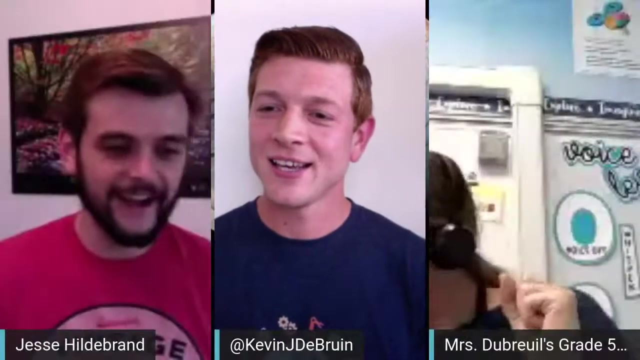 by flying back around Earth and stealing some gravity and going out there. So we're still waiting to see exactly what the SLS can do. Once it's fully done, it will be going at least 25,000 miles an hour. Now the second one: what was that? second question was: Oh shoot, What was it? 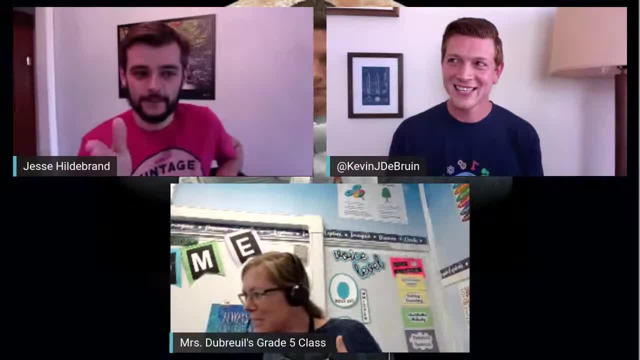 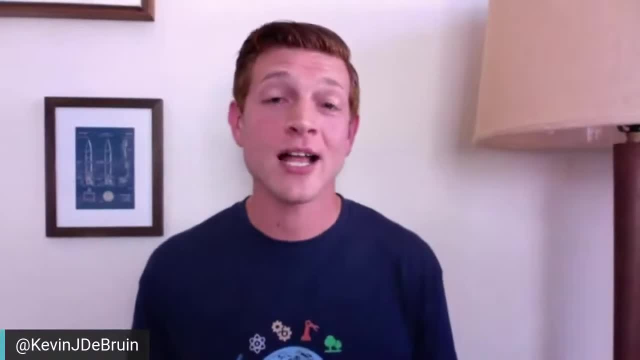 Is there life on Europa? I don't know. if that was it, Oh, will it come back to Earth? Will it come back to Earth? No, it will not, Because to come back to Earth we need to add more fuel so it can leave the Jupiter system and come all the way back to Earth And it's not worth it for us. So what we're actually probably going to do is crash it into. Jupiter is most likely what's going to happen. We've done that with other spacecrafts in the past, where we crash them into planets to make sure that they don't. 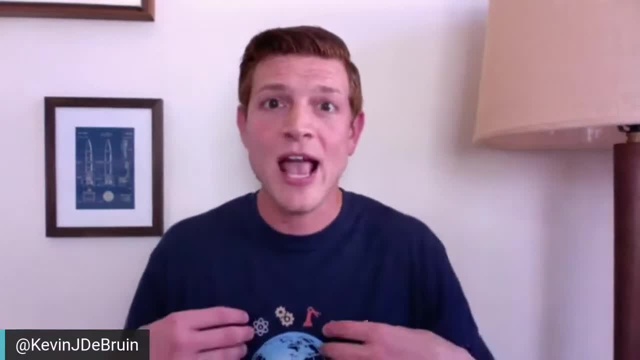 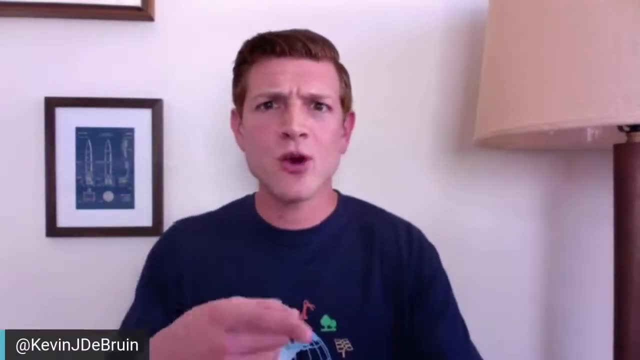 accidentally crash into a moon that has life, And then we accidentally put Earth bugs all over that place And we might find bugs and then go: hey, but these are Earth bugs or are they Europa Clipper? We don't know, So we're not going to bring the Europa Clipper back. And lastly about 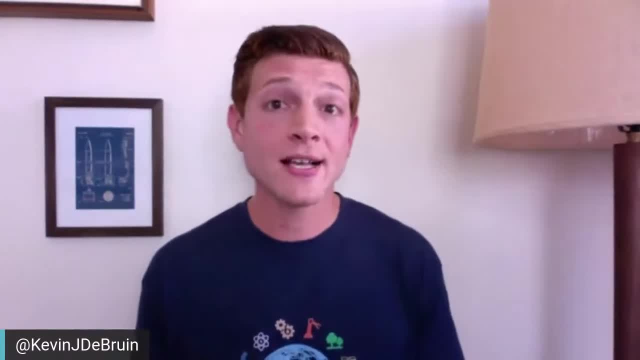 the lander. Well, we prepare it just in case. Well, NASA asked us to look at a couple different things. They asked us if we want to launch Clipper and lander together, what is that going to look like and how much is it going to cost? And through all of the trade space, we did many. 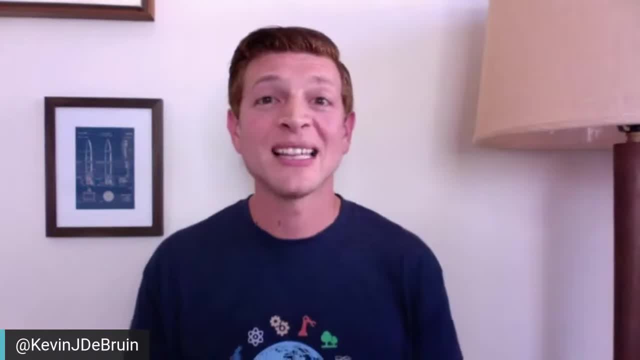 different design studies. The best thing to do was to launch Europa lander later Now. if NASA does want to give us the money to build it, we will do that right now And launch it a few years after Clipper. That was our game plan. That's what it's set up to do. 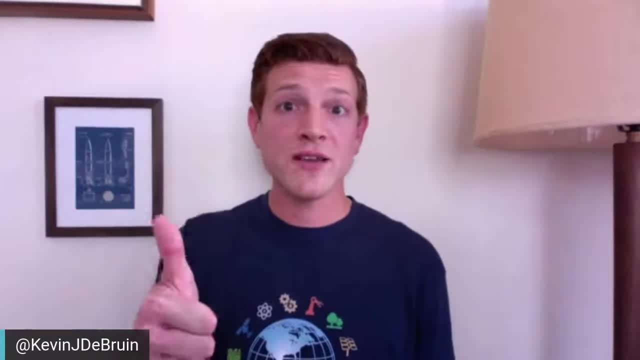 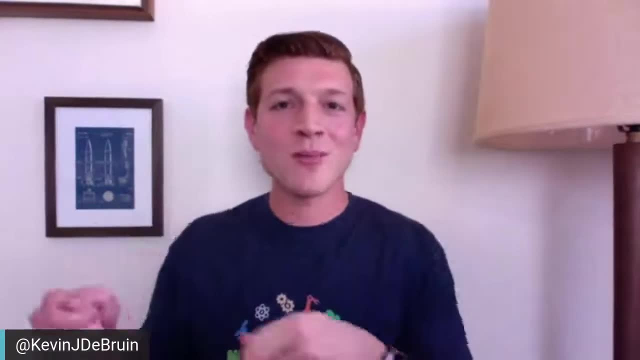 if NASA decides to go, yes, do it, We're going to give you the money, build it, design it, finish it up, send it out there. Well, right now it's just kind of put in a box. we put a bone on. 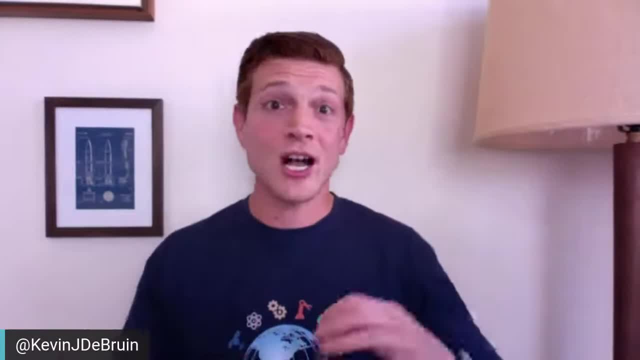 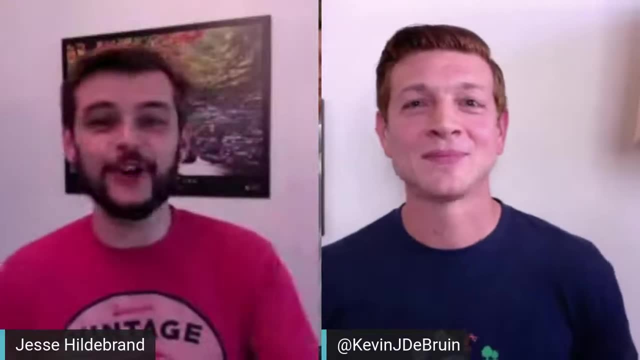 it, put it on the shelf And if NASA tells us to dust it off, we'll dust it off, refresh it and then build it and send it out there. Great question, It is a great question. to kick us off, We're going to go to all our teachers in succession. 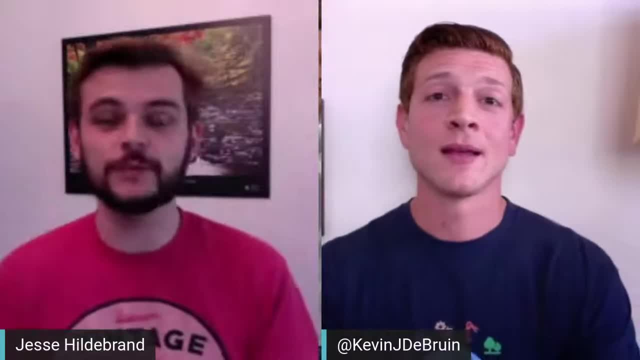 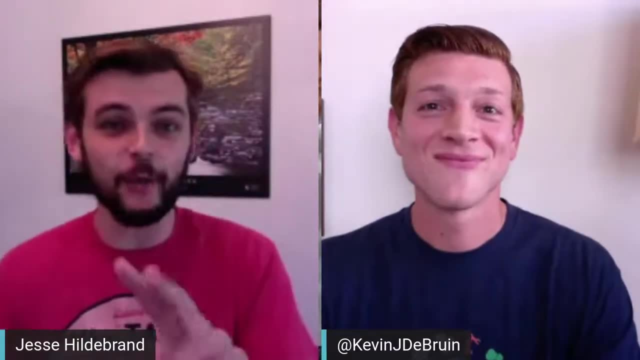 And, by the way, Kevin, you end your presentation with. something I love when we talk about space is that if you're keen on space, there are so many avenues to get involved in NASA and Canadian Space Agency- whatever you're keen on, But no matter what you're doing. 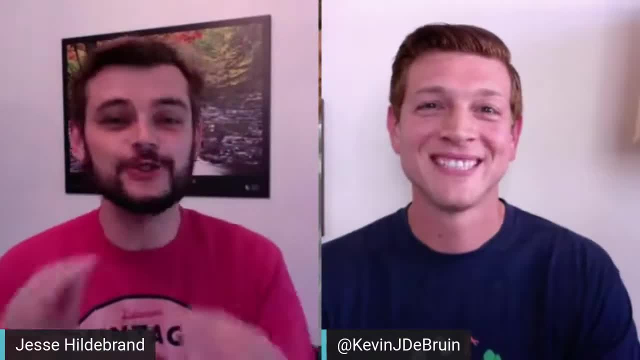 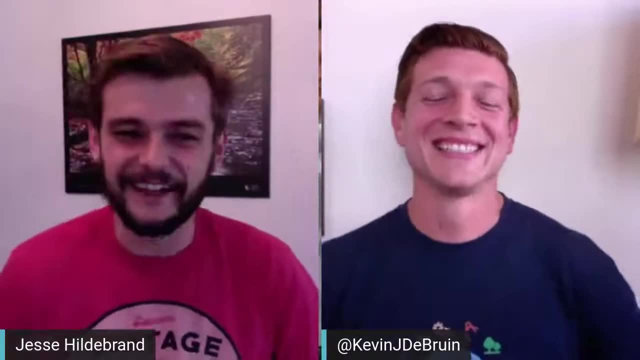 kids. if you find something you're as passionate about as Kevin is about space, do that, Because if you can be this keen, it's a great career, And I'm sure Kevin would tell you that every single day. Ms Hamilton joined us for the first time ever in Toronto, Ontario, So 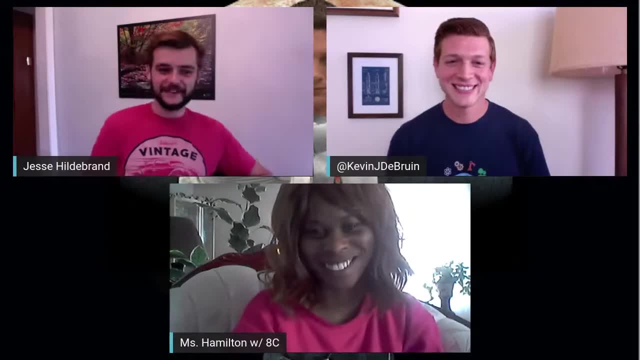 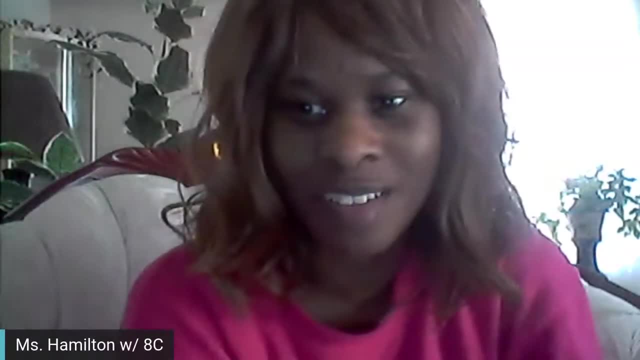 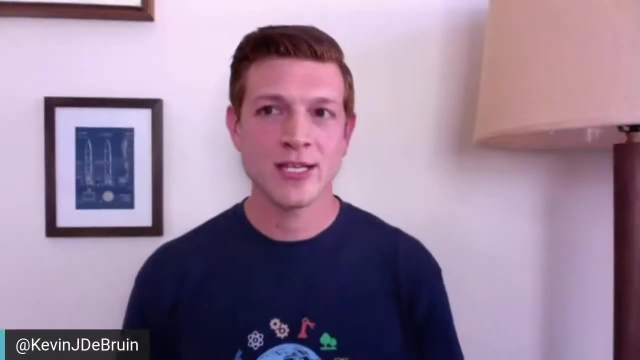 welcome in, Ms Hamilton. If you want to share a question with us, go for it. Okay, So one of my students wanted to know what happens to a failed spaceship. I've got like three questions, but that's like the first one. Yeah, What happens to a failed spaceship? I'm going to take that a. couple different ways. So sometimes our rockets fail when we launch them And that means unfortunately the spacecraft blows up. And luckily sometimes we build two just in case, or we build one to keep on Earth so we can test. Then we turn that one into the real one and launch. 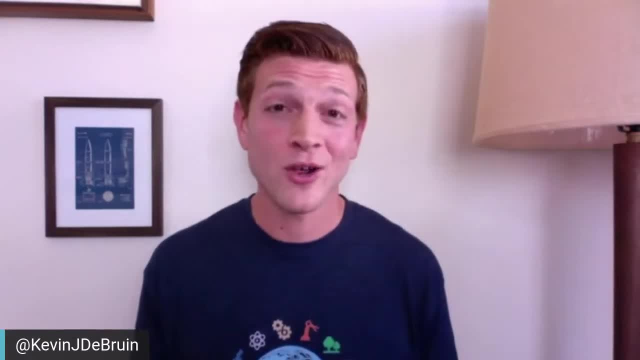 it. Sometimes it just goes wrong, And then we have to do something about it, And that's what we're going to do, And then we have to build it all over from scratch, if they give us the money to do that. The other way is like let's say it's a failed spacecraft in outer space. We've had that. 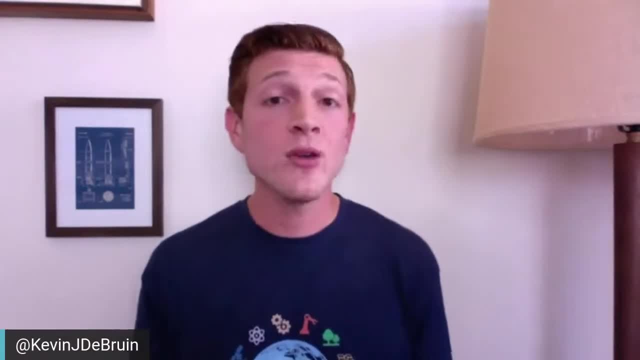 happen where things don't always work right, And we can communicate with the spacecraft with an antenna So we can send them information. They can send us information, figure out maybe what's going wrong. We do the best we can to create software patches, So do the computer code. 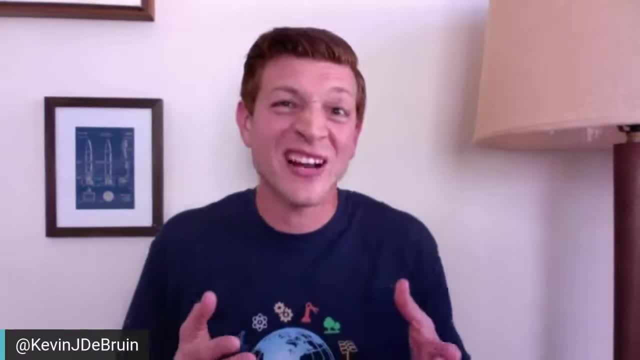 send it up there to try and get the spacecraft back working and try to like limp it a little bit And then we can send it back to the spacecraft And then we can send it back to the long kind of like give the spacecraft crutches to see if it can continue to do some of the 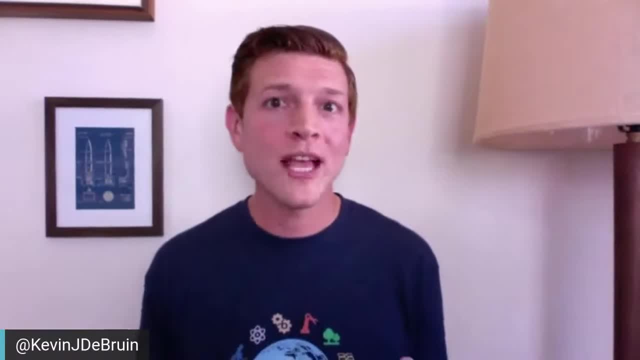 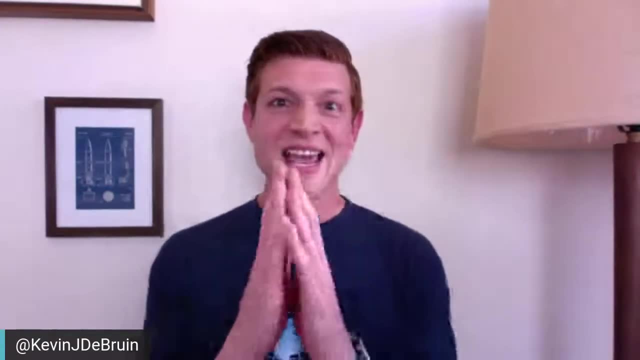 mission, And that happened with the Galileo spacecraft, which is the one that taught us a lot about Jupiter and the Galilean moons, when it was launched back in 1989.. The antenna didn't deploy. The big one didn't deploy, It didn't work, So we had to use a really tiny one that was like: 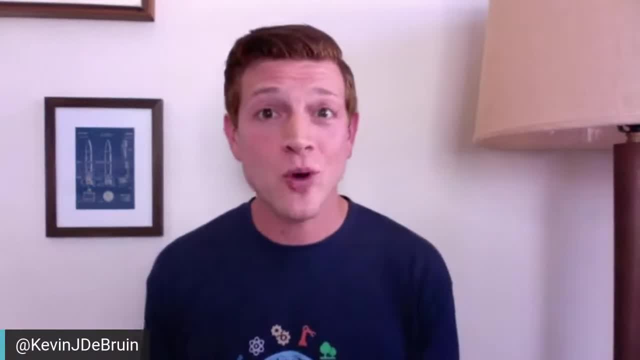 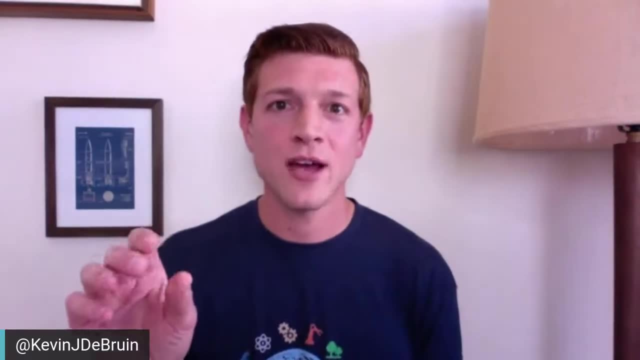 you might not understand, but it's like using dial up versus current Wi-Fi and internet speeds Just takes a really, really long time. It's like sending information very slowly, So we do our best to repair them and send them along the way. 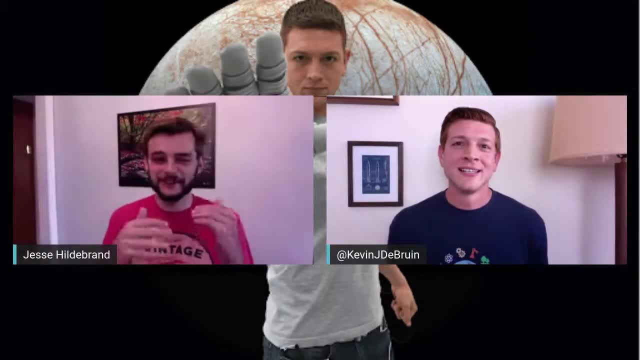 Kevin, it's really distressing to me that the two of us know what dial up is and we have to sort of explain that It'd be something to kids who have no idea what we're talking about. Oh well, getting old, Very slow internet, Very, very slow internet. 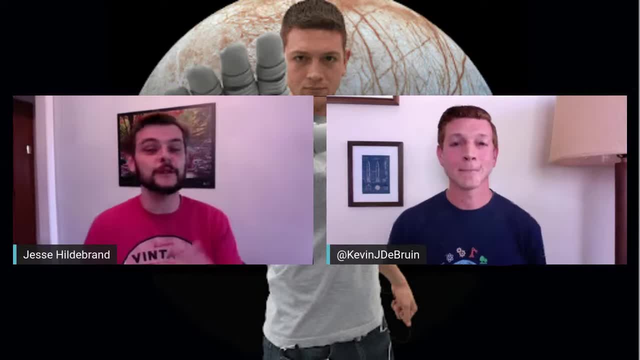 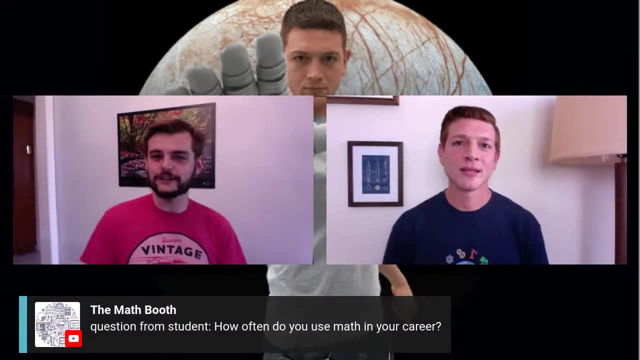 I'm going to go to Ms Cum's class in the story in just a second, but I love this question from the math booth. So we've got a high school math teacher in Nevada, in Las Vegas. They want to ask: how often do you use math in your career, Kevin? Every single day. We use math every single day. 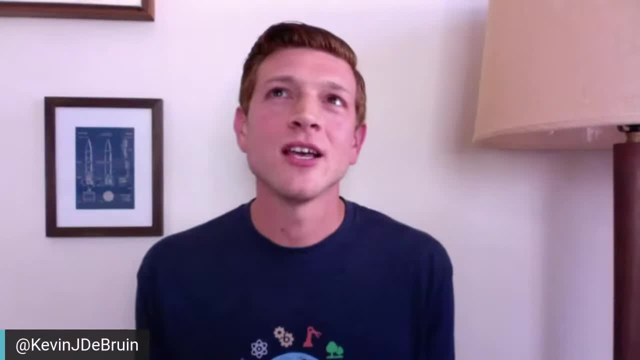 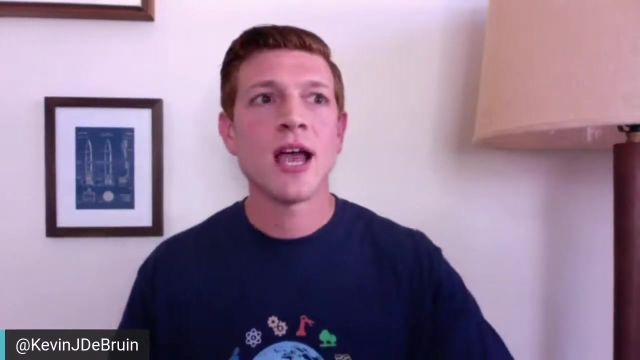 So I ended up going- let's see through, like six math classes past Calculus 1.. So it's Calc 1, Calc 2, Calc 3, differential equations, linear algebra, computer computational methods, And then there were a few others like linear regression, like all of the math behind Excel. 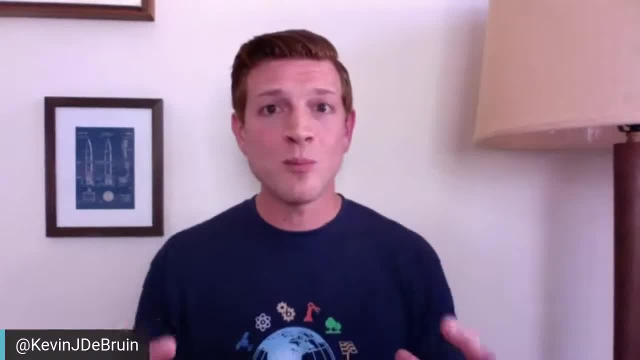 I learned how to do that by hand And we use math all the time to build computer simulations and computer code to help us design our spacecraft- And not only to help design the spacecraft, but we're taking all of this data. Then we need a way to analyze the data. It starts as ones and 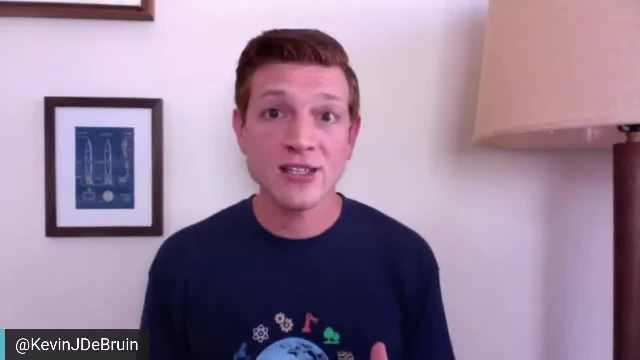 zeros, which is just binary code, And then we have to convert that into actual data that we can use, And then we use the math to study our data, to understand it, to see if what we're studying is is exactly what we're looking for And it's used all the time. The biggest thing I will say with the 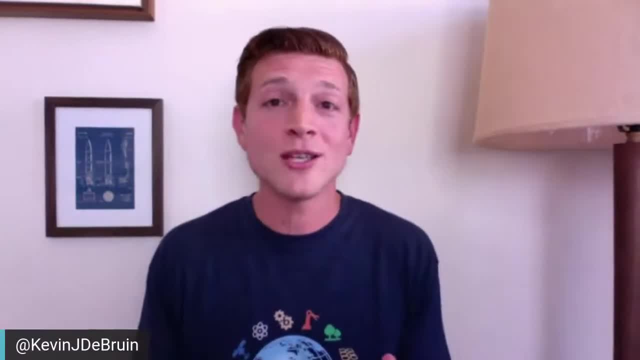 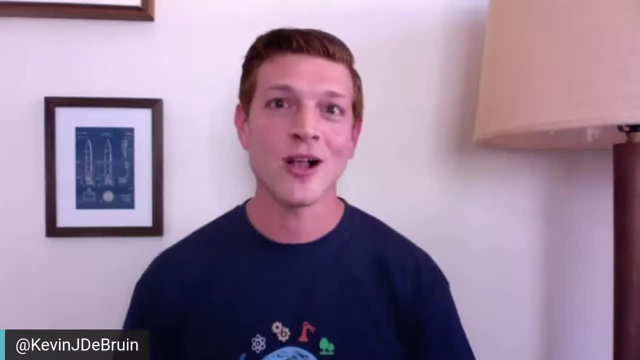 math is that you need to know enough to then build your computer simulation And then the computer does all the hard work. but you have to put all the good quality stuff into the computer to get good quality stuff out of it. Fantastic, I'm so glad we got that question. Thanks so much to the. 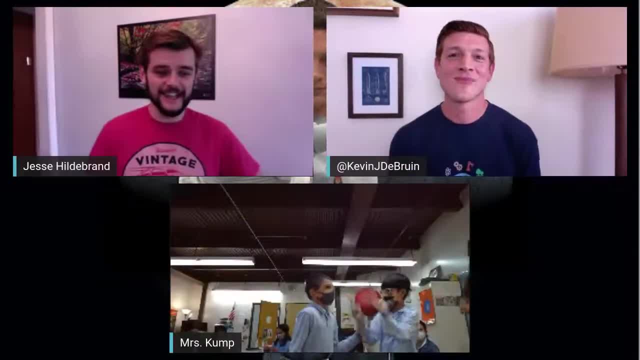 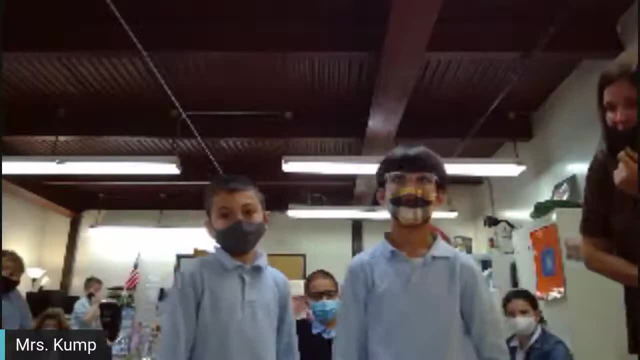 school. So let's go to Ms Kump's class. Come on in, guys, and take us away. All right, How big does the speech pack get? How big is it? How big is it So? can you have life on Europa? 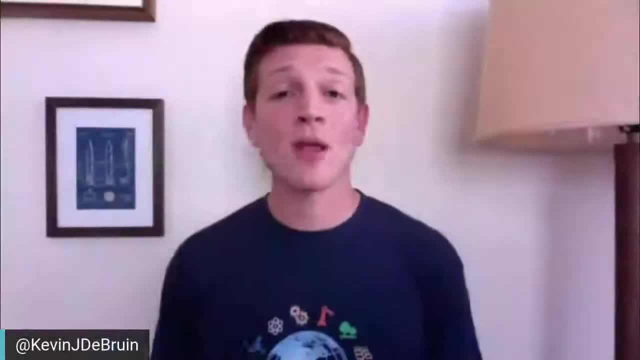 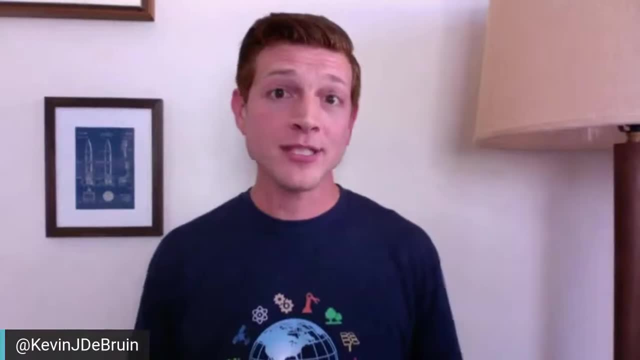 Can you live on Europa? And how big is the spacecraft? Okay, cool. How big is the spacecraft? It's gigantic. So I'm? I'm six foot four. If I'm standing next to the spacecraft, it's taller than me, Right? And if I put my arms out I'd have to. 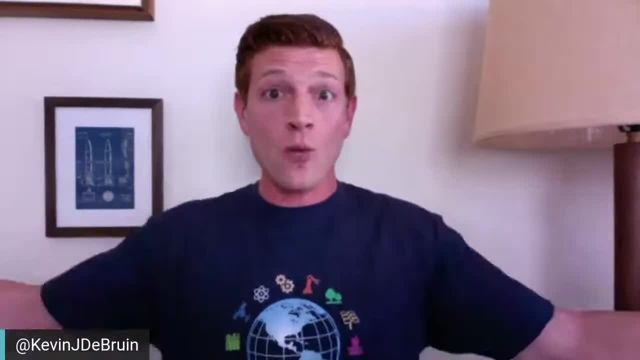 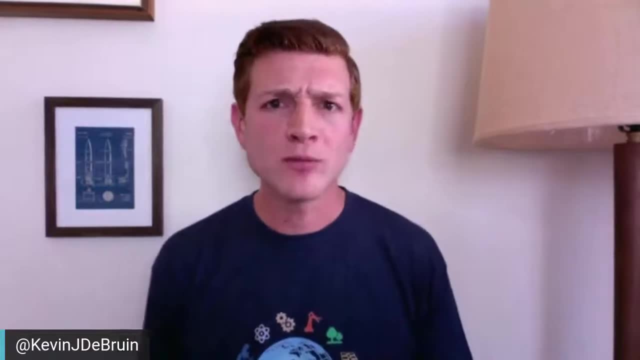 put my arms out like 10 times to get all the way across it. So it's pretty big. It's big, And then can we live on Europa? No, So there's no atmosphere on Europa. This is, we're in the. 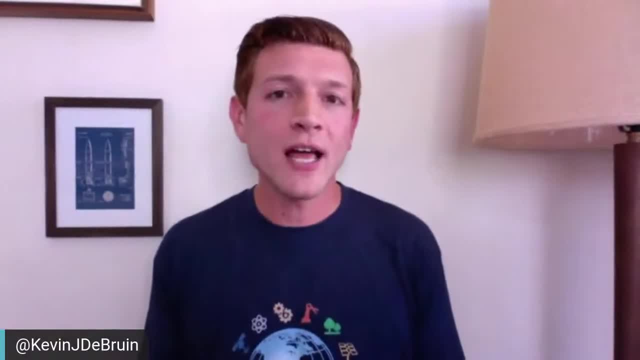 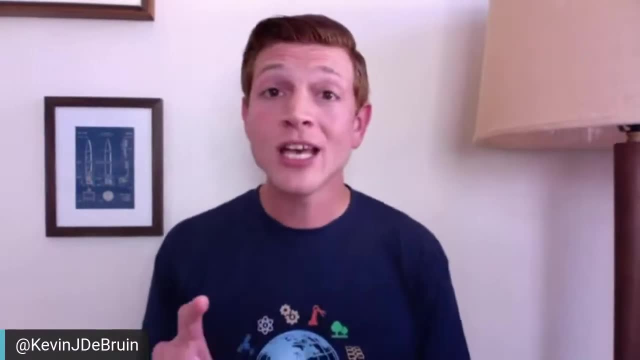 atmosphere. right now We're breathing air. We think that the life on Europa is those tiny little microbes in the ocean. So it's down in the ocean. So maybe it is possible if we built like submarines to live in on Europa. That's something that we could do, But on the surface there's too much. 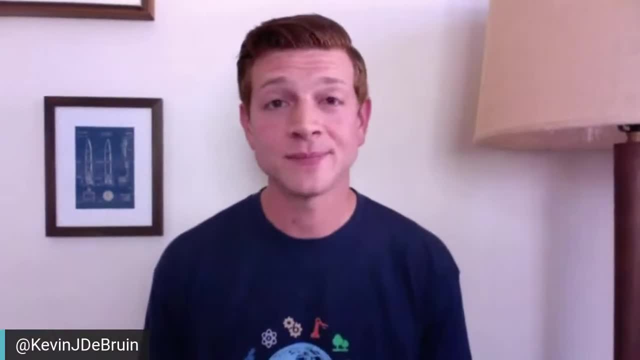 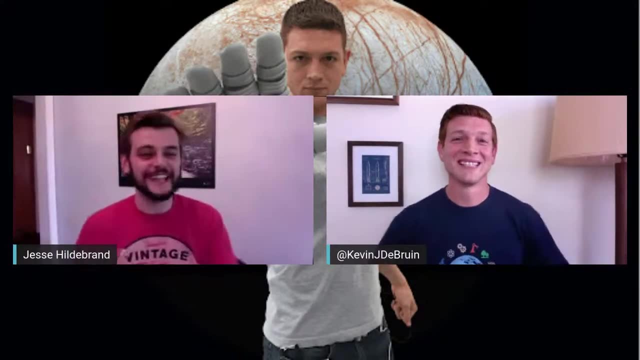 radiation and it's too cold, We wouldn't last very long. Good question, It is Sorry. It's just so funny watching you compared to other space you'll bring on, because one of the questions we often get and I hate to take it away if a kid's going to ask me, but it's like 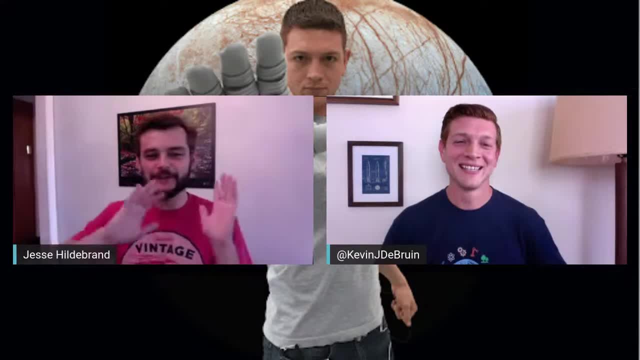 would you go to space if you could, And I think you'd be like in the first: the first rocket into the submarine, into the European ocean. so fast, Awesome man. All right, I'm going to go to Ms Hood's class. She's in Ackland, Pennsylvania. 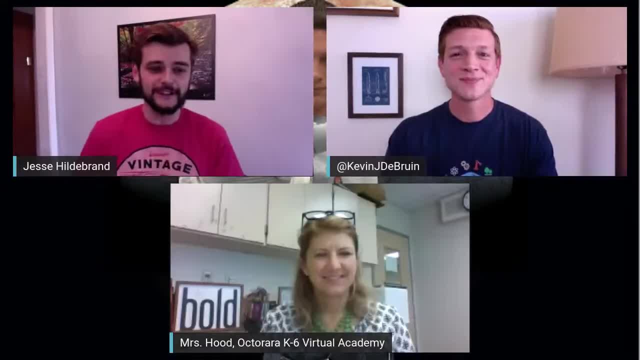 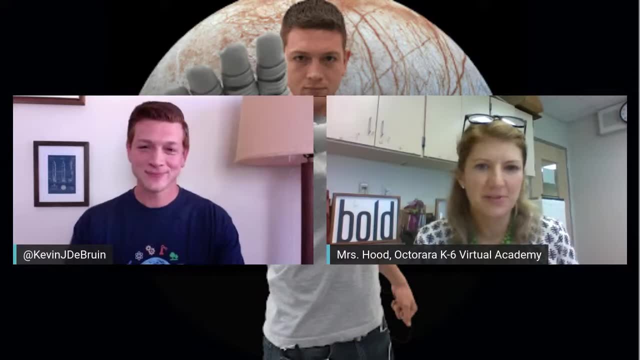 We're going to come to Norway Middle School and Ms Gualtieri's in a minute, but, Ms Hood, take us away, Come on up, Hi Kevin. Hello, I first want to thank you for giving the message of perseverance to our students who are learning. 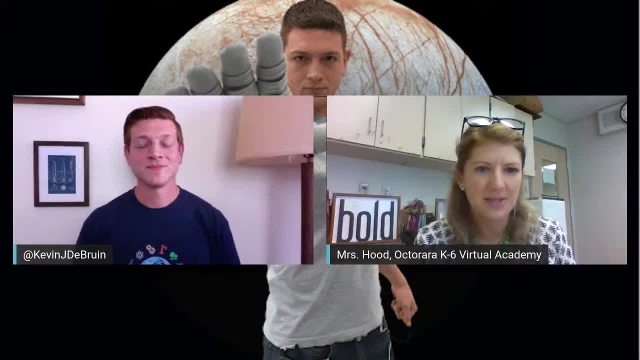 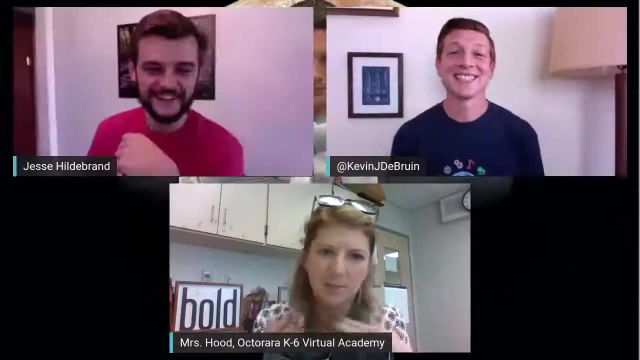 virtually from home. I think that is a great message that they can take something from. Our question is: how often have your expertise that you used for Ninja Warrior and your expertise as a rocket scientist, how often have they like, come together or overlapped for you? 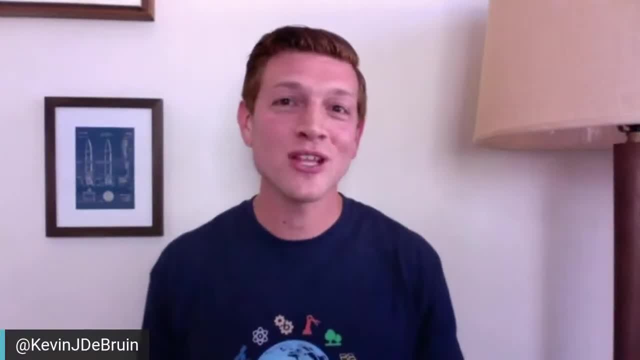 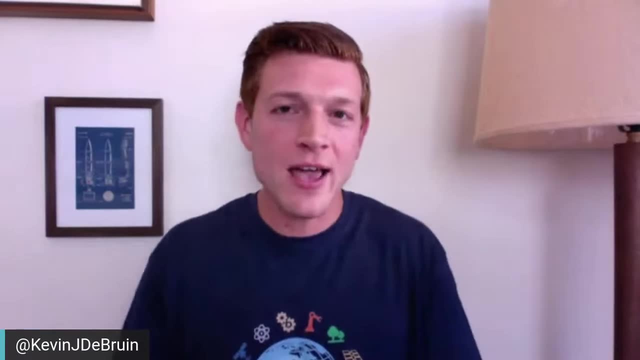 I like it. I love this question And it's something I normally try. I like fit into every single presentation, But what I like to say is: like the reason I like am an American or like am a rocket scientist is because I was an American Ninja Warrior. 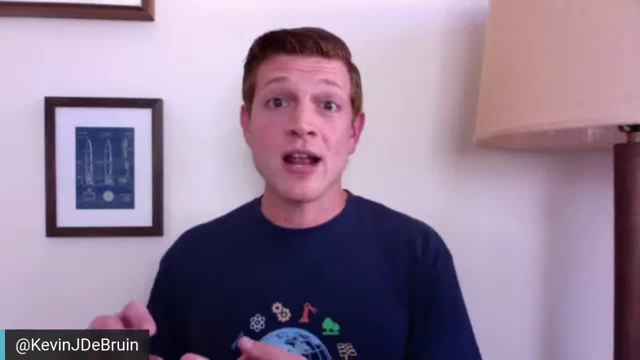 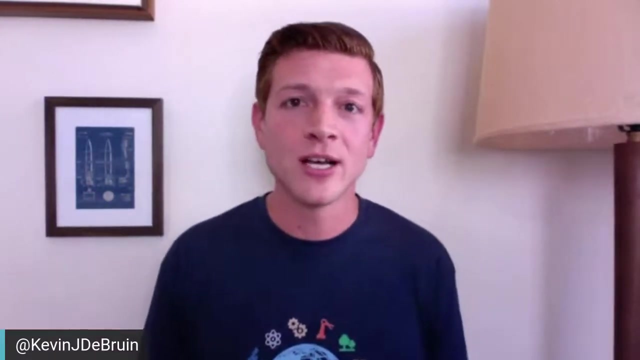 So the fitness side of me, like eating right, exercising really helps my brain right. Like it has been shown that immediately during and immediately after exercise your brain retains more information. You can learn more things and then hold on to it. So when school got tough and when work got tough, I would take a break, go for a run, go to the gym to lift. 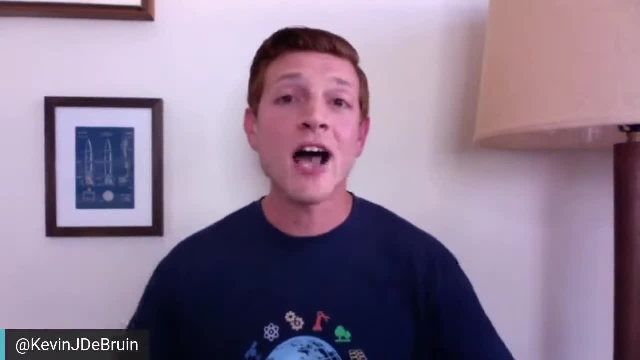 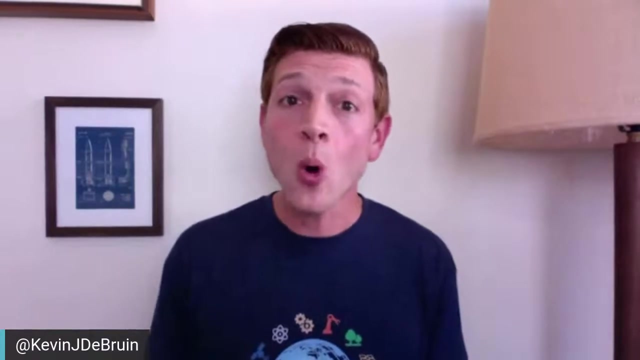 some weights, do some jumping jacks, just go for a walk around to help reset my system, And then I would come back and I would be able to solve the problem. I would like. I like to say that if I'm working on code, I can sit and try and figure it out. if I'm like at a standstill for like four hours Or I can. 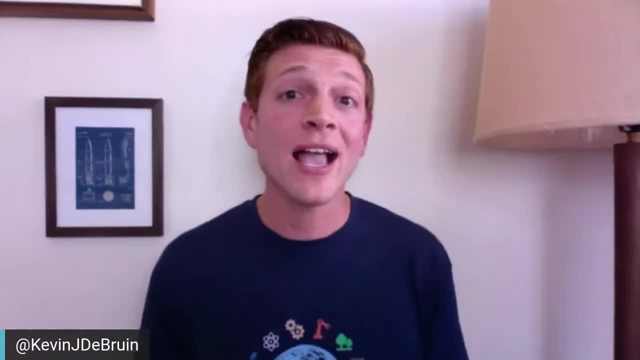 take a half hour break to walk around, go for a run, come back and I will finish that code In about 30 minutes. So it saves time, it resets your system, you're able to think more clearly, you have more energy and stamina to continue on and actually do rocket science, which is what 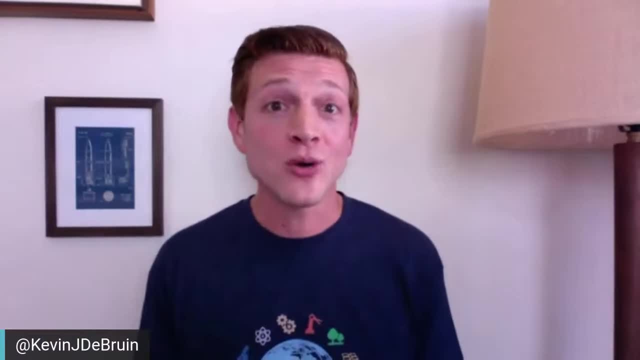 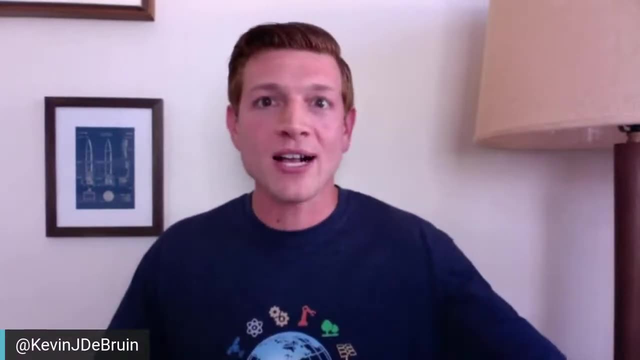 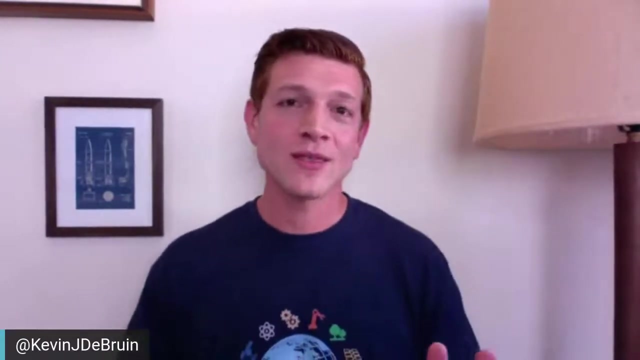 you'd be doing eight to 10 to 12 hours a day. So it actually overlaps a lot. It's not like: how am I able to do Ninja Warrior and be a rocket scientist? Like, without Ninja Warrior I wouldn't be able to do my rocket science. So like. 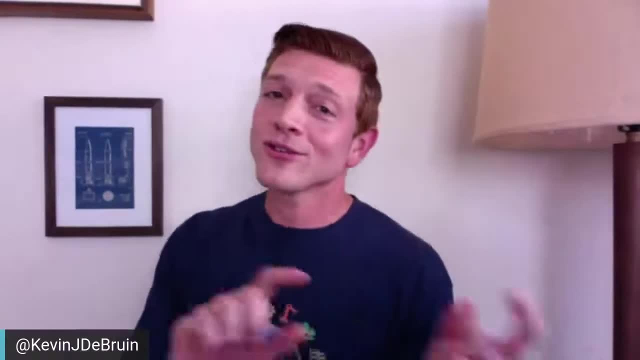 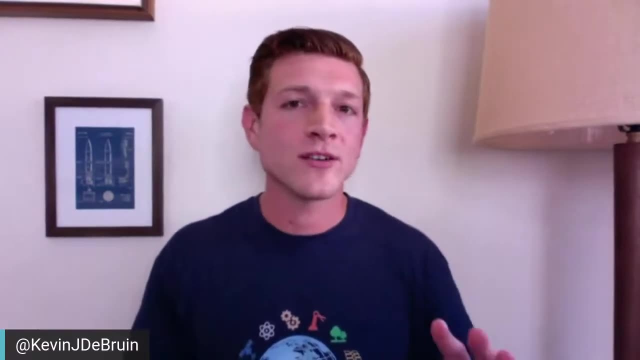 the. the health and fitness aspect crossover a lot. Now let's throw it on the on the ninja side. right, Ninja is a puzzle. It's not like just running or lifting weights or you pick stuff up, put it down. I did that, I was a bodybuilder. move to the ninja because I have to figure it out with. 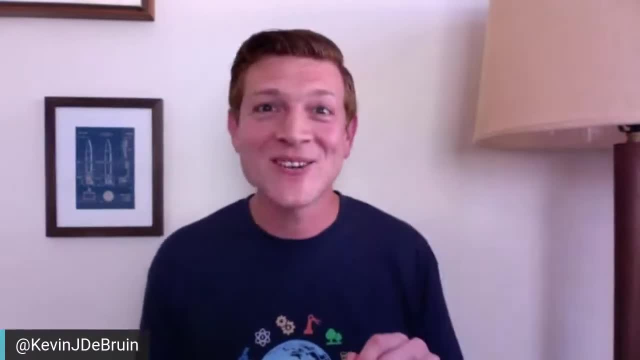 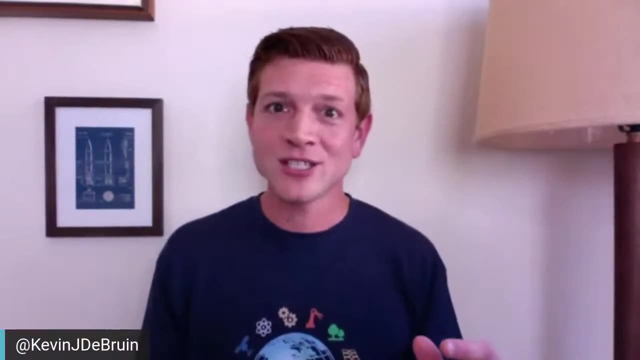 my brain. It's like what angles this honestly goes through my head would be best to put my foot at, to hold that what is going to be the moment arm. So that's a, that's a physics term. right there, You know, moment arm is here. 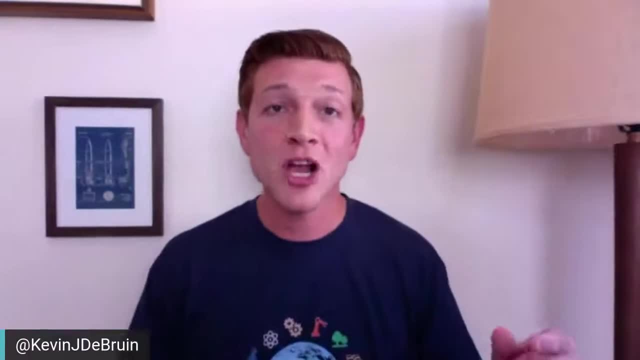 It's like pivoting around: the longer it is, the more torque and momentum can go. I'm like, okay, well, I want to keep my body tight. So actually I go through the physics and math in my head when I'm looking at a new obstacle and the best way to do it crosses over a lot more than you. 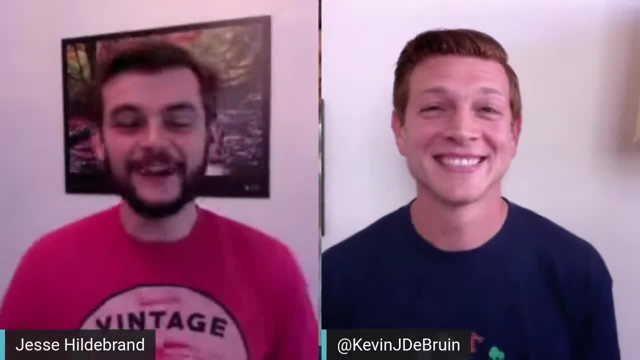 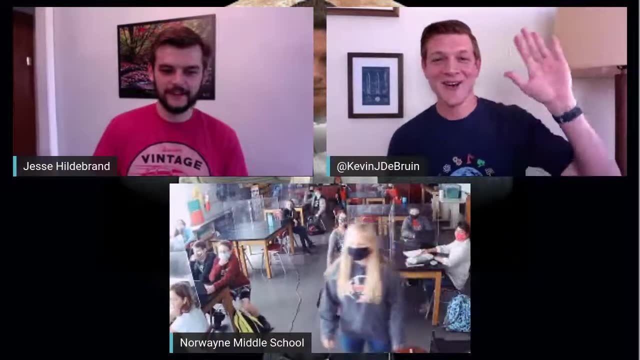 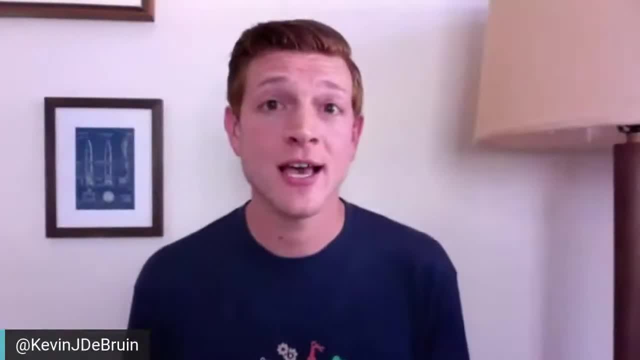 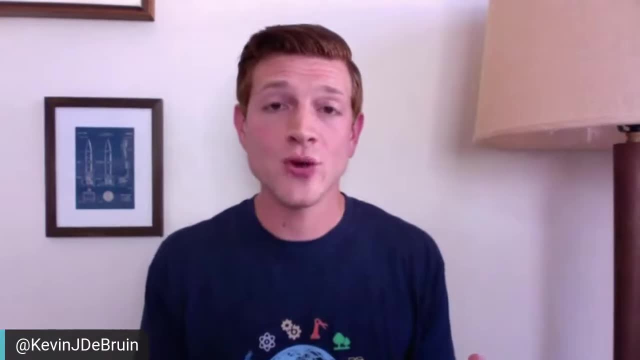 Hi. So what coding environment do you use for spacecraft development? What coding environment do I use for spacecraft design? My main one that I use is Python, if you've heard of that, And the UI that I use is called Spyder S-P-Y-D-E-R, And that's how I 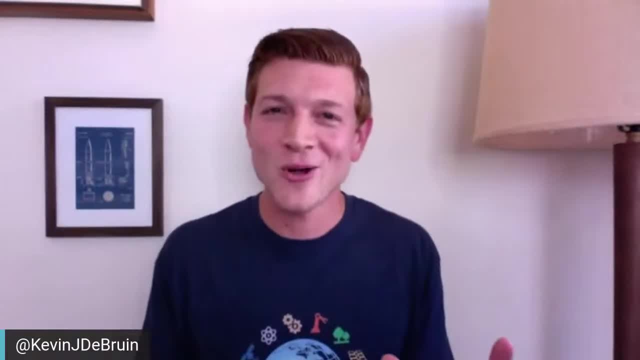 implement my Python. This is kind of advanced. You kind of need to know a little bit about coding and what I'm talking about. But Python is the main one I've used. Matlab is used a lot, VBA, Visual Basic- for Applications- that's the coding behind Microsoft Excel. 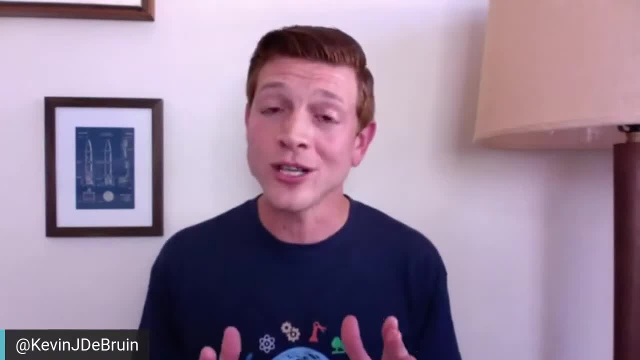 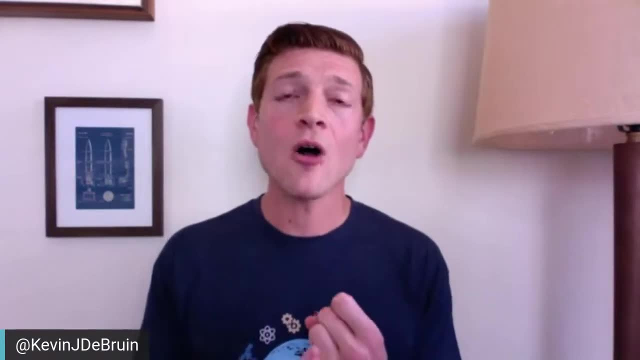 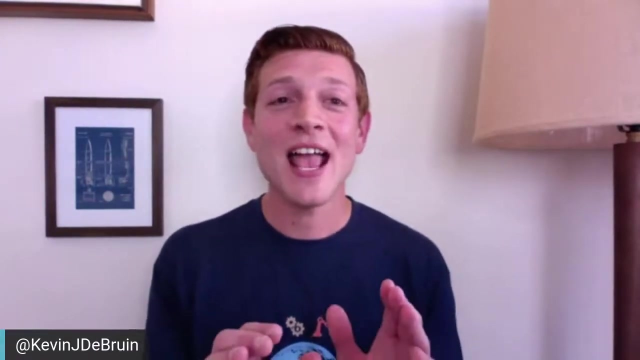 Microsoft PowerPoint. We use that a lot. We use a lot of Excel to build up simulations. So it would be Python, MATLAB, VBA And also the two I will say is Jython, which is Java, Python together. That's crazy, But that helps run MBSE. So it's model-based systems engineering where we implement. 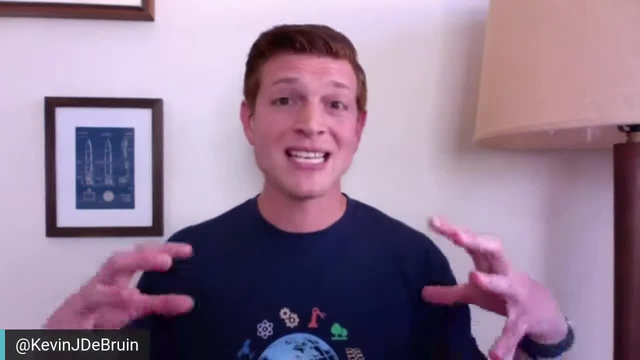 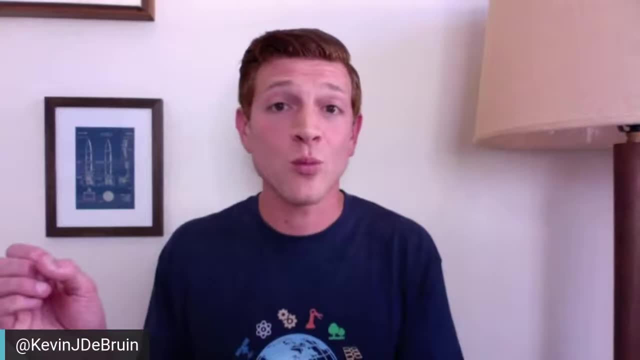 the systems modeling language, SysML, to design our spacecrafts in a computer situation environment where it's not just like the physical model of the computer but we're putting in requirements, So sentences of saying what the spacecraft has to do, and we can link those up to people. So I am 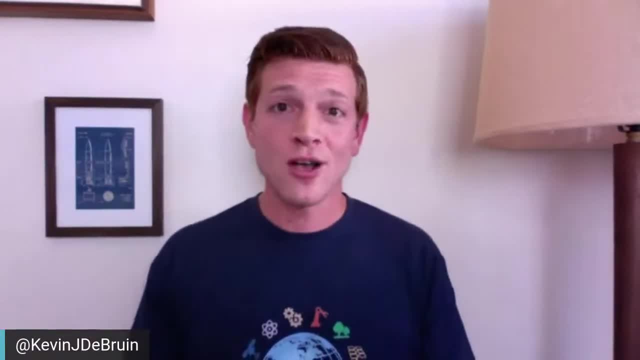 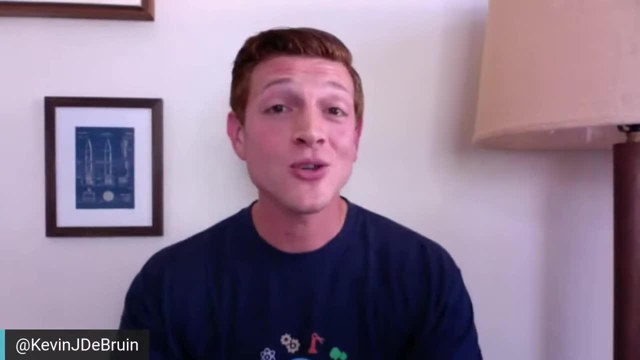 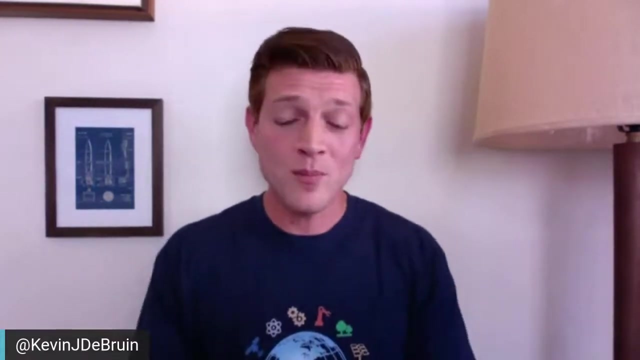 an expert in model-based systems engineering as well. So, yeah, I guess that would be it. Mostly, Python would be the number one, but I've actually also had to work with something called Fortran. You may not have heard of it, It's a very old language, but we build something at NASA and it. 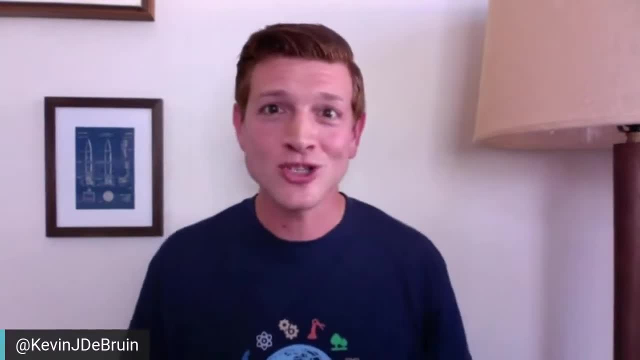 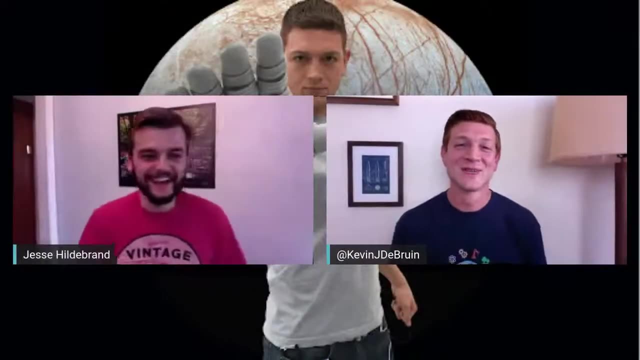 works, So we're going to use it again. So I've had to learn someone's code from 60 years ago to apply to my spacecraft today. How cool is that? Awesome. All right, Ms Voltaire's class, you're in. you're delayed, but you can ask a question. Go for it. 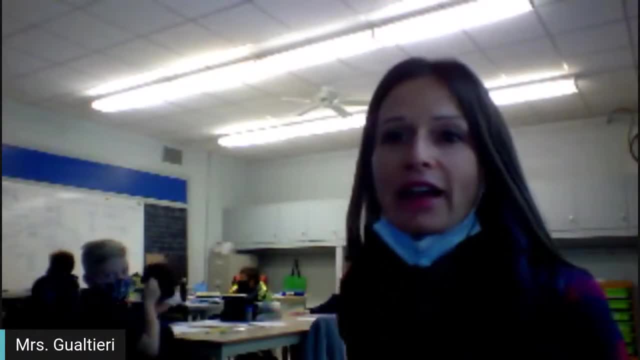 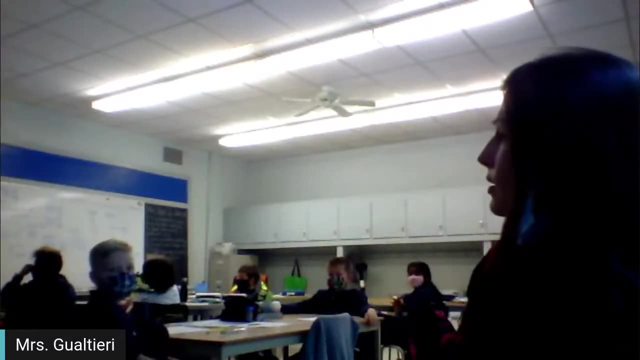 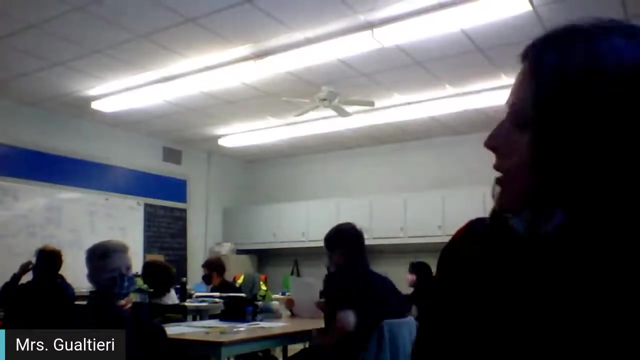 Okay, One of our questions is: how is time different in space? Wow, Is one of our questions different in space? One question, And the other one is: how much does it cost to build the clipper or the clipper? Okay, I'll go with that one first, It's a little bit easier to answer. So how much does it cost it? 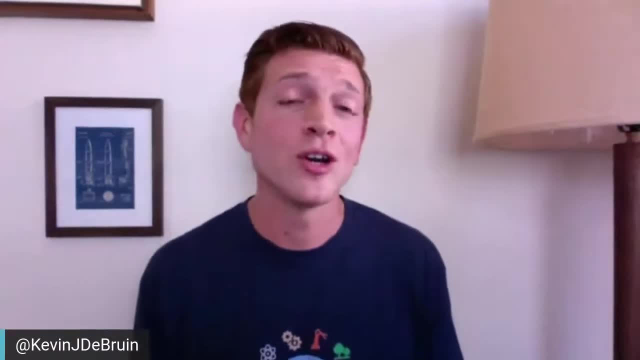 to build the clipper or lander, or I'll even throw in the Mars rover. It's a couple billion dollars, is what we're looking at? Somewhere between like one to 4 billion. normally is the range for those really big spacecrafts. You're right, It's a couple billion dollars. The Europa Clipper. it's not completely done yet, but I believe the estimate is somewhere around 2 billion. Now, to throw a crazy number out there, we have the James Webb Space Telescope that's being built right now. That's looking around $10 billion right now. It's been delayed. There's a 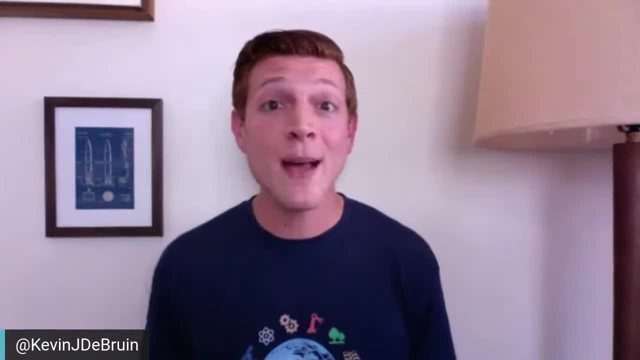 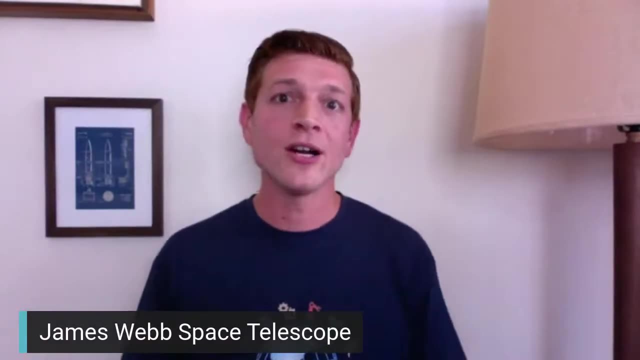 lot more money put into it. So it's a lot of money, And most of that money isn't actually the cost of the pieces. It's to actually pay the hundreds of people that are working together to build the spacecraft. That's the main part of it. 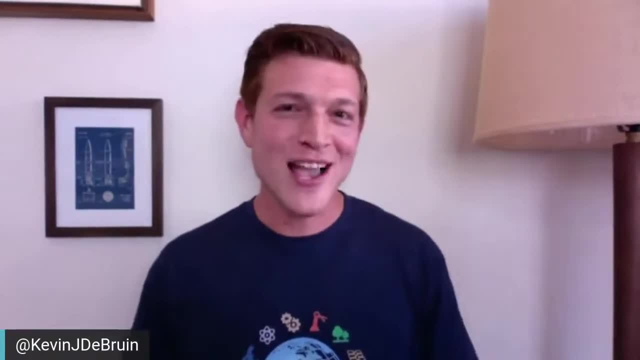 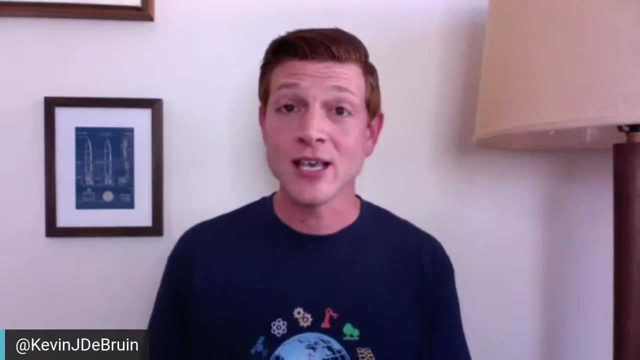 So how is time Time different in space? Now, I'm going to try and keep this very high level so we can understand it. It's called time dilation And, depending on essentially how much gravity you're close to, you can experience time differently than other things. So if we find life somewhere, 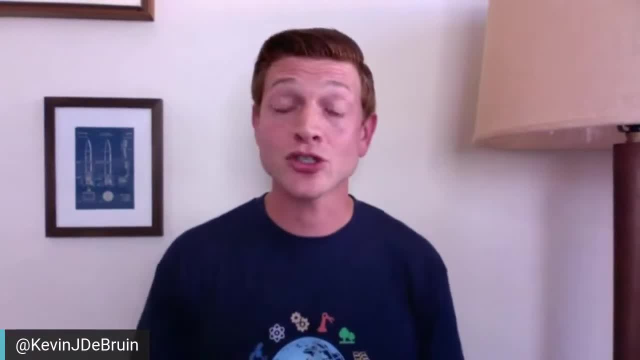 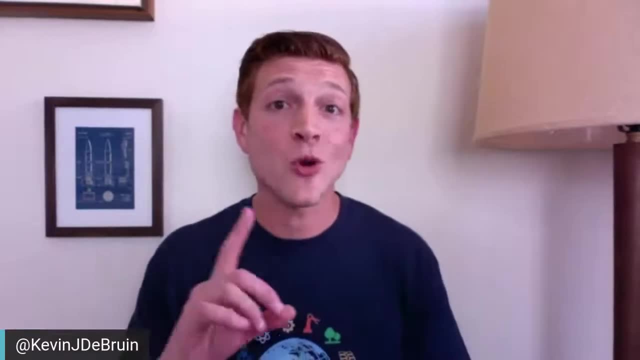 else that has a different sort of gravity. it can experience time slower or faster than us, The astronauts on the International Space Station. that's about 200 miles up, about 400 miles up. That's about 200 kilometers orbiting Earth every 90 minutes are actually a little bit. 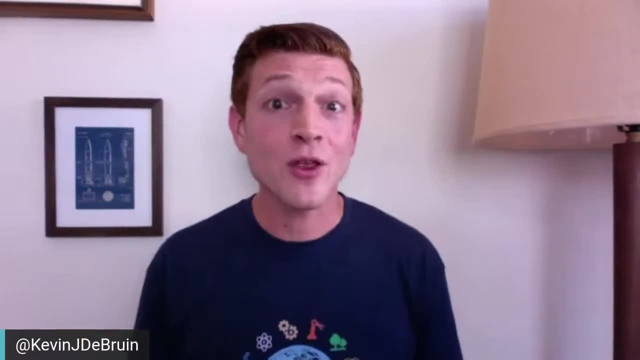 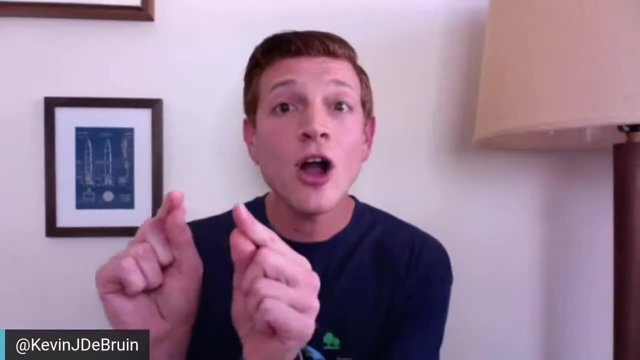 younger than their counterparts down on the surface of Earth because they have less gravity. It's interesting: The ends of their DNA, called telomeres, actually get a little bit longer in space due to the microgravity, the lack of gravity. Now, when they come back down to 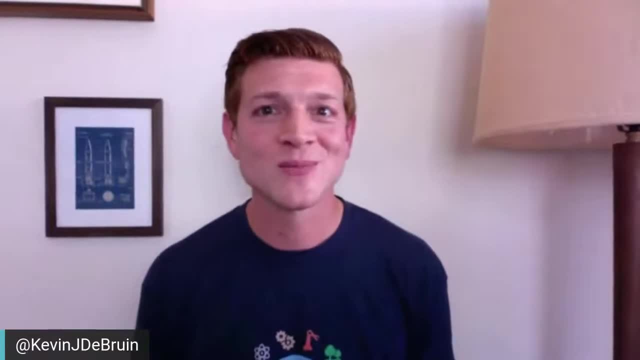 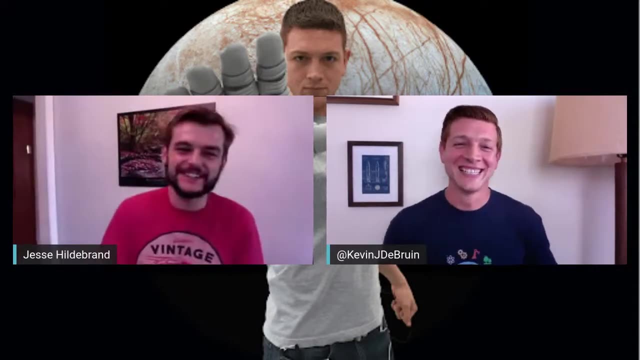 Earth. they shrink back down, but they do get a little bit younger in space. That was a great explanation for a very complicated topic. We can go into some cool special relativity stuff. I don't know what's going on, but great question guys. 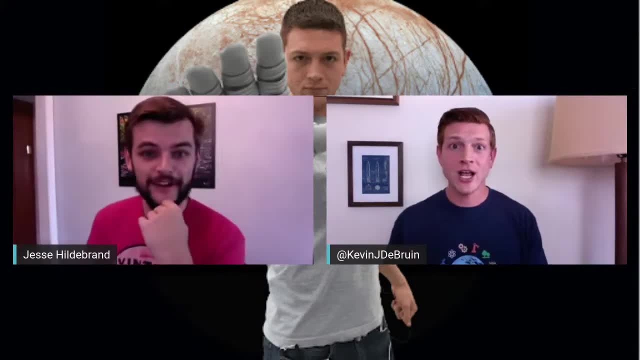 Why don't we get Interstellar to get a good explanation of time dilation? That's a good movie that'll explain the theory of it. Not only will it explain it, but when you're watching the movie it's such an intense score that you will physically age longer. you'll age more than the two and a half hour run time. 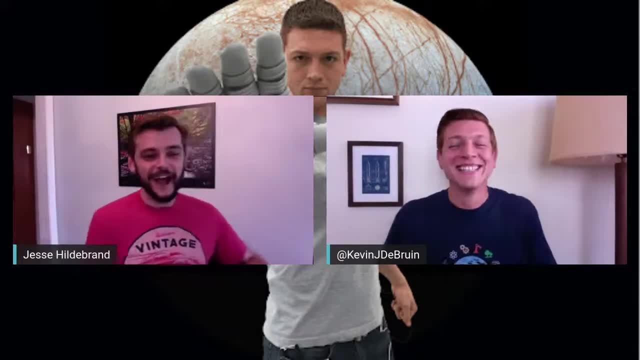 as well. Five years of life go by when you're watching Interstellar. Ms Hamilton again is joining us for the first time. I want to make sure she gets the last question from her classes, and then Kevin will wrap up by highlighting more ways that 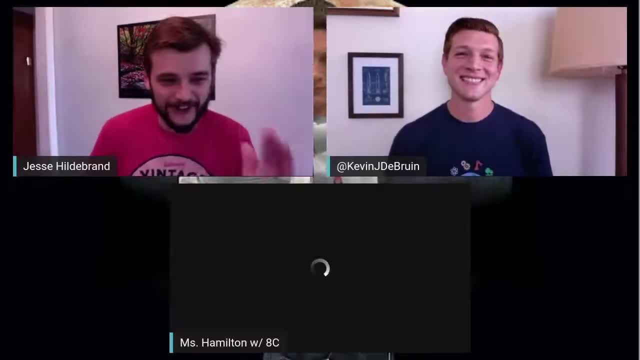 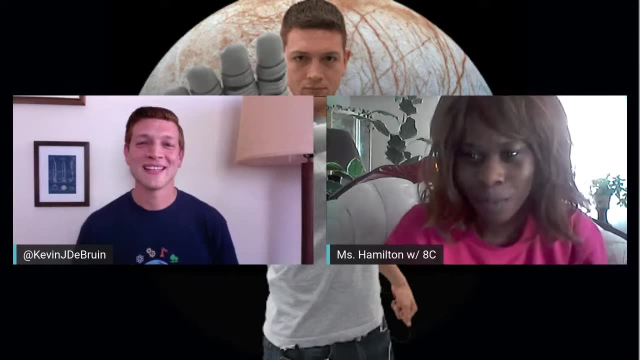 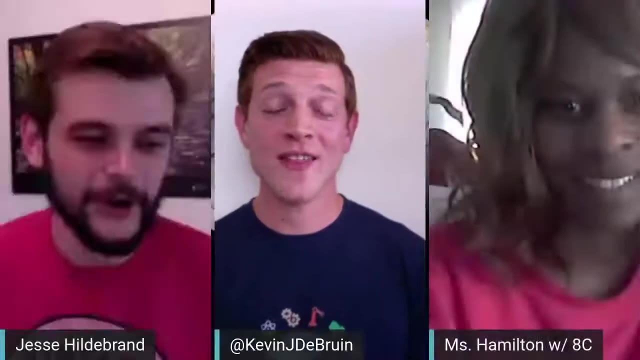 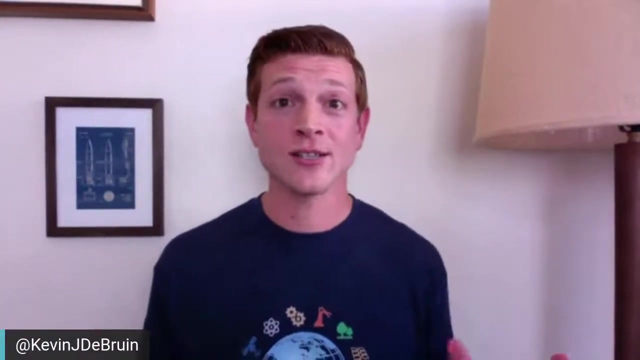 you can do that. We have more than we can possibly answer. so, Ms Hamilton, come on back in and go for it. Thank you for allowing us to have the last question. What is the most important part of designing a spaceship? No pressure on that one. I'm going to go. two of them I'm going to go: soft skills and hard. 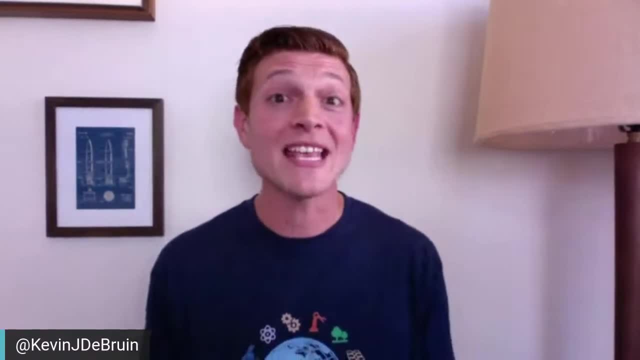 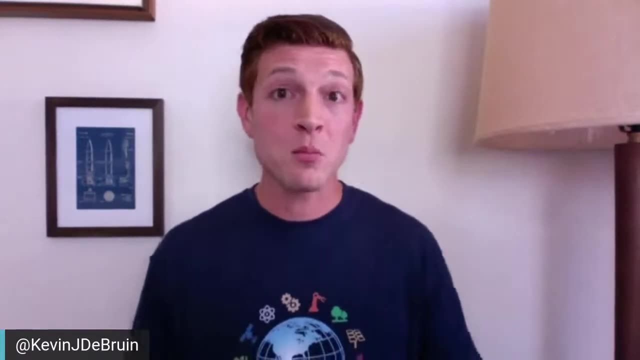 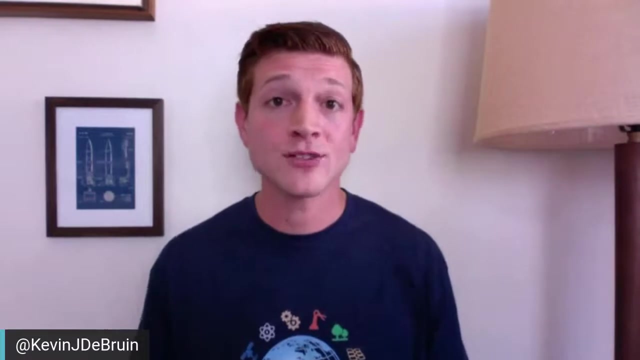 skills. The most important part about designing a spacecraft is teamwork, is being able to communicate with everybody else that is working together, Because we are not building a spacecraft alone. There are hundreds, if not a thousand, people involved in some of our spacecraft, So we need to be able to communicate effectively our concerns, our designs, our. 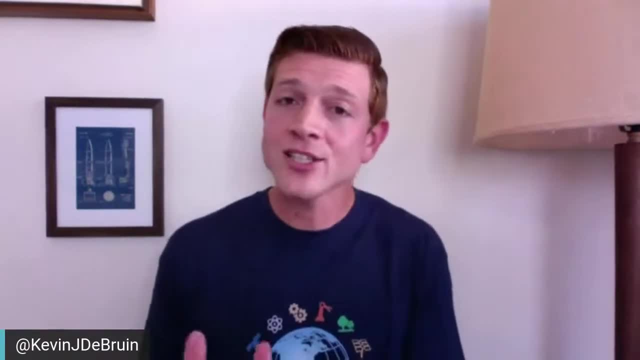 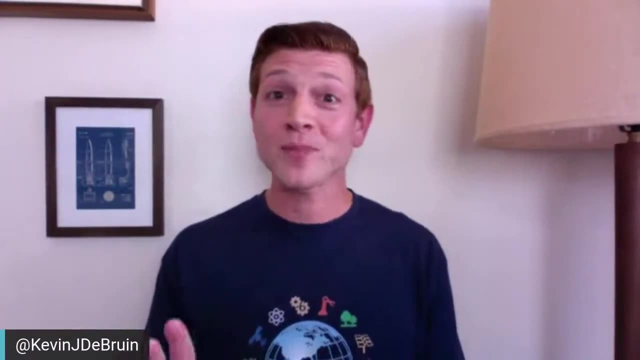 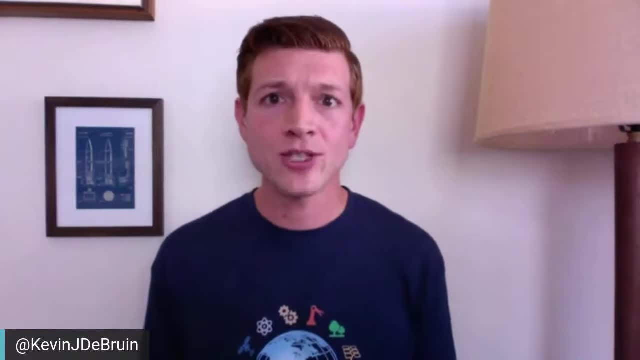 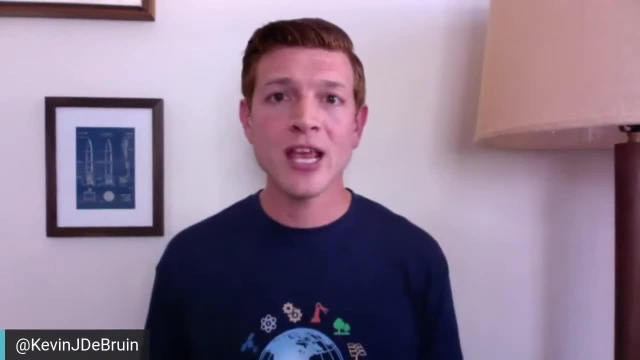 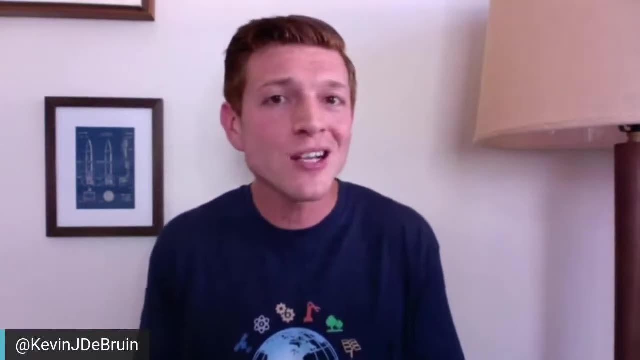 fails, We'll put in two computers And we'll also put in redundancy in terms of computer coding. So we always leave a way so that we're able to change the spacecraft a little bit after it's left the surface of Earth. Because you can't call a tow truck in outer space, We can just call it. 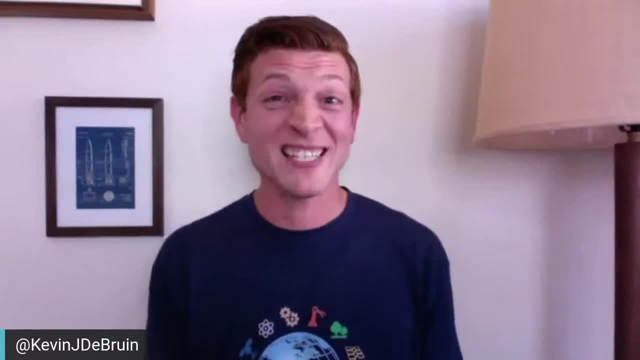 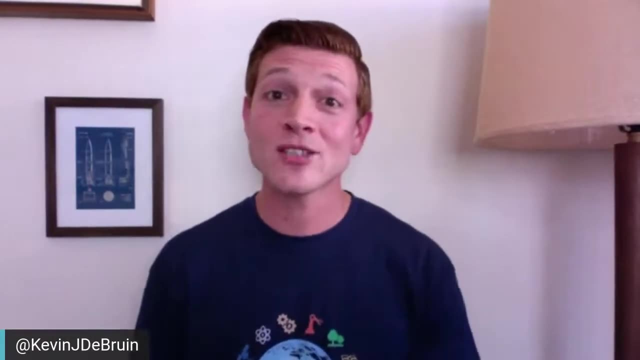 and tell it a few things. So we've got to make sure it works Because, like I said, there are billions of dollars out there in outer space. So being able to communicate effectively with your team, making sure the spacecraft works- Fantastic. 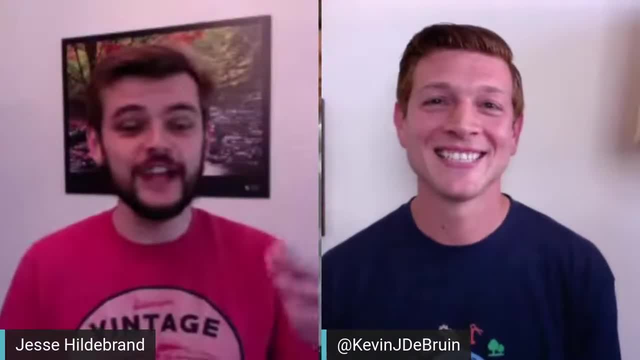 Great question to wrap us up. Thanks, Ms Hamilton, Thanks to all our teachers, And so a bunch of things as we wrap up here. Number one: Kevin's website, on the bottom of your screen in a bar. Check it out. 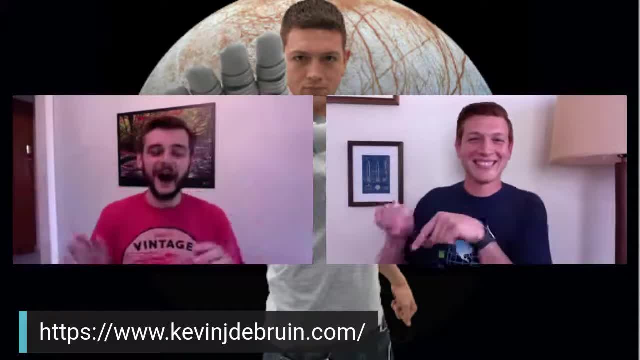 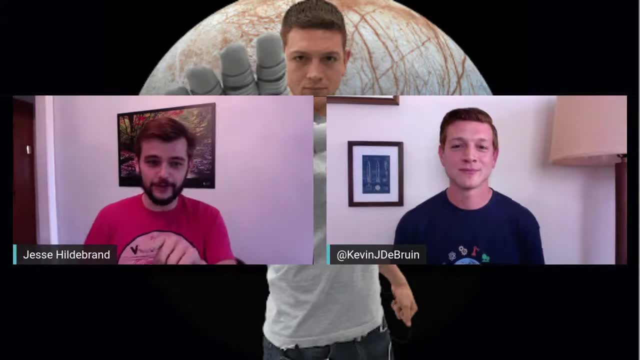 All sorts of really cool stuff- Yeah, there, it's somewhere over there, But yeah, it's amazing- All sorts of great information about him, his books, his work, et cetera. You can check out his name right under his picture there. 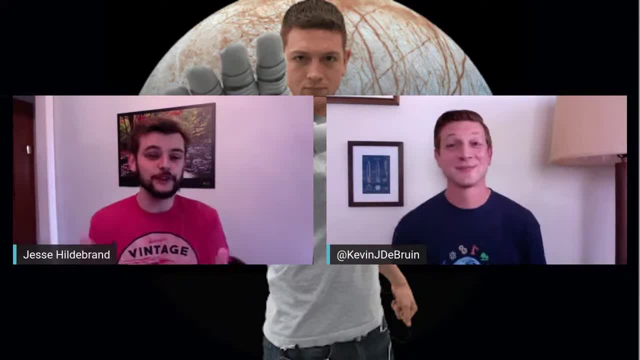 So at Kevin J DeBruin Instagram, ask questions. He's one of the few speakers we have that will literally answer all of your questions. So bug him, harass him to hundreds. by the end of the day, Bring it up. 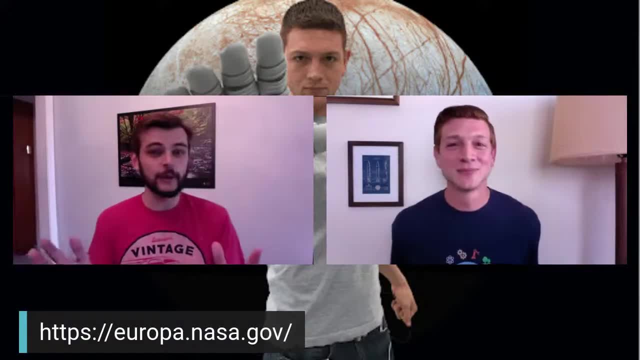 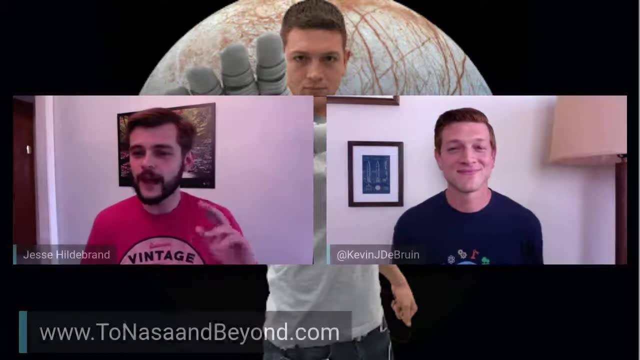 Yeah, let's do it guys. Europa, if you want to learn more about the mission europanasagov- bottom of your screen, It's an amazing program for an amazing moon- Check it out. Learn more To NASA and beyond. Kevin's book. 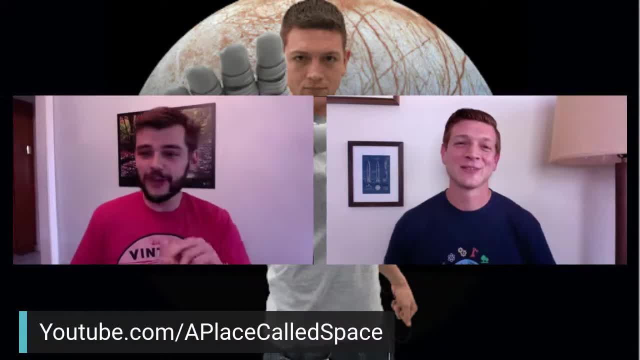 Check that out. And then one thing that I really like actually. first, A Place Called Space, some amazing videos Kevin's been producing over the last few months- Some really really cool stuff. Check it out. It'll keep the learning going. 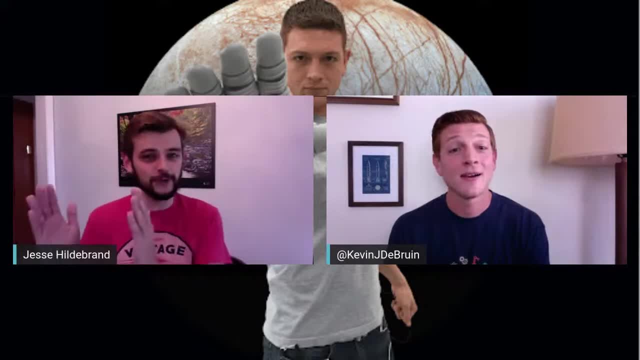 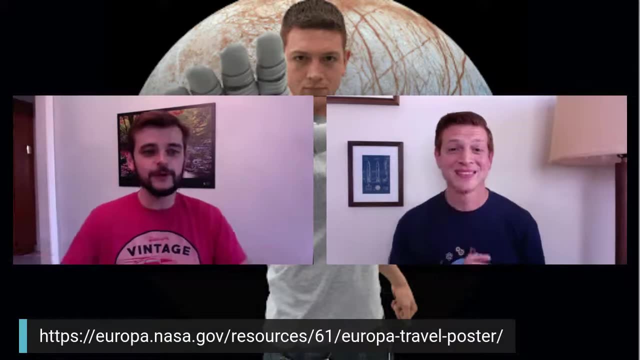 And then, finally, something we didn't get a chance to touch on In Kevin's talk. he showed this really cool travel poster of Europa that NASA produced. NASA allows people to download those, So it's a bit of a long, unwieldy URL. 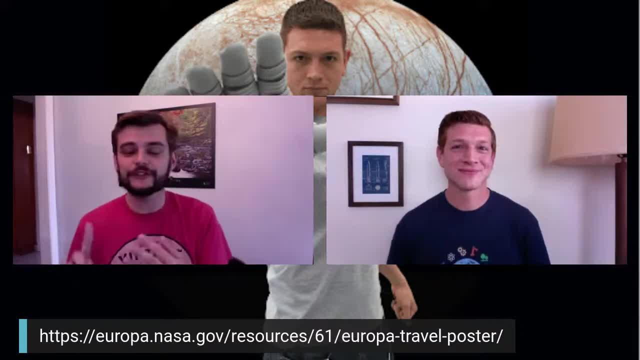 Go to that website. You can check out travel posters for Europa, for Titan, for other moons and planets, for the solar system. Really cool campaign, Really cool book. Print them off, Put them in your classroom and send us a picture of you doing that if you're keen. 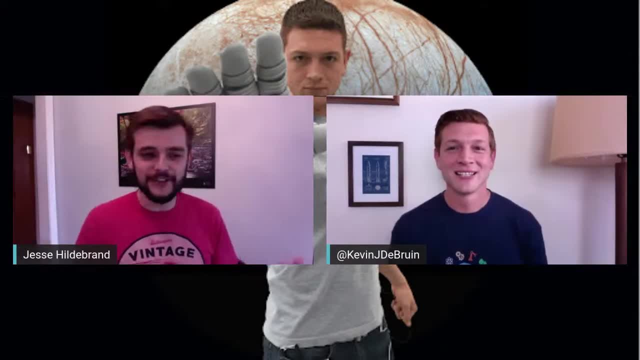 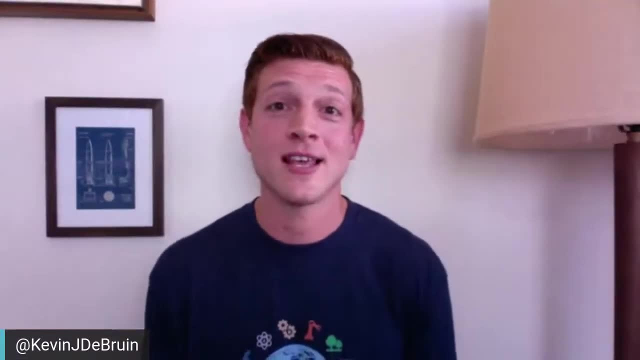 Kevin, is there any last message You'd like to share before we wrap up? It's been such a fun talk today. What are we going to end with? It's been amazing. I will leave with two little phrases that I live my life by. 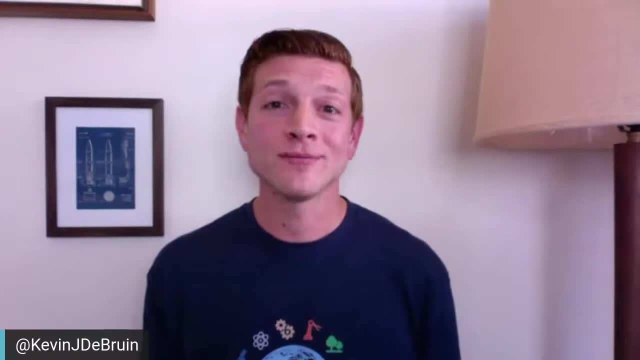 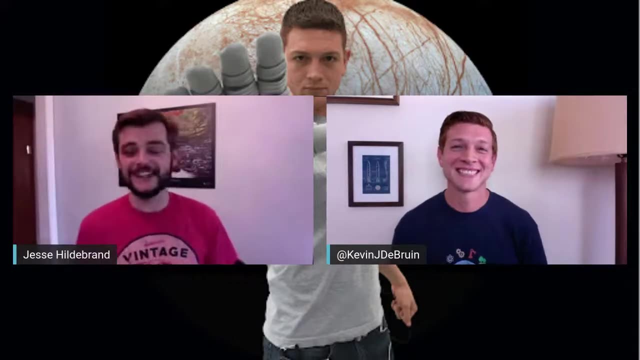 One is never give up And the other one is change the world. Fantastic guys. Well, I'm inspired to change the world. I'm inspired to take some action. I hope you guys are all too, Kevin, as you know what we do at the end of every broadcast. 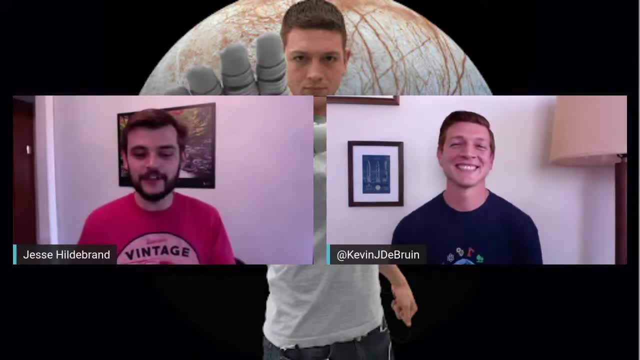 I'm going to bring in every one of our teachers. So, Ms Dubrai, Ms Hamilton, Ms Kump, Ms Hood, Ms Volteri, join me in saying a big thank you and goodbye to Kevin. You're all in. Go for it. 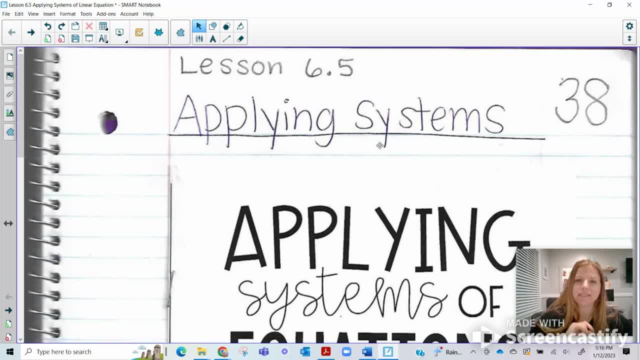 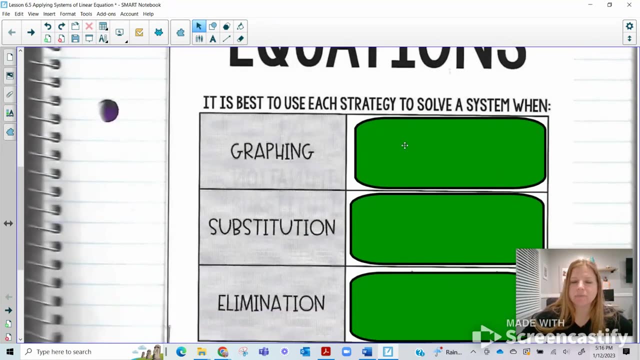 Hey guys, welcome to this lesson where today we're applying systems of equations, which is really just us reviewing. how do we graph and find the solution? how do we use substitution, how do we use elimination? a little mix of everything. So in this booklet that I have here, it says it is best to use each strategy to solve a system when 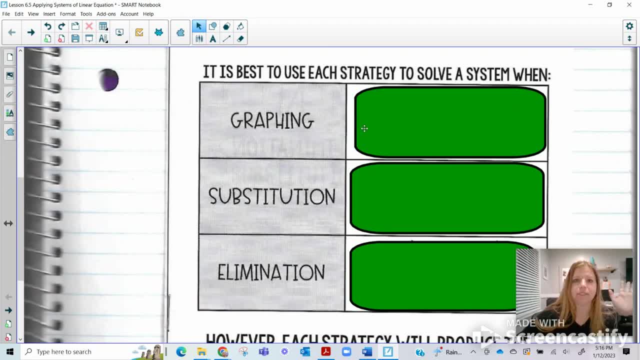 So think about what a system would look like if graphing was like the ultimate thing that you would do, That you would look at that system and say, hey, I'm going to graph this system because it looks like it's set up for graphing.